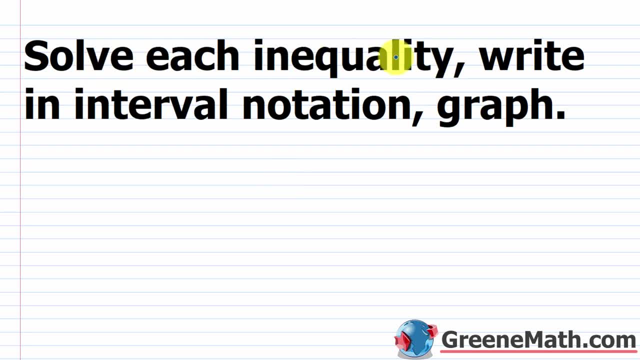 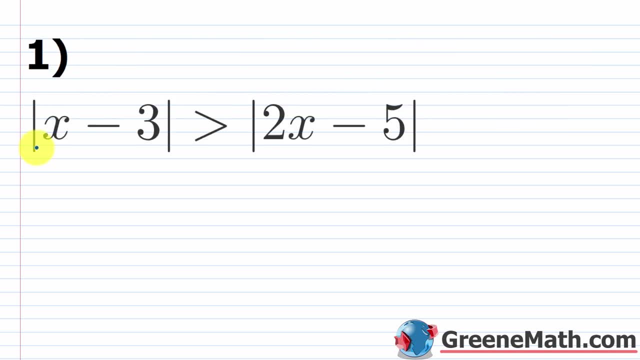 Let's take a look at our practice test. We're told to solve each inequality right in interval notation and graph. We're going to look at problem number one first. So we have the absolute value of x minus three. This is greater than the absolute value of two x minus five. So let's actually take 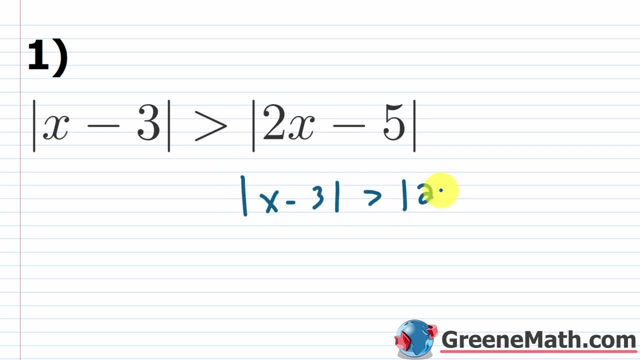 this down to a little table And we'll work on it there And I'll show you how to set this up based on the interval that you're in. Okay, so the first thing is, if you're going to solve this type of inequality, you need to consider a rule for when you're going to drop the absolute value bars. 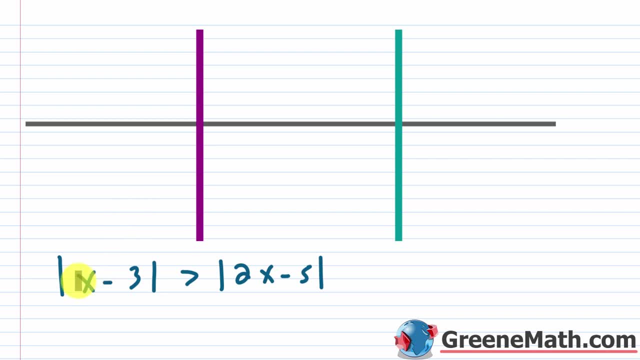 In other words, you would think about: is this guy inside of the absolute value bars that expression? is it negative, Is it zero Or is it positive? If it's negative, then you need the negative of that expression in that interval. If it's zero or positive, you can just drop the. 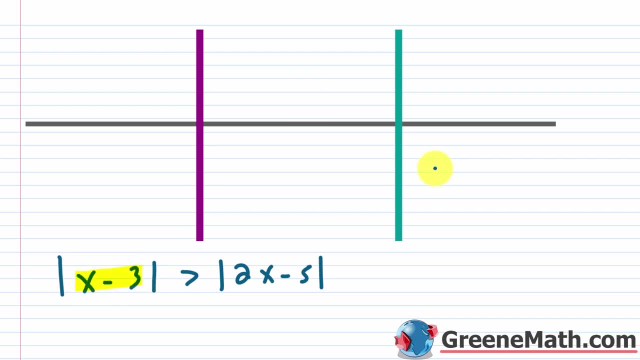 absolute value bars. So you would say: where is this zero? So where is x minus three equal to zero? we would say: is it zero? So we would say: is it zero? So we would say: is it zero? So we would: 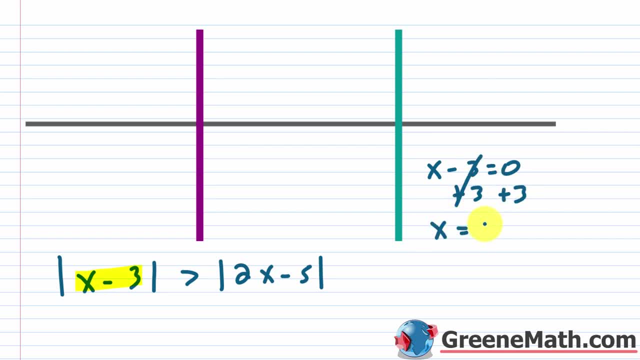 just add three to both sides of the equation, cancel that. you get. x is equal to three, So that's going to be one, what we call breakpoint. Okay, I'm just going to keep this here for right now. I'll fill in the table in a second. We need the other one, So let's look at this one. So this: 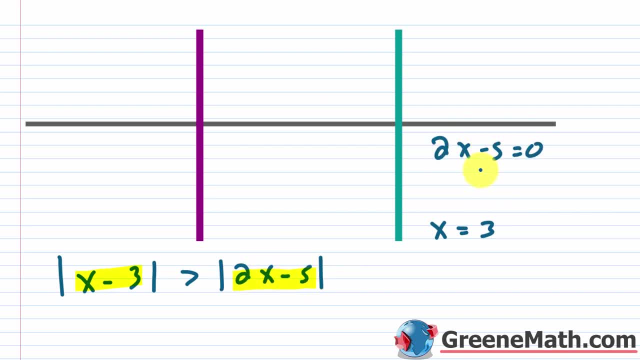 is two x minus five. So let's say two x minus five is equal to zero. we'll add five to both sides of the equation. we'll cancel that. we'll say two x is equal to five. divide both sides by two, So you: 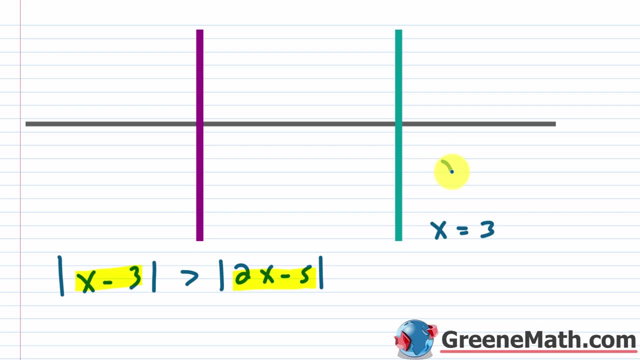 get, x is equal to five halves. Let me just get rid of all this and write this more neatly. So x is equal to five halves. So you're going to use this to solve this type of inequality. So you're going to use these two numbers to set up intervals on the number line. you first think about the. 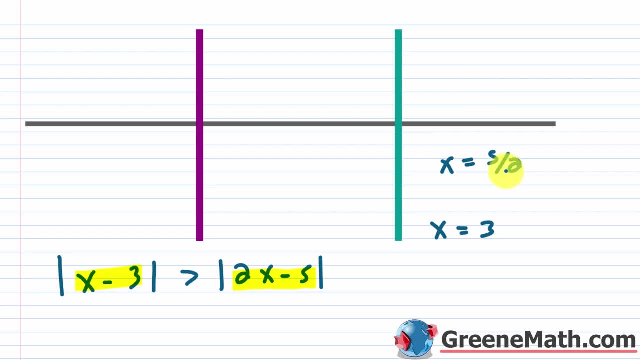 leftmost value. So if I'm on the number line, 2.5 is to the left of three. So what I'm going to do is first have my leftmost interval, I'll say coming from negative infinity, going up to, and. 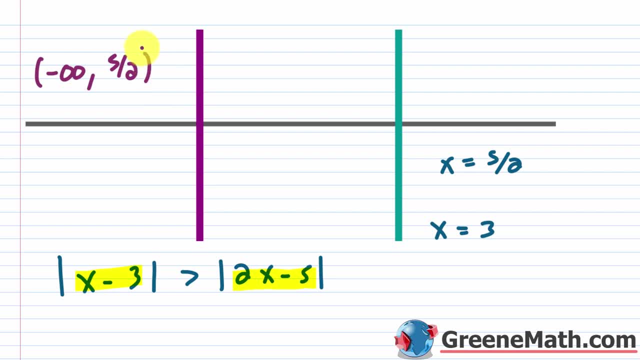 excluding five halves. Now, a lot of people get confused here when you start including or excluding things, So I'm just going to set this up And then I'm going to talk about why. So the next interval, if you look at it's going to be between these two values, So five halves and 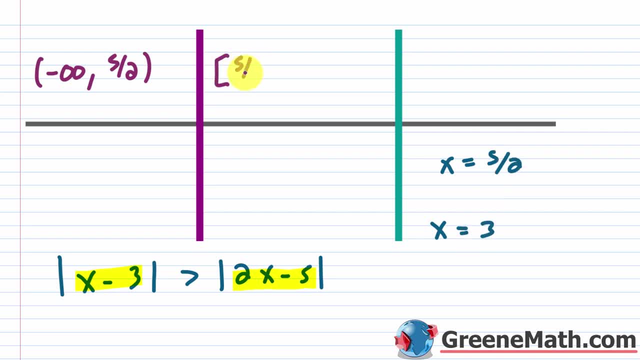 three. So if I'm on the leftmost value, I'm going to use these two numbers to set up intervals on the here And I'm going to exclude three And again. I'll talk more about this in a moment- And then 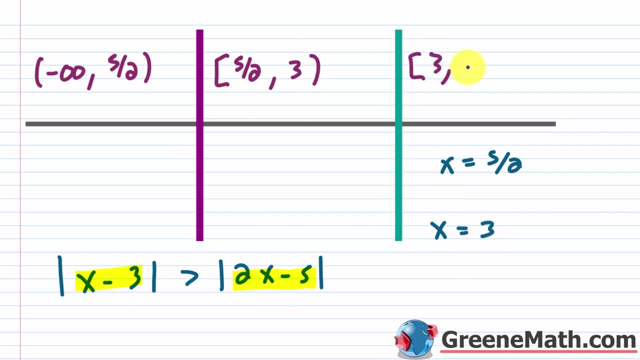 the next interval would be anything that includes three and going out to positive infinity, So basically three or anything greater. So now we've basically split up our number line into three intervals, So anything that's strictly less than five halves, anything that's between five halves. 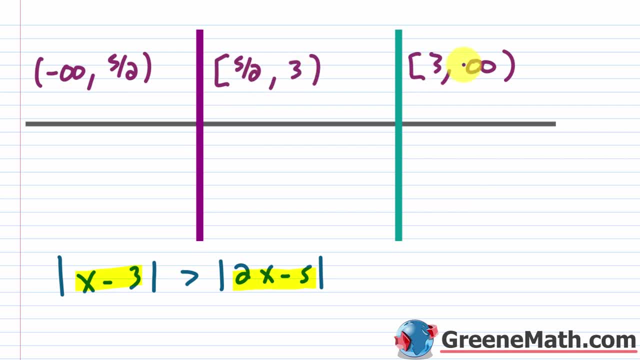 and three, where five halves is included, and then anything that's three or larger. Now what you're going to do is go through and think about, in this interval here, where x is less than five halves, well, each one of these guys is going to be negative. So 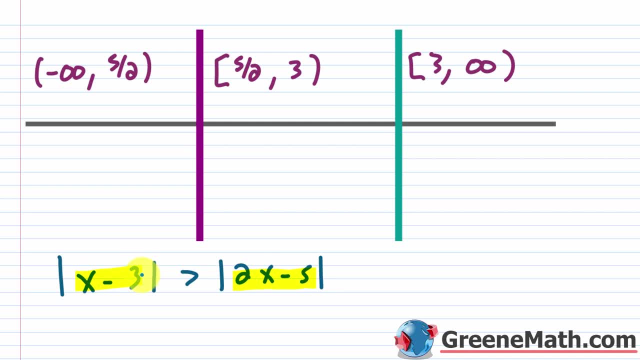 basically, instead of the x minus three here, when I drop the absolute value bars, I want the negative of the quantity x minus three. And then, when I drop the absolute value bars here, I want the negative of the quantity two x minus five. So that's going to be our rule in this interval. 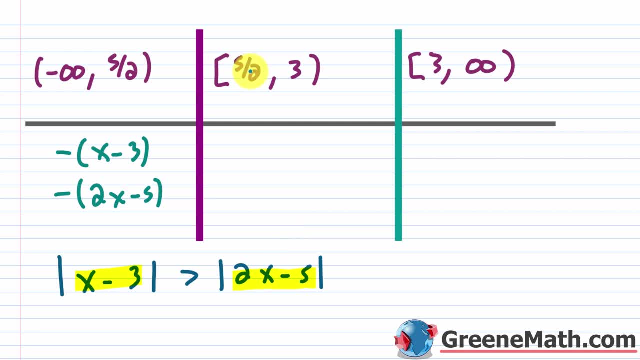 When we get into this interval here, you think about five halves itself. The reason it's included here is because five halves would make this guy, this expression, the negative of the quantity x minus three. So what we're going to do is we're going to take this and we're going to take this. 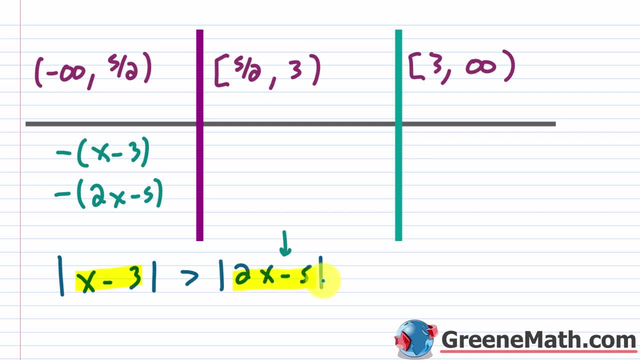 expression zero. So whether it's zero or some positive value, you can just drop the absolute value bars. So this one right here would be two x minus five, And then in this interval it's going to be positive. So it's just two x minus five. Okay, so if it's zero or positive, just drop the. 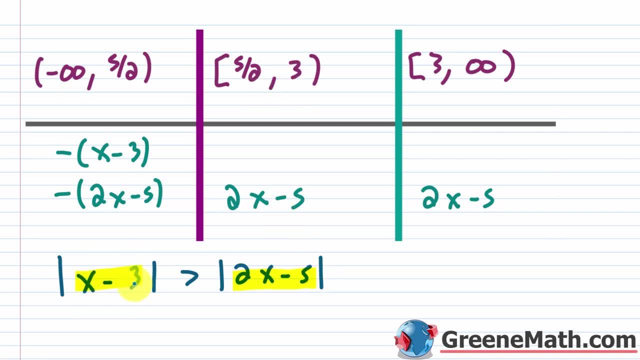 absolute value bars. Now, in this interval, here, this guy is still going to be negative. it's going to be zero when it's three, So that's not till here. So here it's negative, right, Because we're less than three. So we're going to say that this is the negative of this quantity x minus three. 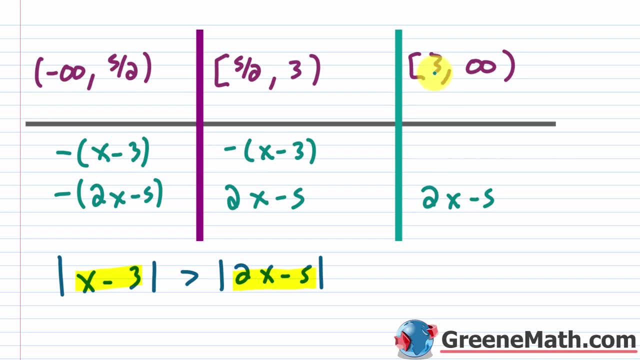 Okay, So in this final interval, again, this guy right here starts at three and includes three. So this guy could be zero or it's anything greater where this guy would be positive. So again, whether it's zero or positive, just drop the absolute value bars. So this is just x minus three, So one thing. 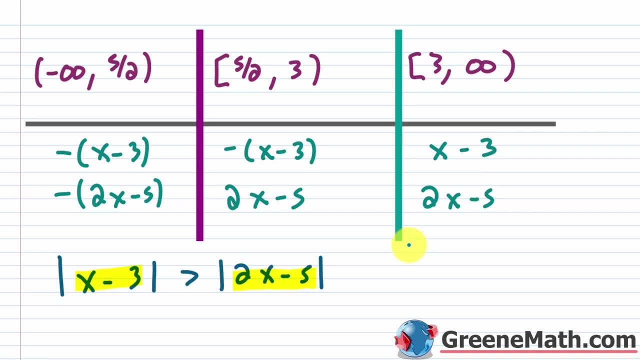 I want to touch on. if you worked on this with me, where we solved equations, you saw that I actually excluded this. So I excluded five halves and I excluded three. Now, I'm not going to do that in this situation, Because when you work with inequalities, you often have this overlap and 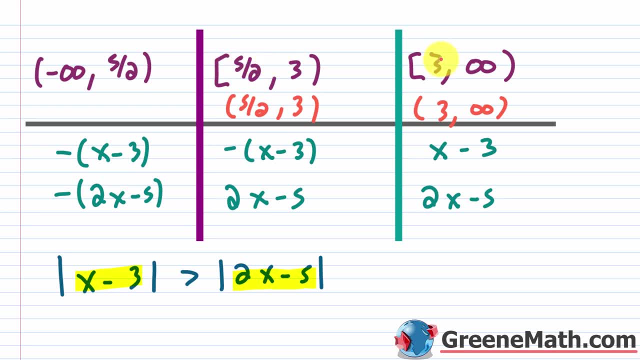 the other way. upbig question here is: is this a negative or positive eruption? You're going to see that in this problem. So I think in this situation this is better, although you could still make it work with this one. I think it's a little bit more challenging to think about it that way. So I'm just 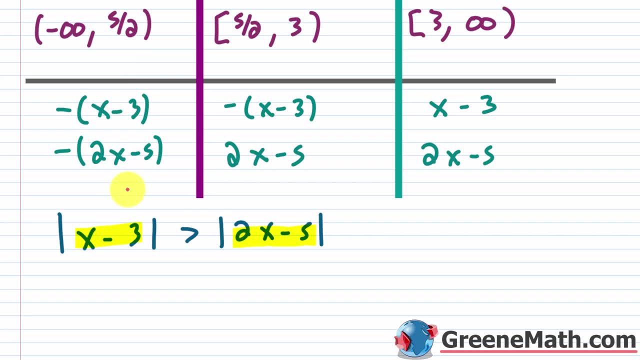 going to just work with it this way. for this type of problem let's start out in the left most interval, or where x is less than five halves. So again, I'm going to basically replace this guy right here with this guy right here. So I want the negative of the quantity x minus three. that's my. 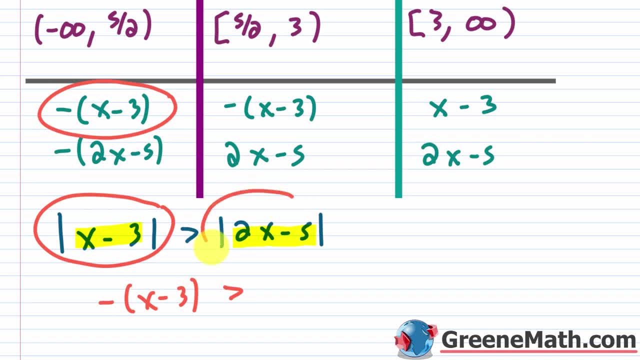 rule for dropping the absolute value bars there, Then this is greater than I want to replace this guy right here with this guy right here. So the negative of the quantity 2x minus 5.. So let's come down here. We'll go back up in a minute. 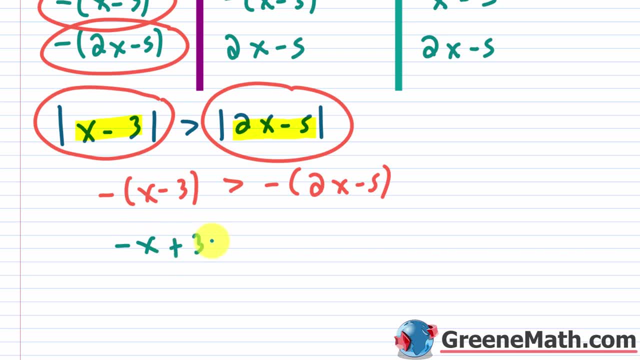 So just distributing the negative, this is negative x and then plus 3.. This is greater than this is negative 2x and this is plus 5.. What I'm going to do first is add 2x to both sides of our inequality here. 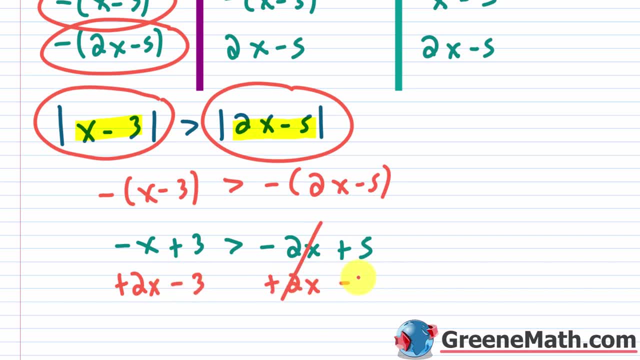 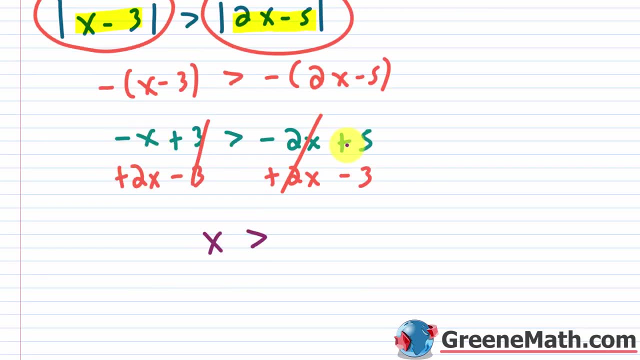 This is going to cancel. And then I'm going to subtract 3 away from each side of the inequality here. This is going to cancel. So negative x plus 2x is going to be x, and this is greater than 5 minus 3 is going to be 2.. 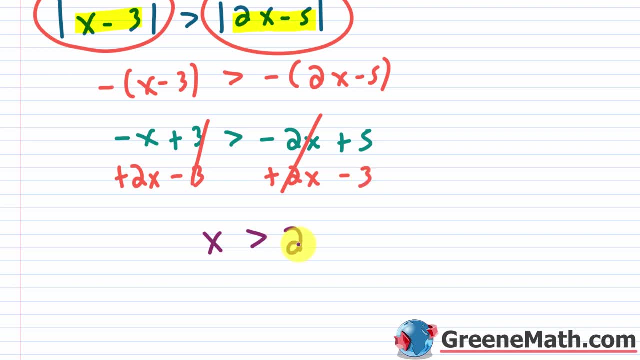 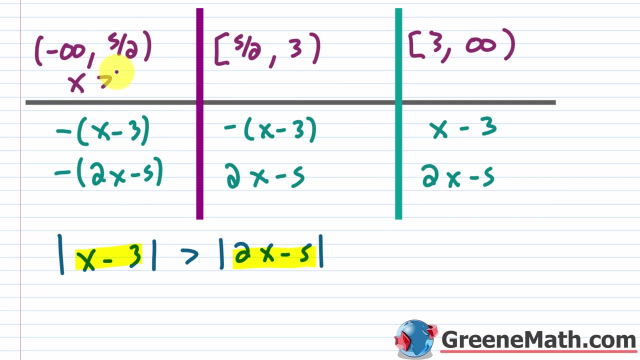 So here we have that x is greater than 2.. So I want to think about that with you. Let's erase everything first. So the way this works, when you get a solution you come into your interval. Let's just write: x is greater than 2 here. 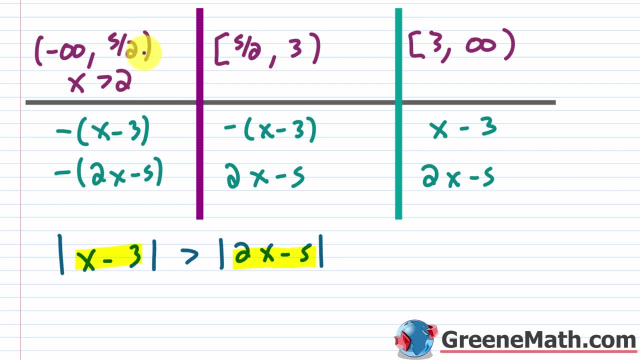 And you would say: is this in this interval? So if I think about 5 halves, that's 2.5.. If I said that x is greater than 2, what I would have here is a partial solution. right, because it has to be in the interval. 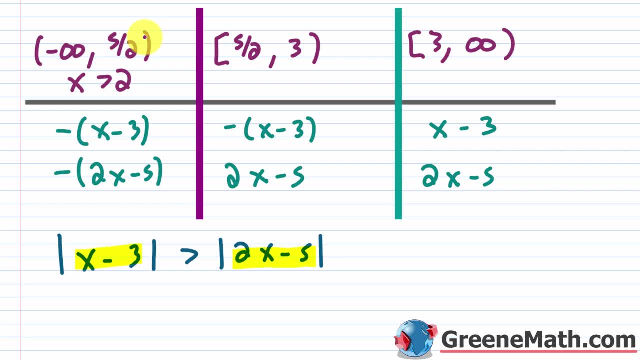 So basically, x would be greater than 2, but it would also have to be less than 5 halves, because you have that cutoff there. So we're going to replace this and say that x is greater than 2 and less than 5 halves, so that we can stay in this interval. 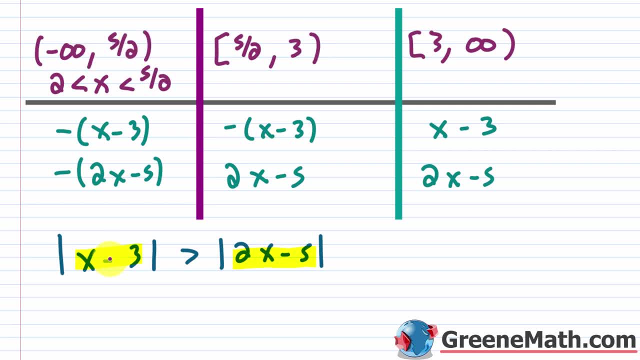 Now I move on to the next interval and I think about what we have here To replace this guy right here. I'm going to use this guy right here. So this is the negative of the quantity x minus 3.. And this is greater than. 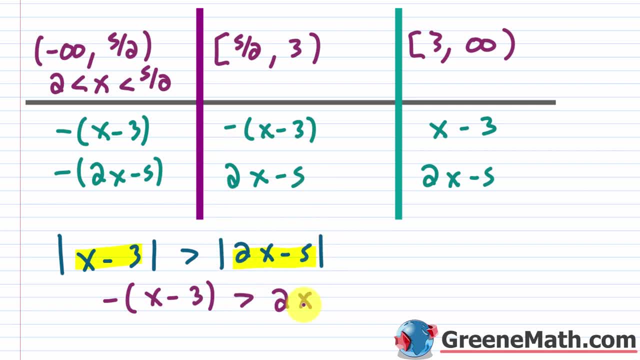 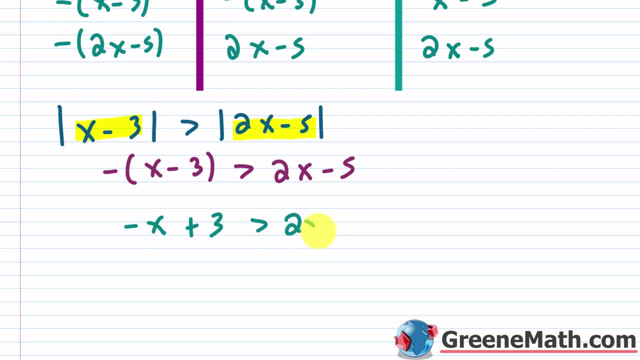 To replace this, I'm going to use this one, So it's just going to be 2x minus 5.. Okay, This right here is going to be negative x and then plus 3. And this is greater than 2x minus 5.. 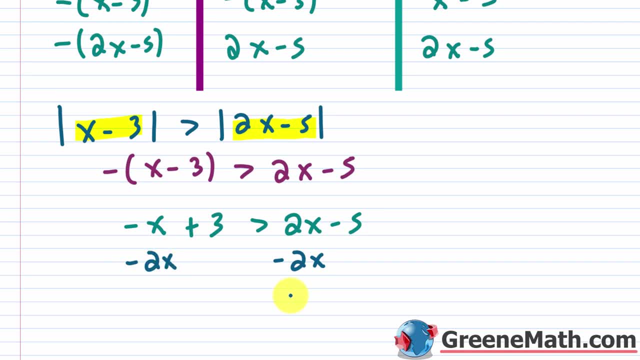 So here I'm going to subtract 2x away from each side of the inequality. This would cancel. Let's subtract 3 away from each side of the inequality. This is going to cancel. So we'll come up here: Negative x minus 2x is going to be negative 3x. 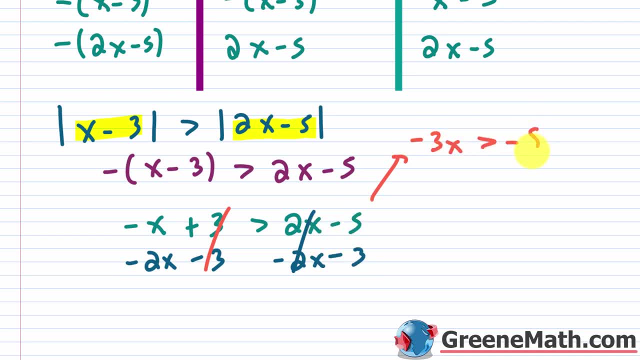 This is greater than Negative. 5 minus 3 is going to be negative 8.. What I'll do from here is divide both sides of the inequality by negative 3.. This will cancel. We'll get x is Remember. this has to get flipped here because we divided by a negative. 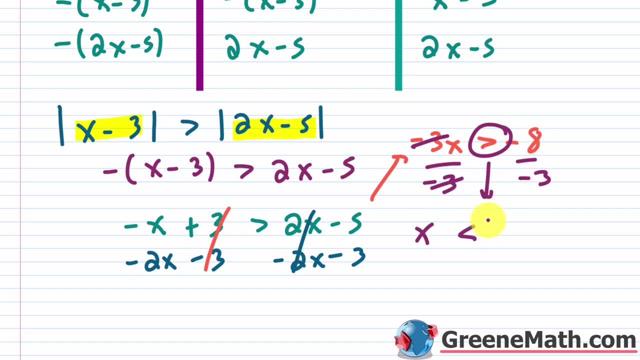 So this is less than Negative over negative is positive. This is going to be 8 thirds. Now, is this in this interval? Well, yes, 8 thirds is going to be 2 and 2 thirds. So that is, if you think about 5 halves, that's 2.5.. 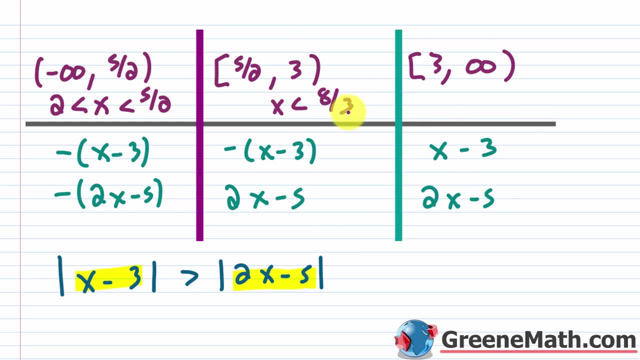 That is a larger value than 2.5.. And it is a smaller value than 3.. So we're good to go there. But what you have to consider again is if you're going down to the left, you have to. 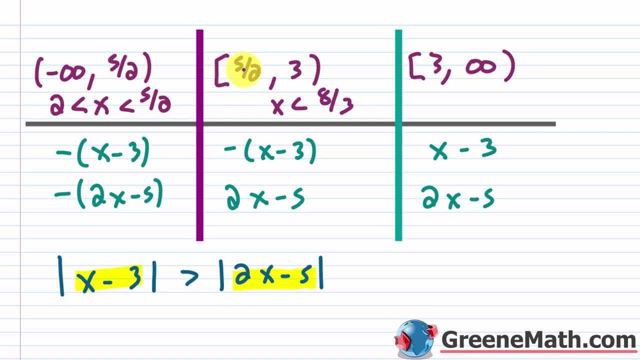 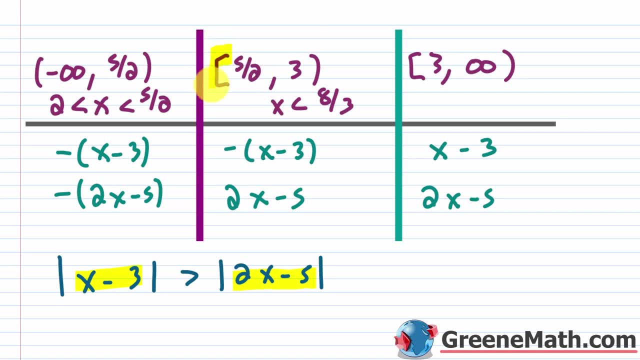 stop at this 5 halves. Now you would include 5 halves here because it's included. So what you would do is you would say that x is greater than or equal to this 5 halves and less than- and this is going to be strictly less than this- 8 thirds. 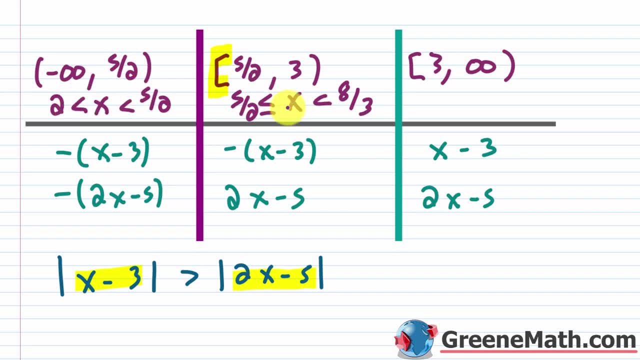 So you can see that we're going to be able to merge these two, and we'll talk more about that in a moment. Now let's work on this last interval here. So here everything is going to be non-negative. So this is 0 or positive. 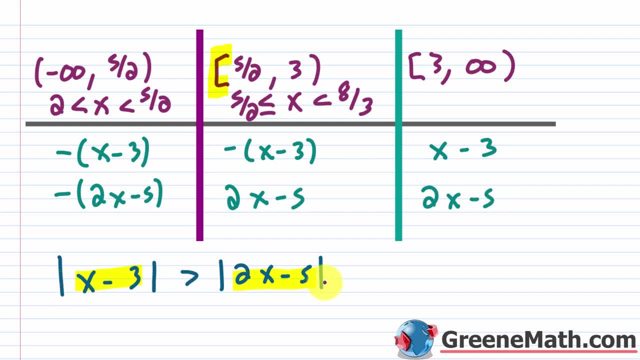 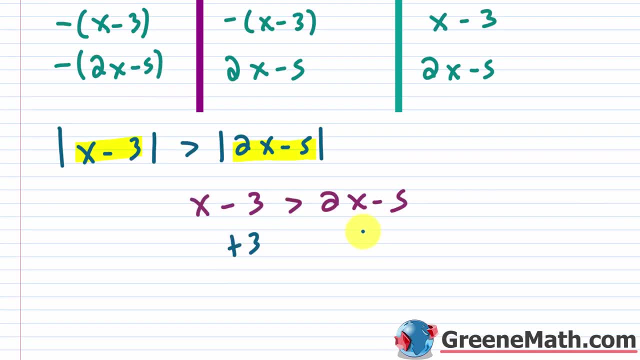 And this guy right here would be positive, right? So I can just drop the absolute value bars and just solve: x minus 3 is greater than 2x minus 5.. So what we'll do is add 3 to both sides of our inequality. 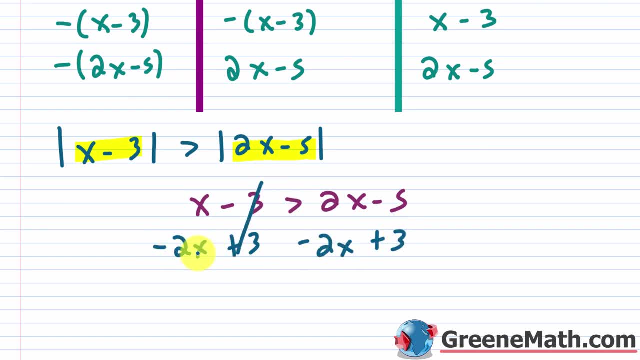 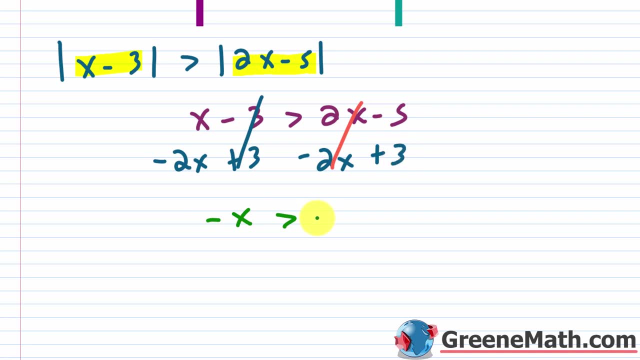 We'll cancel this. We're going to subtract 2x away from each side of the inequality. Let's cancel this. x minus 2x is negative. x- This is greater than negative. 5 plus 3 is negative 2.. Let's divide both sides by negative 1.. 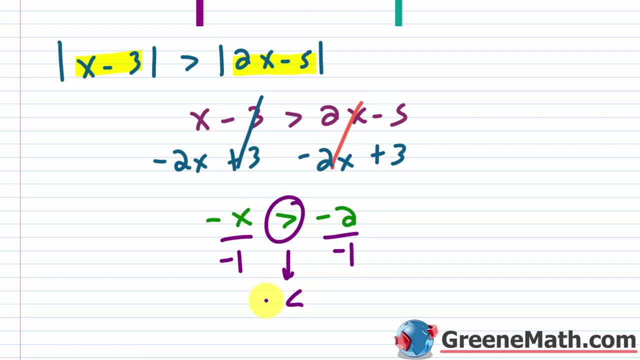 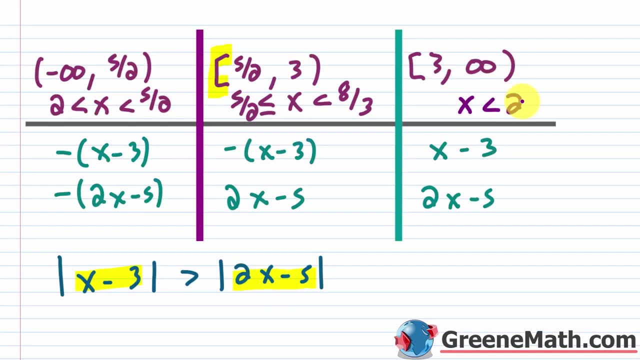 So this is going to get flipped. This is a less than So. here we basically have: x is less than negative, 2 over negative, 1 is 2.. So we have x is less than 2.. Okay, Is this in this interval? 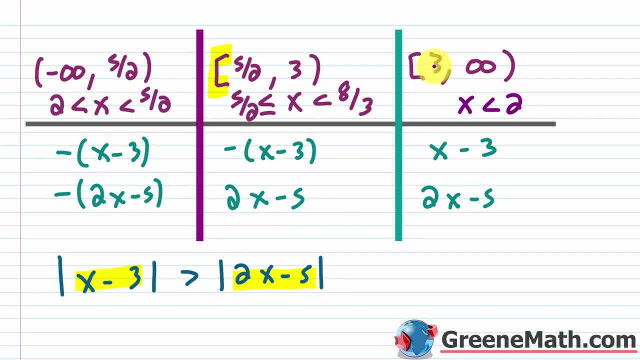 No, This guy has a smallest value of 3,. 3 is included or anything larger, right? This is. x is less than 2.. This is not in this interval. So basically, you just reject that solution, right? You don't even consider it. 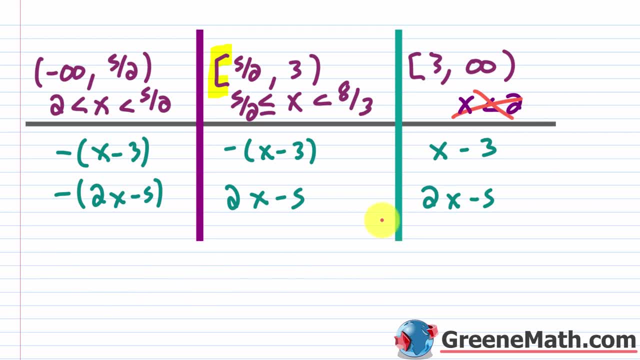 So now what we want to do- I'm actually just going to erase this so I have enough room. You're going to take these two guys and you're basically going to merge them with the keyword. OR You're going to say that x is greater than 2 and less than 5 halves then, OR you're. 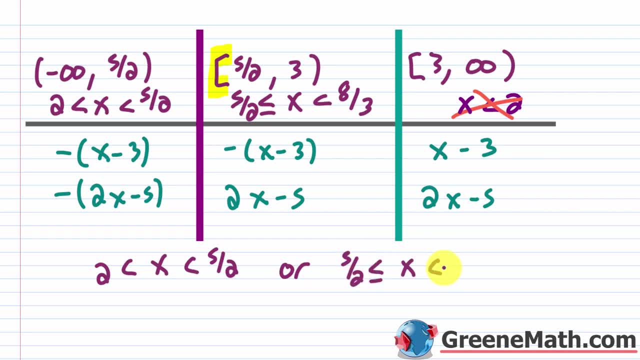 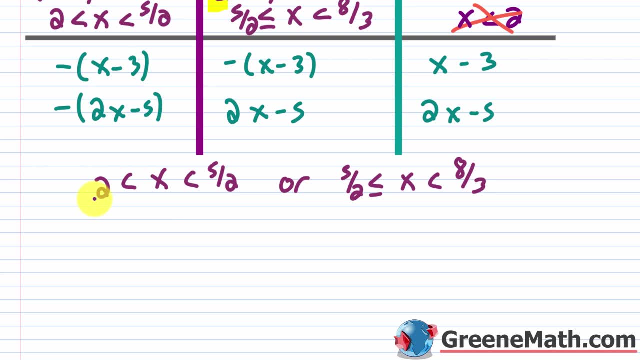 going to say x is greater than or equal to 5 halves and less than 8 thirds. Now, if you think about this, this is basically where x is going to be greater than 2 and less than 8 thirds. which is this 2 and 2 thirds, right? 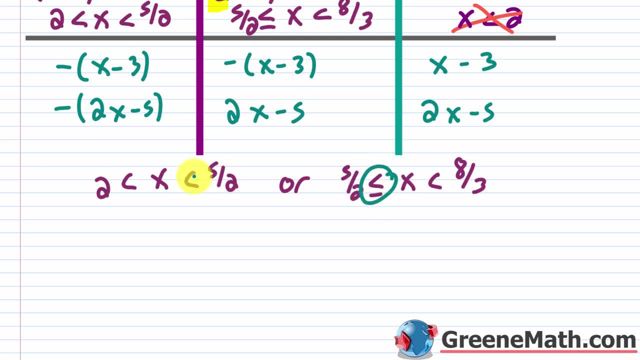 Because the 5 halves is actually included here. okay, even though it's excluded here. So that's how that works. So what I'll do is say that my final answer is: x is greater than 2, and it's going to be less than 8 thirds. 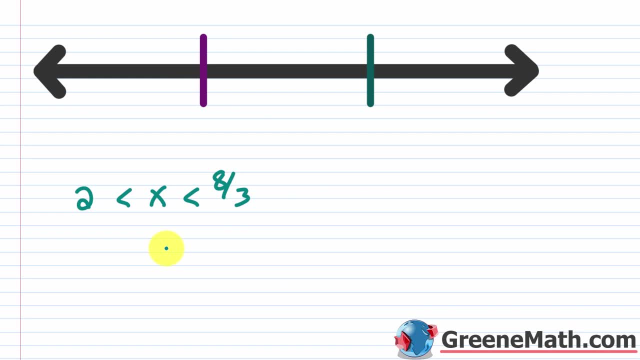 Let's grab this Now. typically, when you solve this type of problem, they're going to ask you to write the solution in interval notation. So let's put a parenthesis next to 2 because it's not included, And let's put a parenthesis next to 8 thirds because it's not included. 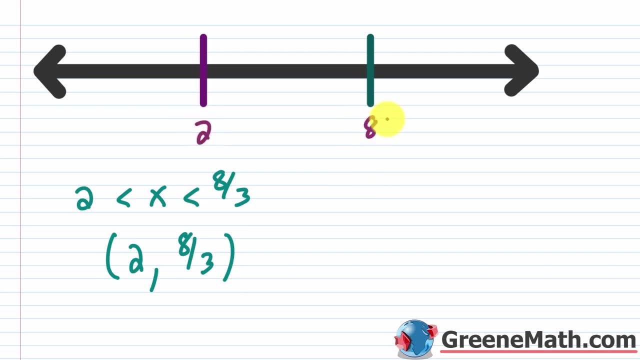 All right now, in terms of graphing this, let's put a 2 here and then 8 thirds here, And then I'm going to use a parenthesis at 2 to show that it's excluded and a parenthesis at 8 thirds to show that it's excluded. 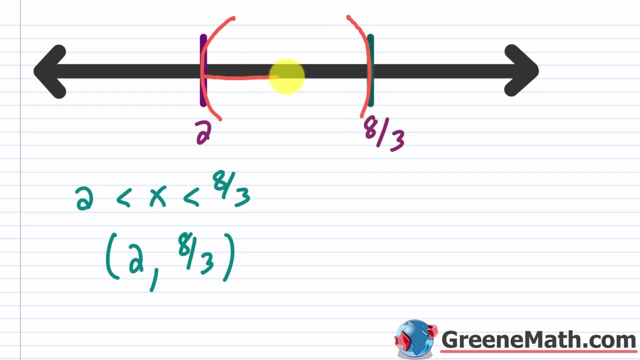 Again, you can always use an open circle. Your book may do that instead, So let's shade this in. So basically, we're showing that x can be anything that's larger than 2, going up to and excluding 8 thirds. 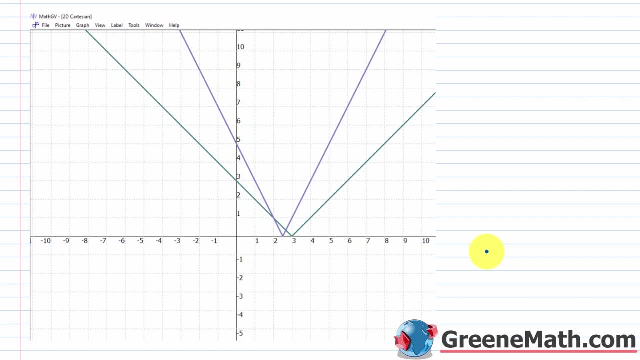 All right. so if you're struggling with this concept, you can always graph this using a free online graphing calculator. I would recommend something like Desmos. I'm using MathGV, which is something that's also free, So let's first think about what we had. 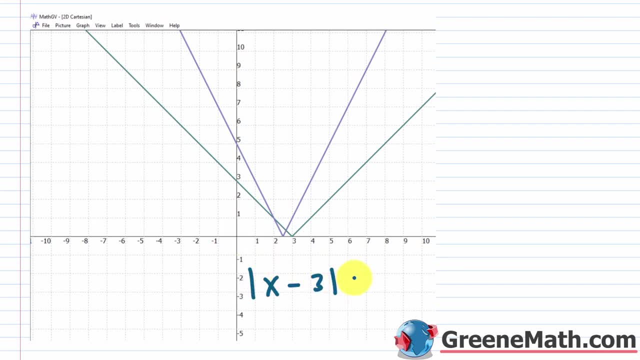 We had the absolute value of x minus 3.. And we said: this is greater than the absolute value of 2x minus 5.. Now, we haven't talked too much about graphing in this course yet, but hopefully you remember some of this stuff from Algebra 1.. 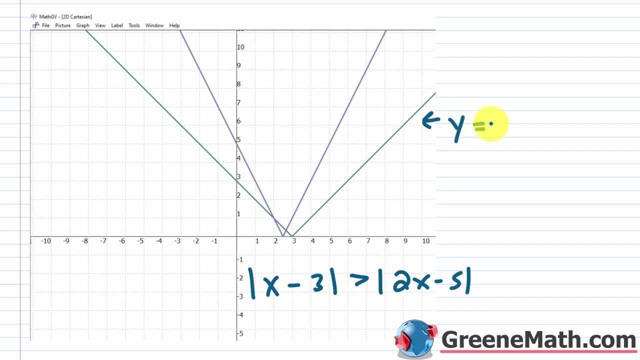 Essentially, this guy in green- this is y- is equal to the absolute value of x minus 3.. This guy in purple- this is going to be y- is equal to the absolute value of 2x minus 5.. So you're just looking at the graph of each and you're saying, hey, where is this green? 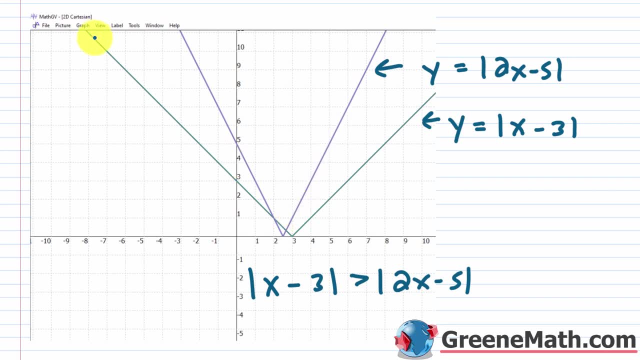 graph above. Okay, Where is this purple graph Right? So you can see here it's below below, below, below, below, below below, And you'll see that at 2, they're going to intersect And they're also going to intersect. 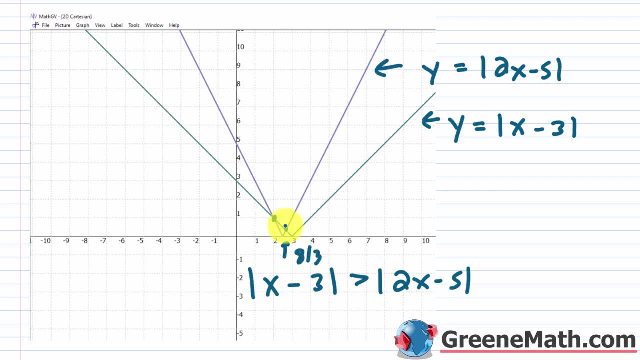 This is going to be that 8 thirds that we talked about, or the 2 and 2 thirds, And then everywhere outside of that it's going to be below. So you can see that this piece right here, between this 2 and 8 thirds, it's actually 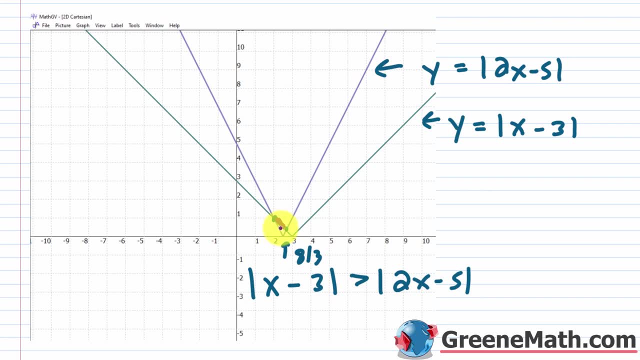 going to be above the purple graph where it has a higher y value or function value for those given x values. So that is true: Where x is greater than x, It's less than 2. And less than 8 thirds. Again, at 2 and 8 thirds they're equal. 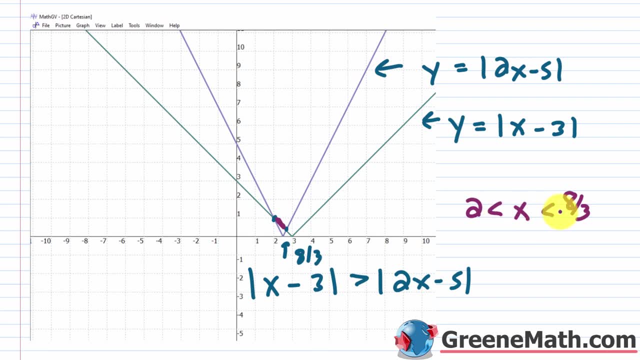 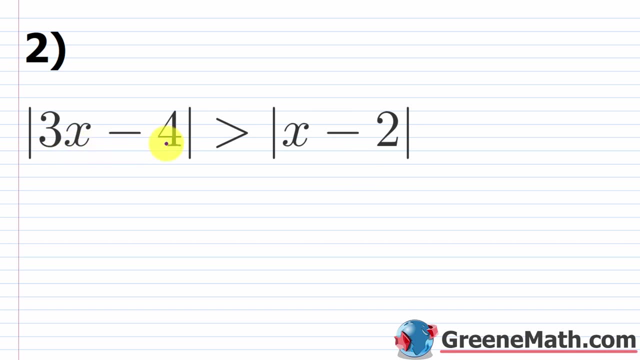 So this is a strict inequality, So you have to use strict inequalities here. So that's how you could get your solution graphically. All right, Let's take a look at problem number 2 now. So we have: the absolute value of 3x minus 4 is greater than the absolute value of x. 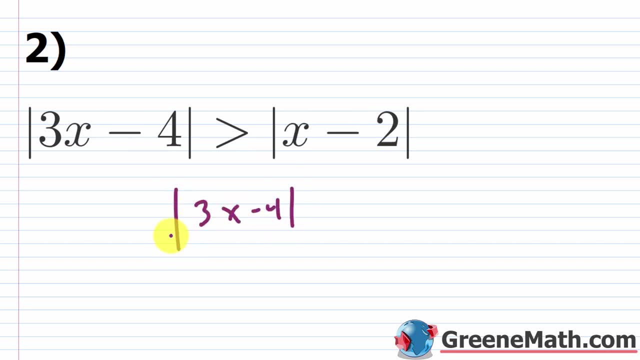 minus 2.. So let's just write that really quickly. So again, the absolute value of 3x minus 4 is greater than the absolute value of x minus 2.. Okay, So once again I'm going to work on a table. 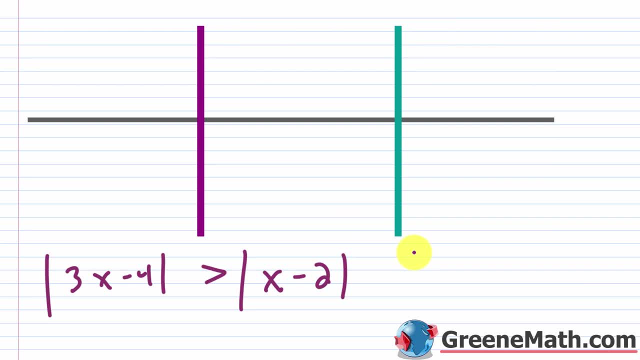 If you want to use a number line, that's fine. Okay, So let's split this into different intervals. Now we get the intervals from again thinking about what's inside of the absolute value bars. You're going to set that equal to 0.. 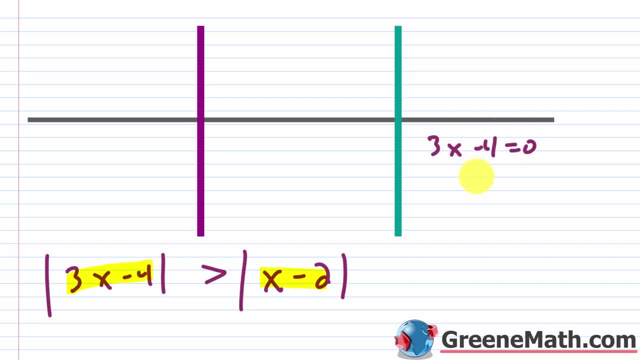 So for example here: 3x minus 4, if I set that equal to 0, we add 4 to both sides. Cancel this. You get 3x is equal to 4.. Divide both sides by 3.. 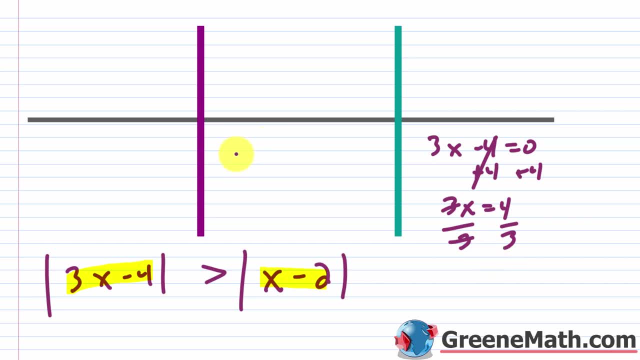 We'll cancel that. So x is 4 thirds. So let me just put x equals 4 thirds And this is just scratch work. I'm going to erase that in a moment. The other guy is this: x minus 2.. So x minus 2 equals 4.. 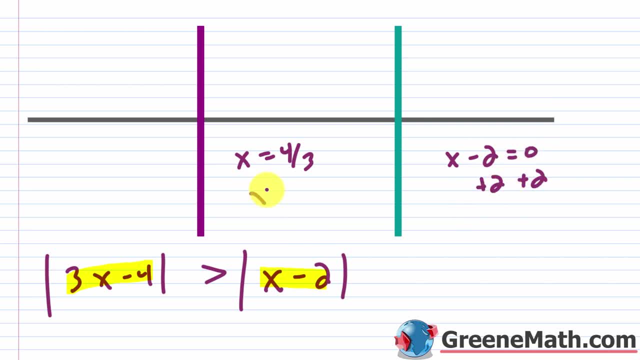 Okay. Okay. So x minus 2 equals 0. Add 2 to both sides And you get x is equal to 2.. So you're using these two numbers here to split the number line up into three intervals. Okay, So you think about the leftmost value. 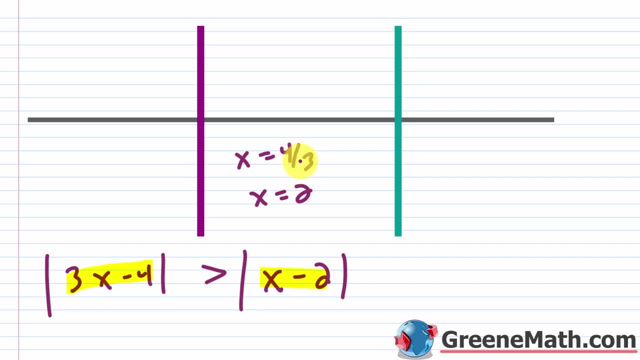 The leftmost value here is 4 thirds. right It's 1 to the third. That's less than 2.. So you're going to create this interval here, coming from negative infinity and going up 2 and excluding this value, So excluding 4 thirds. 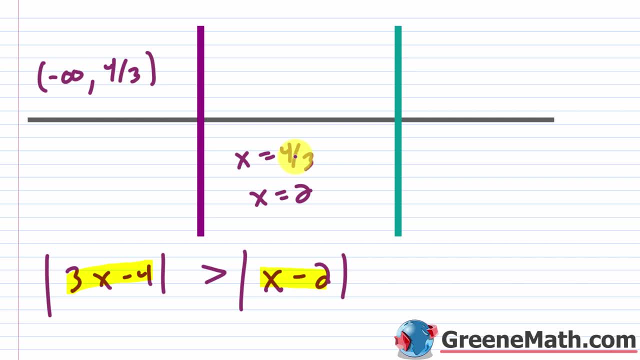 You want something where both of these are going to be negative. You don't want to include 4 thirds, because there this would make this 0. Okay, So they both have to be negative in this first guy, Then here this is going to be between these two values, but I'm going to include 4 thirds. 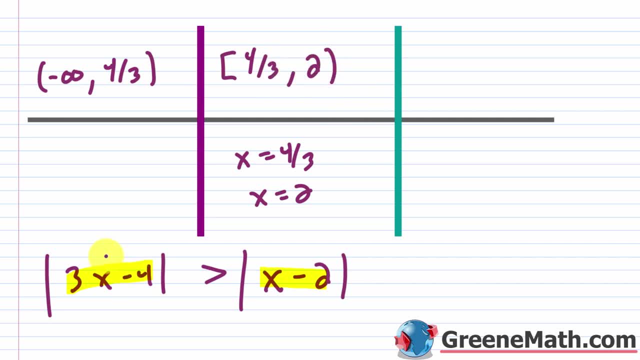 and I'm going to exclude 2.. And the reason I'm doing that is if I include 4 thirds for this one it's 0, and that's okay, Because if this guy is 0 or some positive value, it's the same rule. 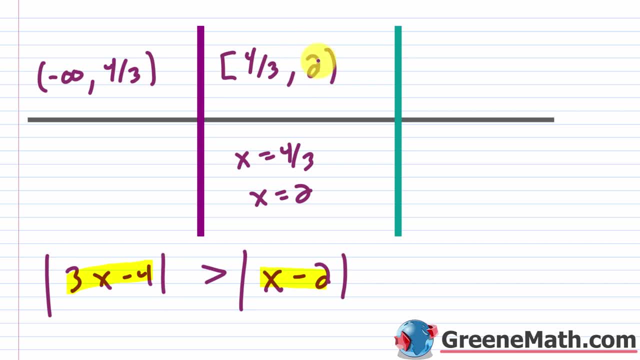 I can just drop the absolute value bars, But I don't want to include 2 here, because if I did well, then here at 2, this is 0. It's a different rule than if it was negative or less than 2.. 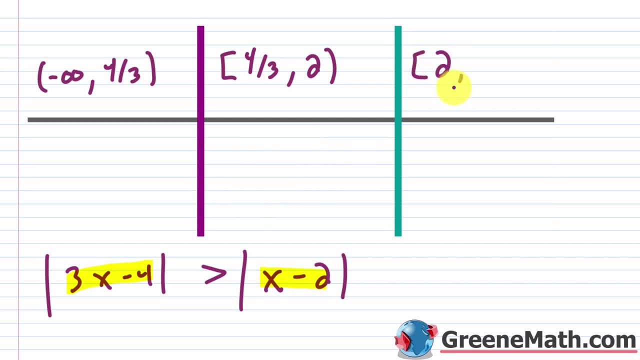 Okay, So this interval would include 2 and go out to positive infinity. Okay, So we've split the number line up into these three intervals. So what we are basically doing is just getting a rule for dropping the absolute value bars in each interval. 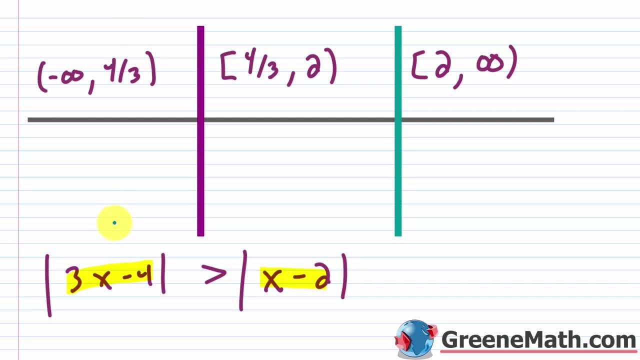 So in the leftmost interval, where we're strictly less than 4 thirds, this expression is negative and this expression is negative. We know that. So basically, you replace this guy right here with the negative of the quantity 3x minus 4.. 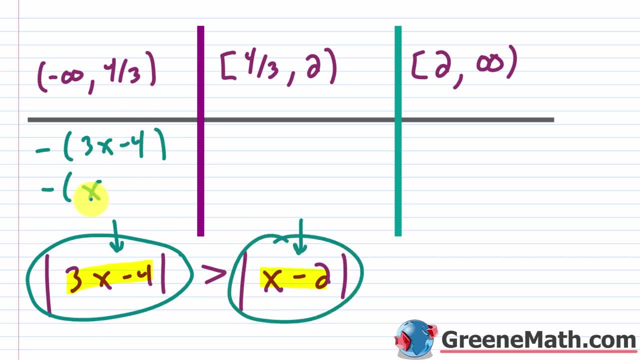 Okay, So this guy right here with the negative of the quantity x minus 2.. Now when we move to the right in this next interval, 4 thirds is included. So that makes this guy 0 here. And then we're going up to, but excluding 2.. 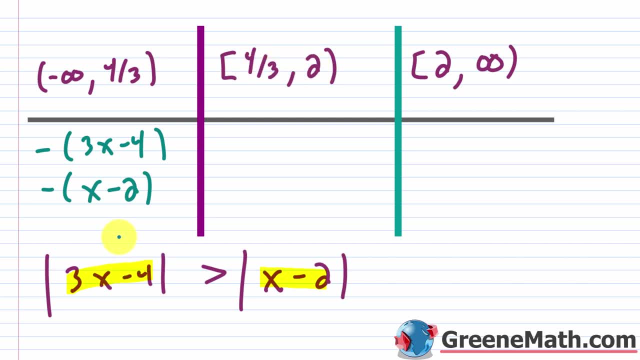 So between 4 thirds and including 4 thirds and 2, this guy is either 0 or positive, And whether it's 0 or positive, you just drop the absolute value bars, So it's just 3x minus 4.. 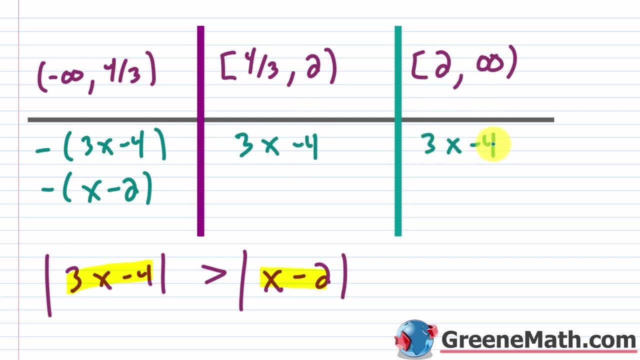 Then when we get to 2 or larger, it's going to be positive, Right? So it's 3x minus 4 here as well, Okay. So if we think about this x minus 2 here, this is negative in this interval. 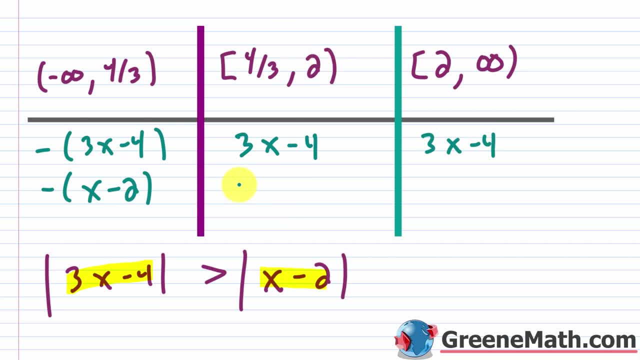 Okay, And that's because we're less than 2.. That's why we didn't include it here. So this is the negative of the quantity x minus 2.. And then here, because we're including 2, it can be 0 or anything larger where it would. 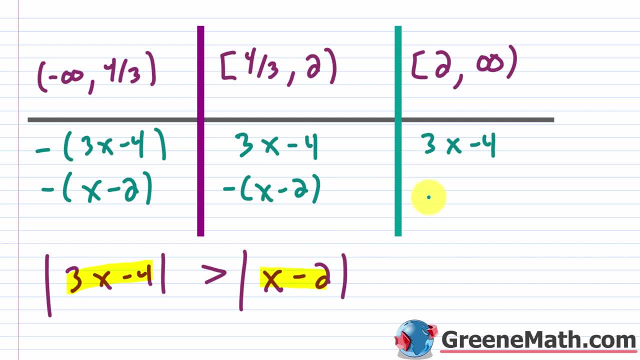 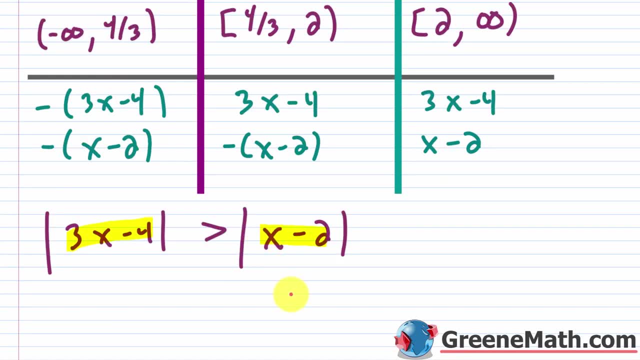 be positive. So for that, if it's 0 or positive, just drop the absolute value bars. So this is x minus 2.. Okay, So this gives us our setup, And once we've done all this work, we just go through and set up our inequality in each. 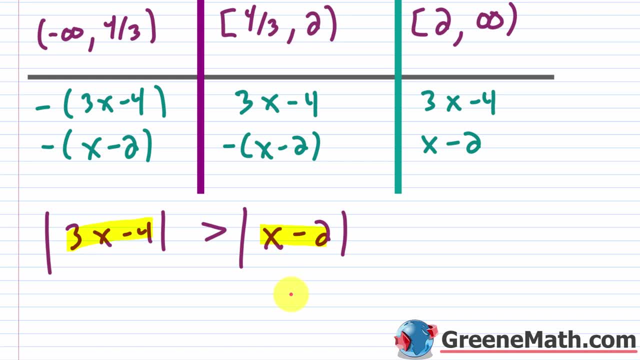 interval. See if it fits in the interval. If it does, we can accept it, If it doesn't, we can reject it. And then at the end we're going to think about everything together and try to merge. So we're going to think about this first guy, where both of these are negative. 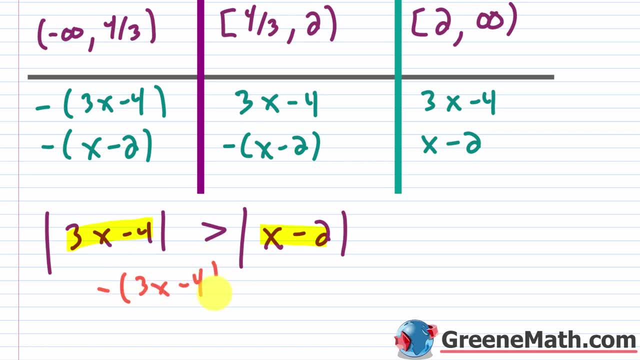 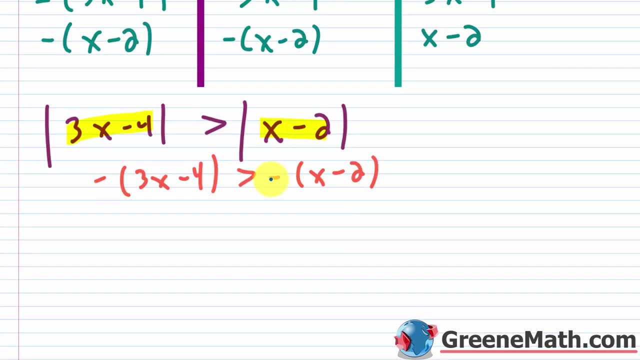 So I want the negative of the quantity 3x minus 4. And this is going to be greater than the negative of the quantity x minus 2.. So here you could distribute the negative into each, or you could just divide both sides by negative 1 and flip the direction of this. 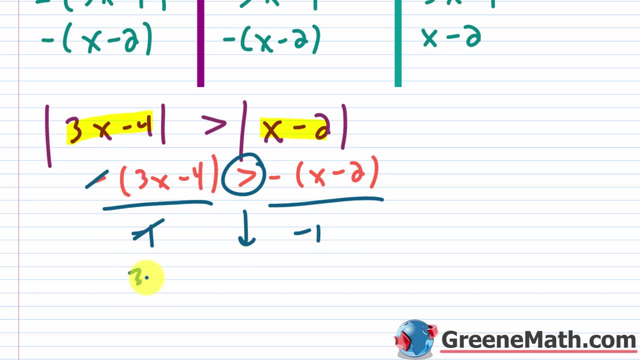 Again, that doesn't really matter, But this would cancel and you would have 3x minus 4.. I'm going to flip this to a less than, and this is x minus 2.. Maybe that's quicker, Maybe it's not. 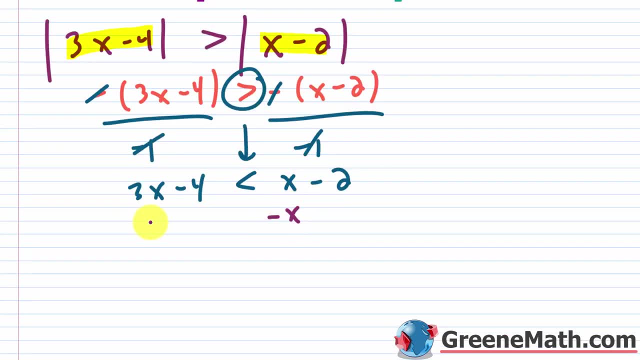 It just depends. Let me show this is canceling, so nobody's lost. So from here, I'm just going to subtract x away from each side of the inequality and I'm going to add 4 to both sides of the inequality. So let's show this is canceling and this is canceling. 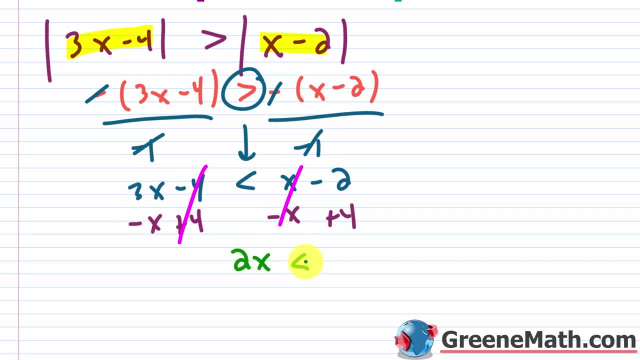 If we think about 3x minus x, that's 2x and this is less than negative. 2 plus 4 is positive 2. So that's 3 by 2. That will cancel And you'll get. x is less than 2 over 2 is 1.. 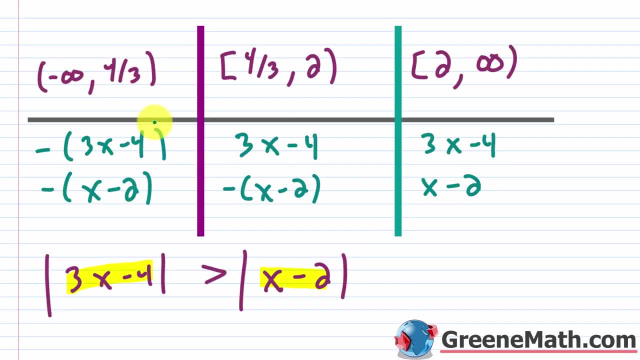 So we get: x is less than 1.. So coming back up and thinking about this, this interval is: x is less than 4 thirds, So that's 1 and 1 third. If I put x is less than 1, that's in that interval. 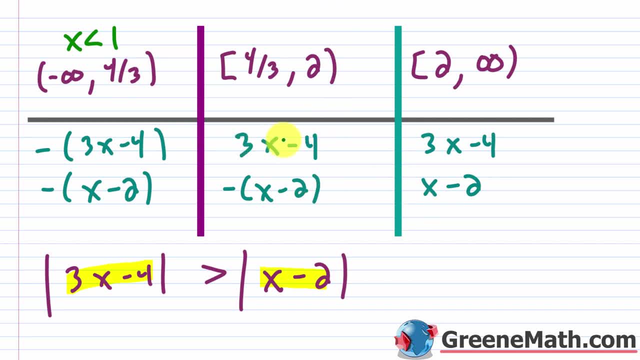 So you don't have to do anything there at all. So for this next one, this guy is going to basically be either 0 or positive. So we just drop the absolute value bars And then this guy right here is going to be negative. 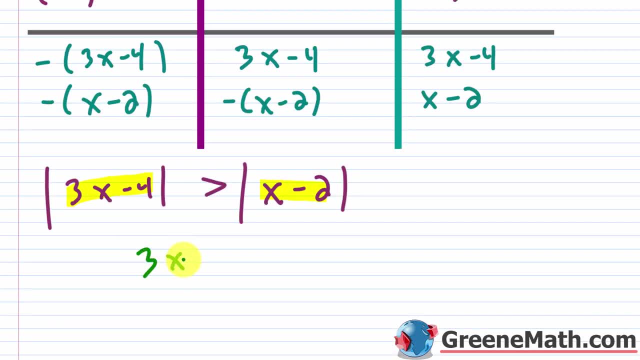 So I want the negative of the quantity x minus 2.. So let's go: 3x minus 4.. Okay, 3x plus 4 is greater than you can just distribute this now. This is the negative of x and then plus 2.. 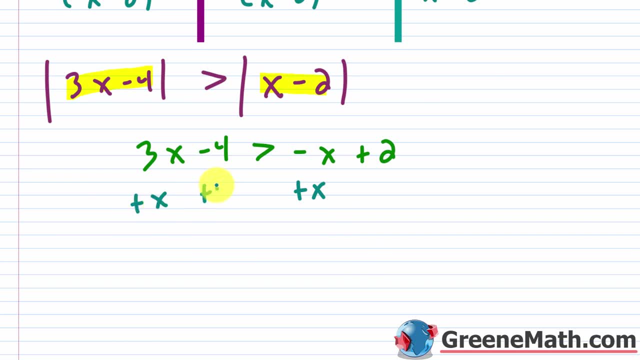 We will say that we'll add x to both sides of our inequality, add 4 to both sides of our inequality, And so this cancels, and this cancels. 3x plus x is 4x, and this is greater than 2 plus 4 is going to be 6.. 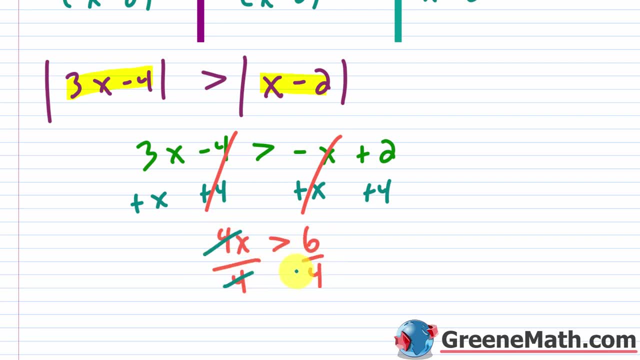 Let's divide both sides of the inequality by 4.. So this is going to cancel and we have: x is greater than for 6 and 4, they're each divisible by 2.. 6 divided by 2 is going to be 4.. 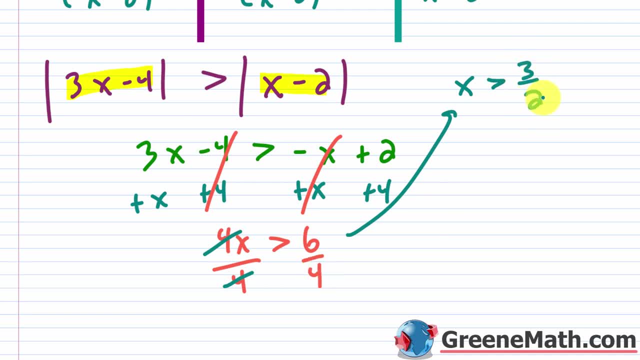 Okay, 6 divided by 2 is going to be 3. And 4 divided by 2 is going to be 2.. So you get: x is greater than 3 halves. So let's put: x is greater than 3 halves. 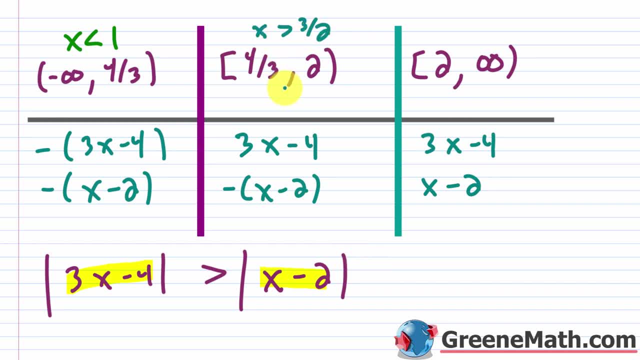 But there's an issue here. You can't just have: x is greater than 3 halves, because it has to be in this interval. Now, 3 halves is greater than 4 thirds. right, 4 thirds is 1 and a third. 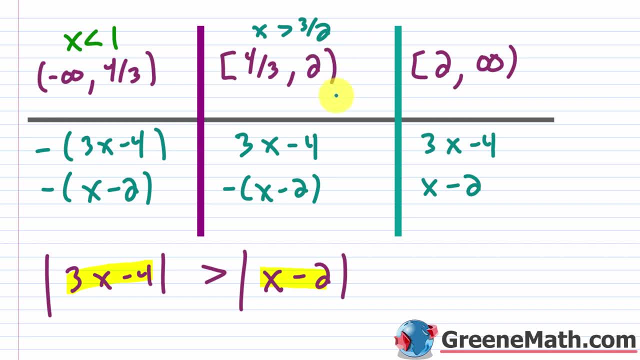 3 halves is 1.5. You would just want to adjust it to cut it off, to stay in the interval. So you would say that x is greater than 3 halves and you have to say that it's less than 2.. 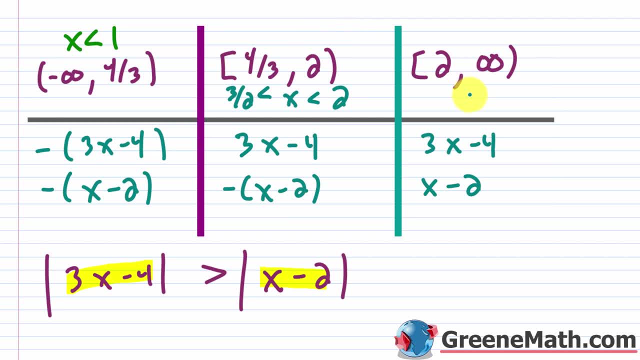 Because you have to stay in this interval. Now again, you might get something over here that works. I'm going to tell you in advance you do So. you're going to end up including 2, but we're not going to do it just yet because 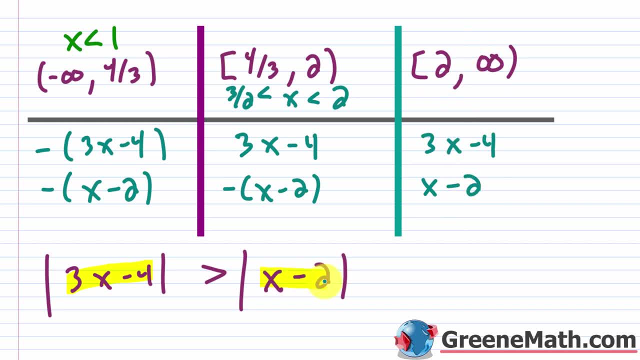 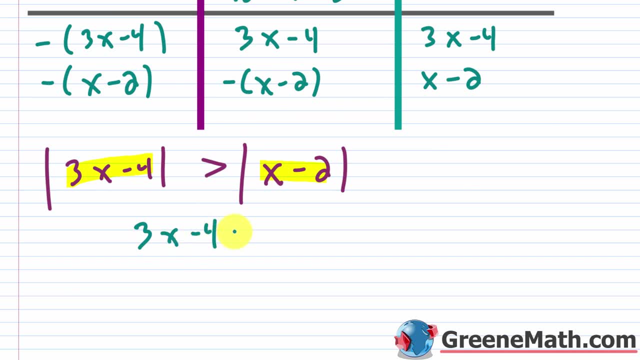 we're not there yet. Now, over here, everything is non-negative. For this one it's 0, or some positive value. For this one it's positive. So in each case you can just drop the absolute value bars, So you would have: 3x minus 4 is greater than x minus 2.. 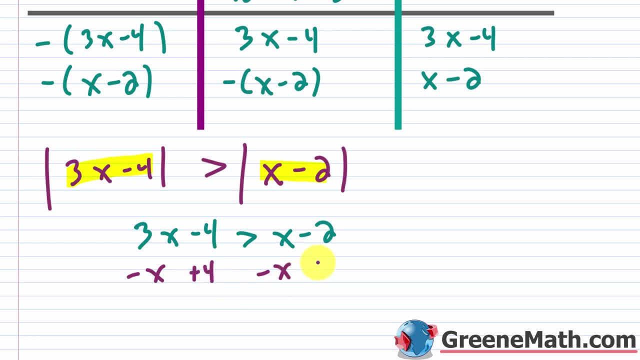 Let's subtract x away from each side of the inequality. Let's add 4 to both sides of the inequality. Let's cancel this and cancel this, And we'll say that 3x minus x is 2.. Let's add 4 to both sides of the inequality. 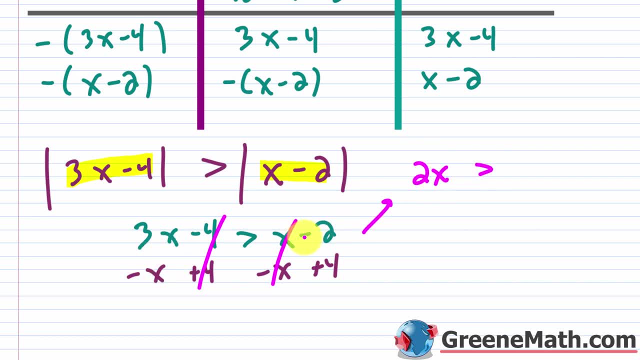 Let's cancel this and cancel this And we'll say that 3x minus x is 2x and this is greater than negative. 2 plus 4 is going to be 2.. Let's divide both sides of the inequality by 2.. 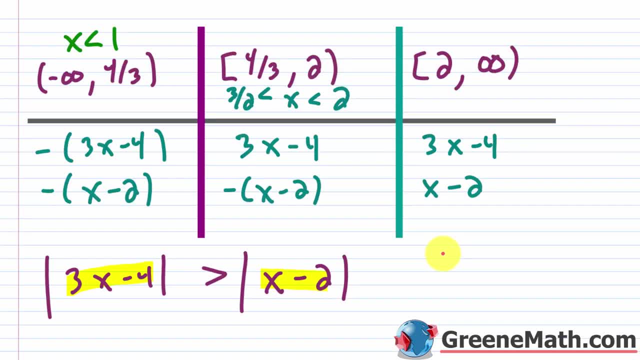 We'll cancel this and say x is greater than 2 over 2 is 1.. Okay, so let's come back up here and I'm going to write x is greater than 1.. Now we have to be in our interval and remember. the smallest value here in the interval is: 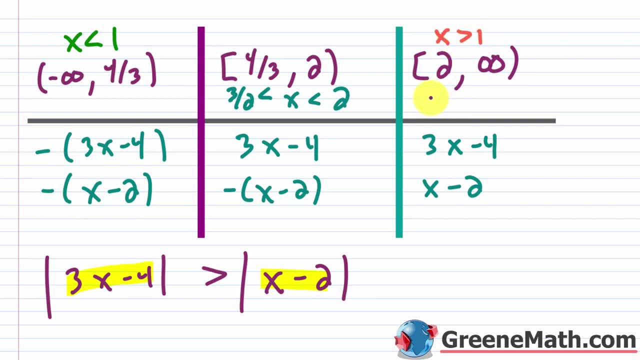 2. So I'm just going to adjust my solution to account for that and say here x is greater than or equal to 2.. Okay, So now we're ready to put everything together. Let's get rid of this. we don't need it anymore and you're going to put everything together. 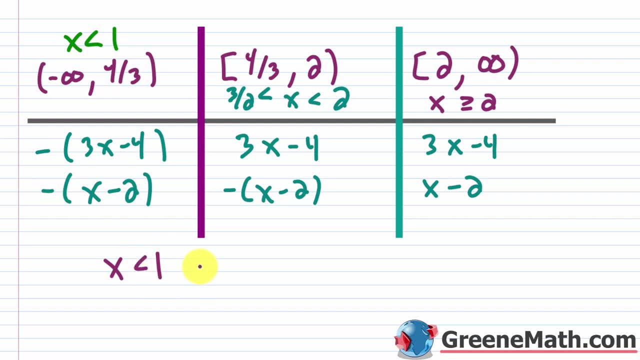 with the keyword or. So you're going to say that x is less than 1, then or you're going to say that x is greater than 3 halves and less than 2, then you're going to say, or x is greater than or equal. 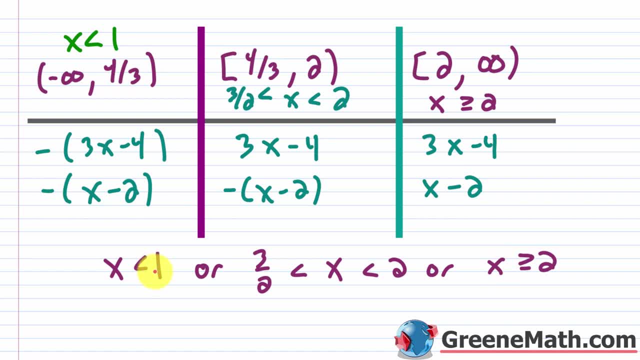 to 2.. Now this part right here on the left is straightforward: x is less than 1. nobody's going to get lost on that. But this part right here, I think, would trip a lot of people up. so let's spend some time on it. 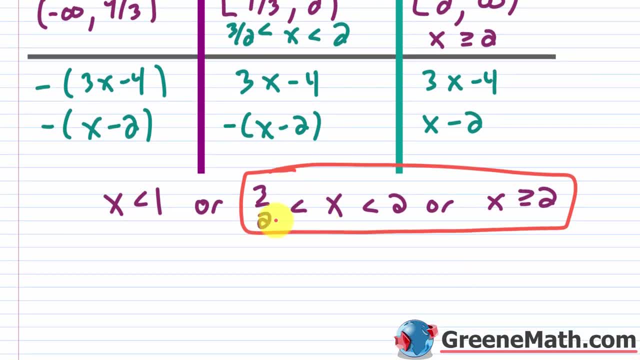 Okay. So let's start with the fact that here x is greater than 3 halves. So let me start by just writing that so x is greater than 3 halves. then you say and less than 2.. Okay, But then you have the keyword or here and you're saying x can be 2 or anything larger. 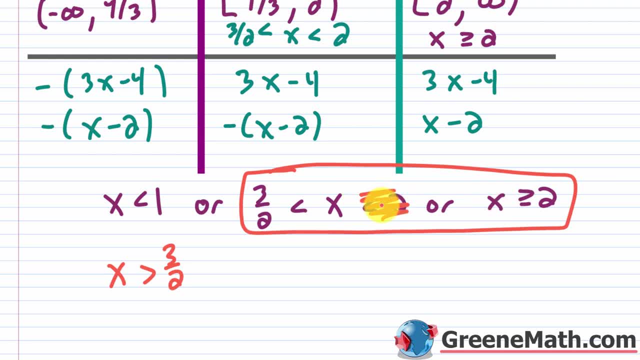 So really it's kind of like you can get rid of this part from this statement here, and if you considered x is greater than 3 halves, or x is greater than or equal to 2, well then it's just, x is greater than 3 halves. 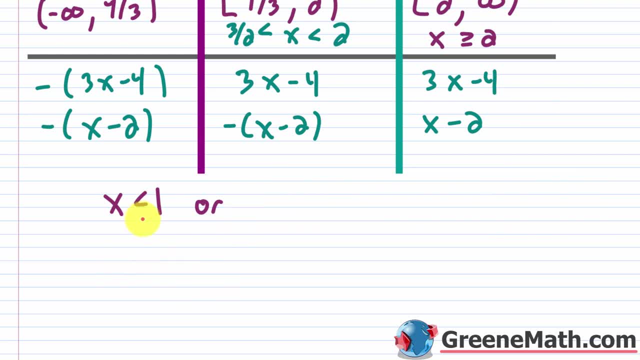 So you can actually just get rid of this all together and write your solution as x is less than 1 or x is greater than 3 halves, And I know that was confusing, but you might need to just pause the video. really think about what's going on. 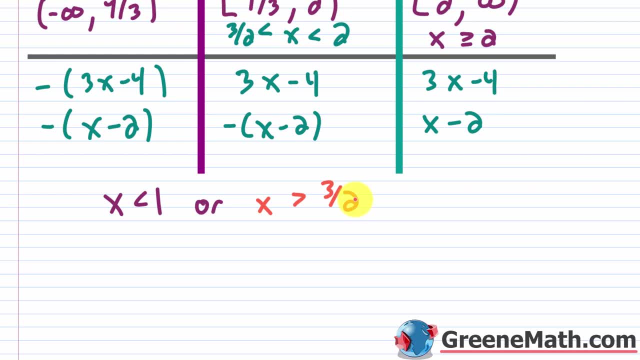 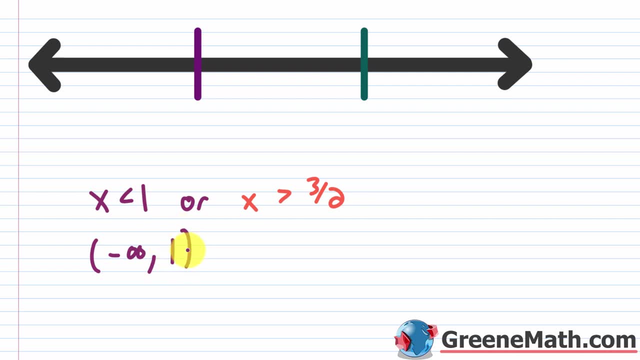 You can draw this out on a number line and consider everything. So let's grab this. So I'll say coming up from negative infinity and going up to, but excluding 1.. So make sure you use a parenthesis with 1, and then it's the union with you're going. 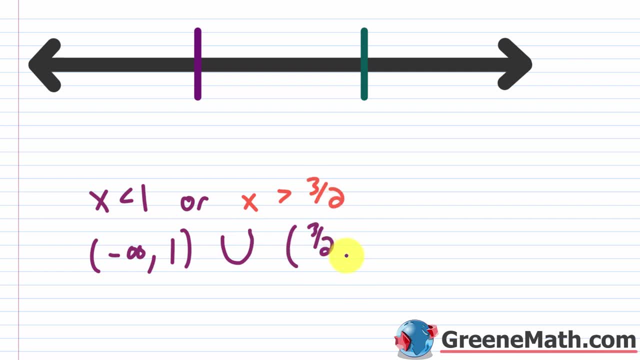 to use a parenthesis with 3 halves, because it's not included, So anything larger than that. so that's going to go out to positive infinity. So graphically you could find 1 on the number line. I'm just going to put a 1 here and then 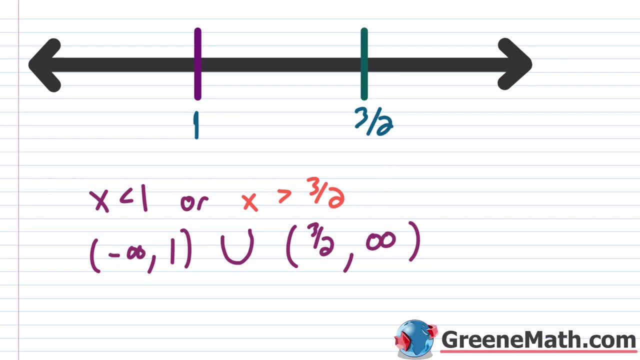 3 halves. I'll just put the 3 halves here and then, basically, I'm going to use a parenthesis with 1 and then I'm going to shade everything to the left here, and then I'm going to use a parenthesis with 3 halves and I'm going to shade everything to the right here and 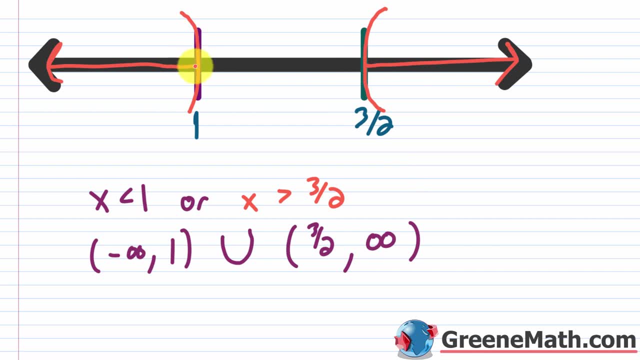 remember, you can always use an open circle instead of a parenthesis if that's what your book does. So we can see graphically that x can be anything that is less than 1, or x could be anything that's greater than 3 halves Alright. so once again, if you're struggling with these types of problems, you can graph. 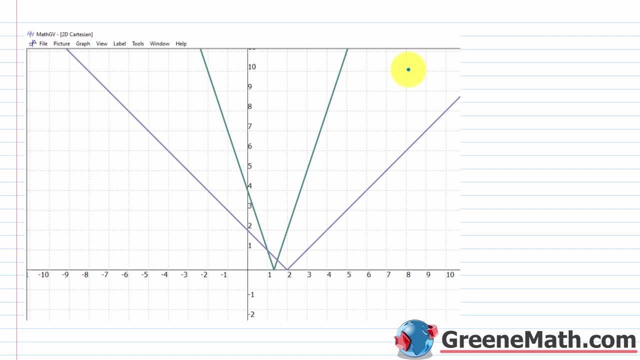 them use Desmos. We had the problem where we said the absolute value of 3x-4 is greater than the absolute value of x-2. So graphically we could say: this guy in green is y is equal to the absolute value of 3x-4. 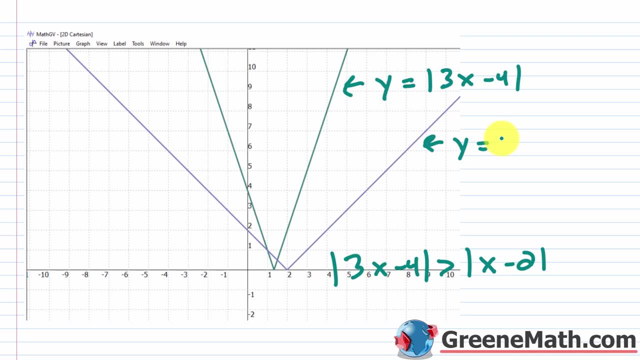 and this guy in purple, we could say this is: y is equal to the absolute value of x-2.. So, graphically, what we're saying is: where is the green graph? or again, the graph of y equals the absolute value of 3x-4. where is that above the purple graph or the graph of? 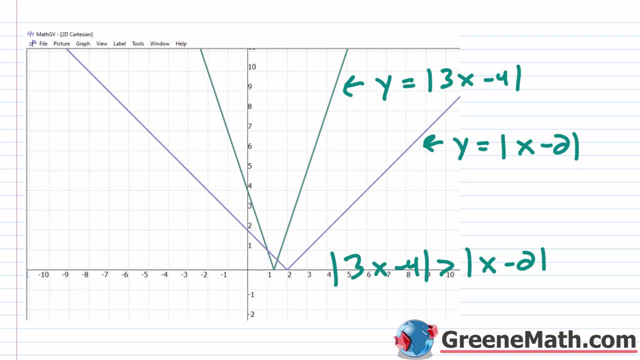 y equals the absolute value of x-2.. We can see where they cross and that's going to be important. So we have this 1 right here in terms of this x value. that's where the y values or the function values would be equal. and then also you have this other crossing point. this is going to 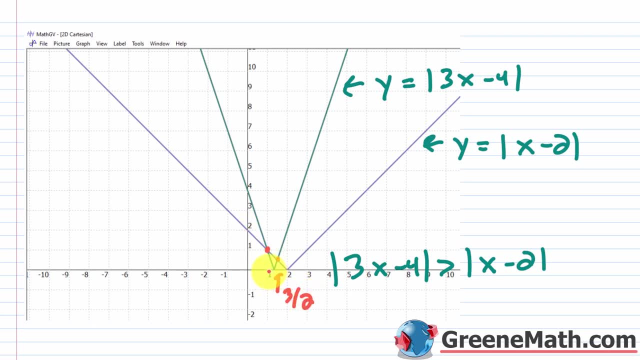 be 3 halves. remember we saw that everywhere to the left of 1 in terms of the x value, this green graph is above this purple graph. we can all see that. And everywhere to the right of this, 3 halves in terms of the x value, the green graph is: 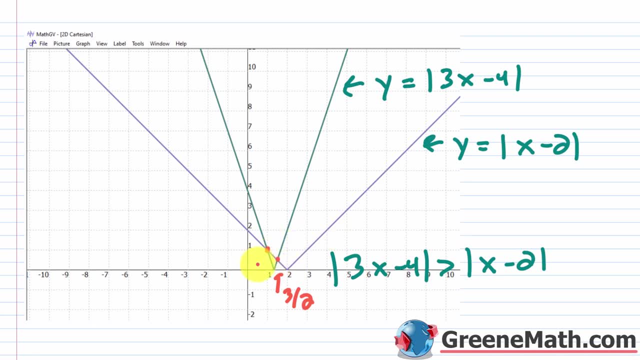 again above the purple graph. So graphically we can say the solution is x is less than 1 or x is greater than 3 halves. If this guy had been flipped and it was a less than well, then you're talking about this piece in between. 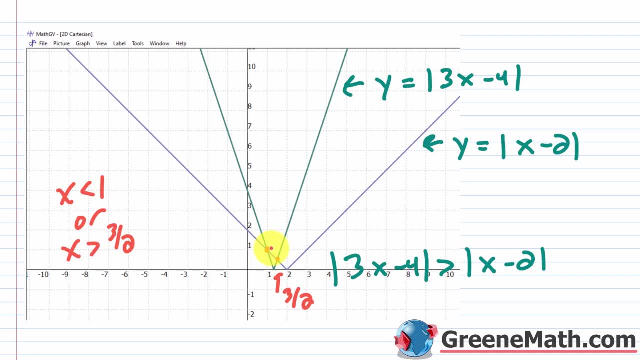 So there it would be, that x is greater than 1 and less than 3 halves. so again, really easy to see what's going on when you graph these guys. I strongly suggest this if you're struggling with these problems. All right, let's move on now and look at problem number 3. so we have x plus 3 is greater than. 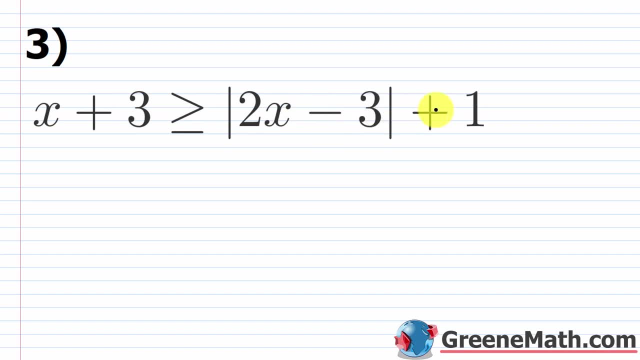 or equal to. we have the absolute value of 2x minus 3 and then plus 1.. So with this one we don't have two absolute value operations, we only have one. so it's going to make it a little bit easier, let's just copy the problem. so we have x plus 3. 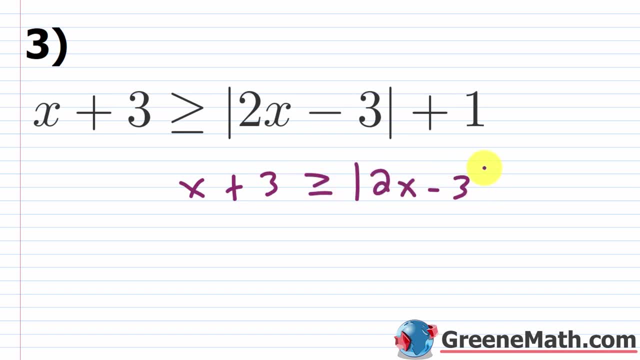 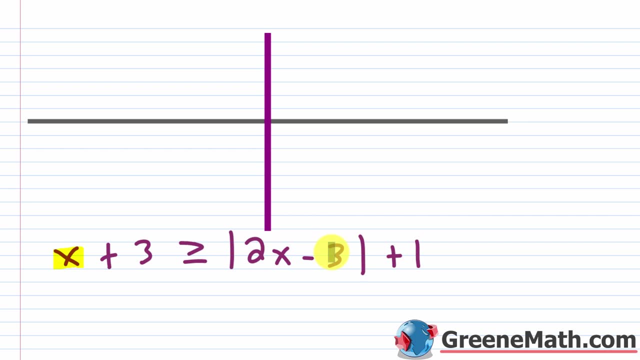 is greater than or equal to the absolute value of 2x minus 3 and then plus 1. now, because we have this x Here, that's outside of the absolute value bars over here we still have to do a little bit more work. so we have a table here, but it's just going to be two intervals, okay. so 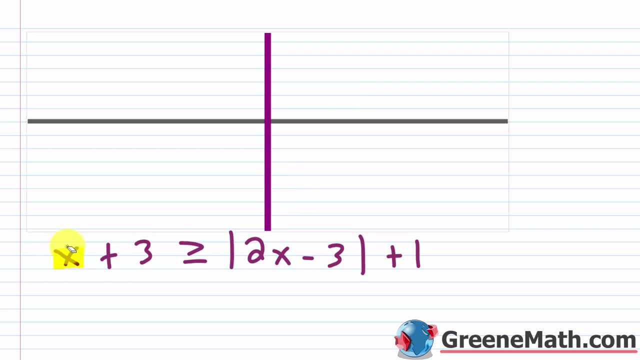 we don't need three intervals here. so you're just going to consider- now let me unhighlight this so nobody gets confused- you're just going to consider where 2x minus 3 is equal to 0 and then basically let's set that up: so 2x minus 3 is equal to 0, let's add 3 to both. 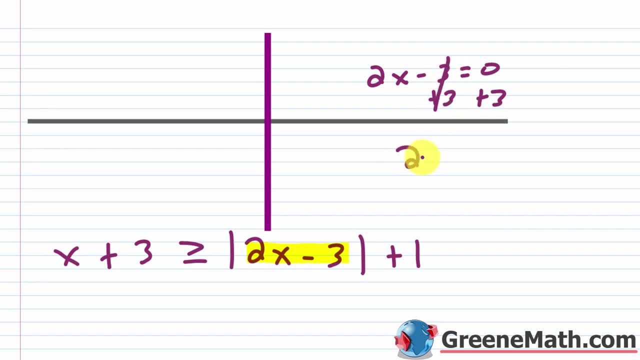 sides. we make that 3 a little bit better, we'll cancel this. we get 2x is equal to 3. divide both sides by 2.. We get x is equal to 3 halves. so we know if x is less than 3 halves. so basically coming. 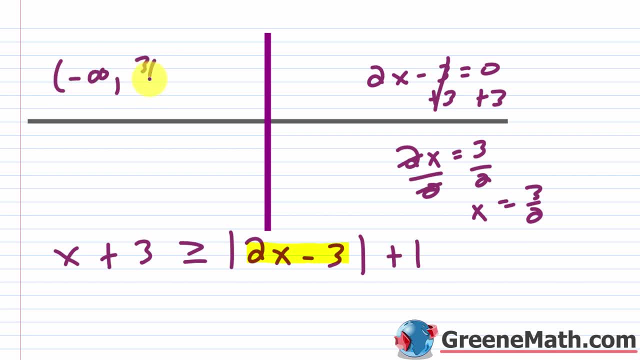 from negative infinity going up to, but excluding 3 halves, that this guy right here, this expression is going to be negative. so we want the negative of the quantity 2x minus 3. so that's the rule. if we drop the absolute value bars, Now anything where we are at 3 halves or greater, well, this guy would be 0 or some positive. 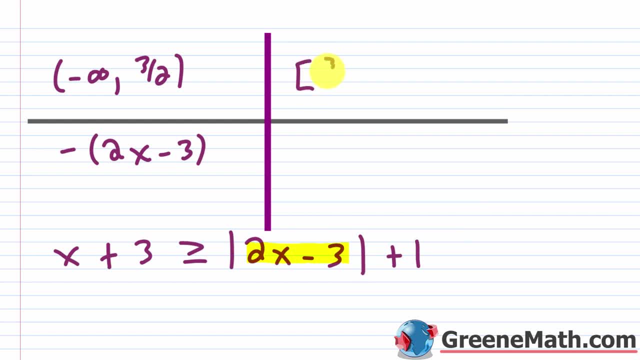 value. so we could just drop the absolute value bars. so I'm going to include 3 halves here and go out to play. So we have our rule. we just have to solve two inequalities. so let's see, with the first one I have, x plus 3 is greater than or equal to. we'll replace this guy with this guy. so 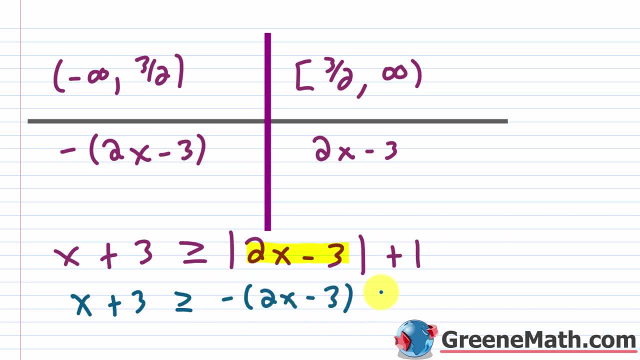 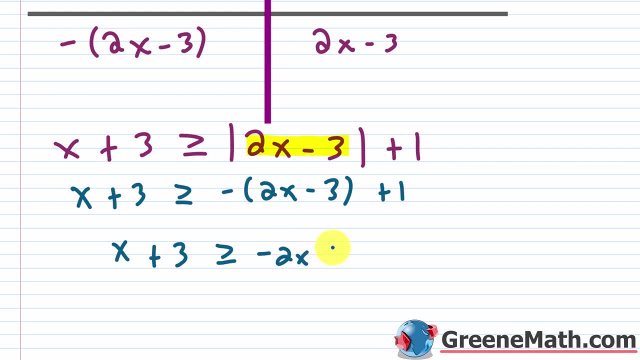 I have the negative of the quantity 2x minus 3 and then basically we have plus 1.. Okay, so we have x plus 3 is greater than or equal to- let's go the negative of 2x and then plus 3 and then plus 1. now you notice that you have 3 here and 3 here. you could subtract. 3 away from here. Okay, so let's spray the negative of 2x and then this crazy thing I'm going to do is we're going to divide by 2 and then we're going to cancel the negative 2x and then we'll have. 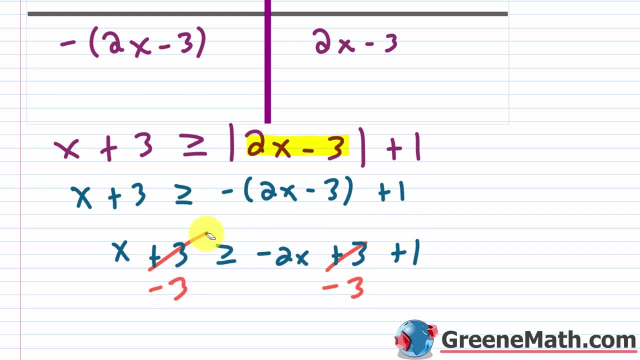 the negative of 2x. that's sad, but let's just go ahead and do the negative minus 1, and then we're going to add 2x, and then we're going to add 2.. Let me actually just show that so that nobody is lost, and I'll cancel like this. so it's. 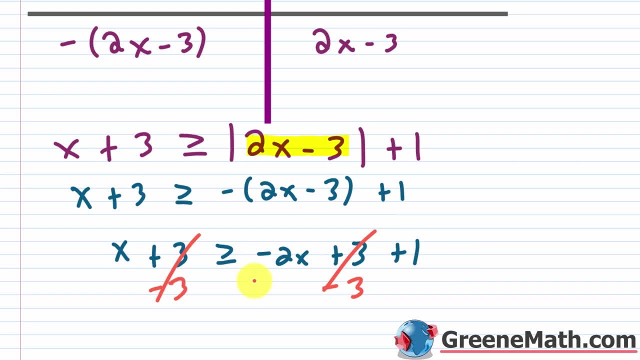 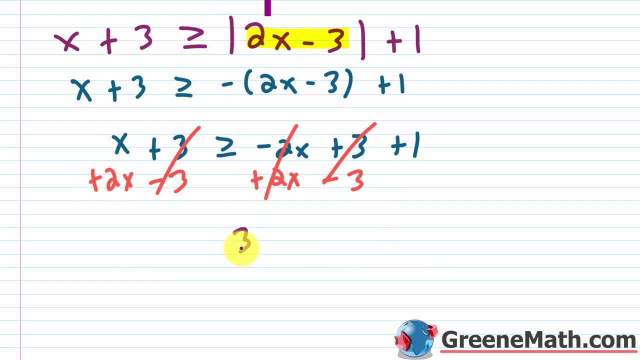 a little bit more clear what's going on. Okay, from here, I'm going to add 2x to both sides of the inequality and I'll cancel this. and so what do we have left? We have x plus 2x. that's 3x. this is greater than or equal to 1. we'll divide both sides. 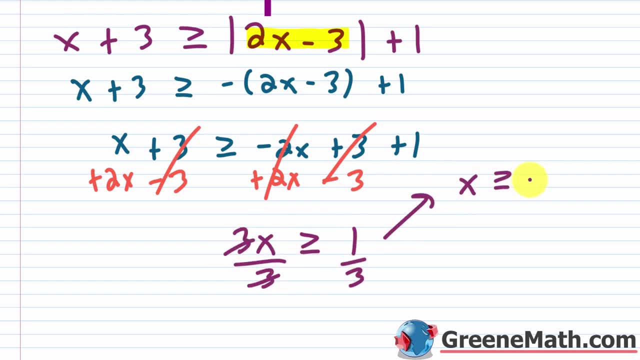 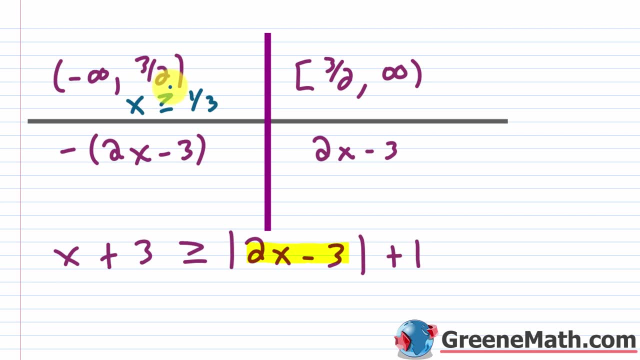 of the inequality by 3, this will cancel and you get: x is greater than or equal to 1 third. so let's put that x is greater than or equal to 1 third. is that in our interval? Remember, the interval is basically going to be anything that's less. 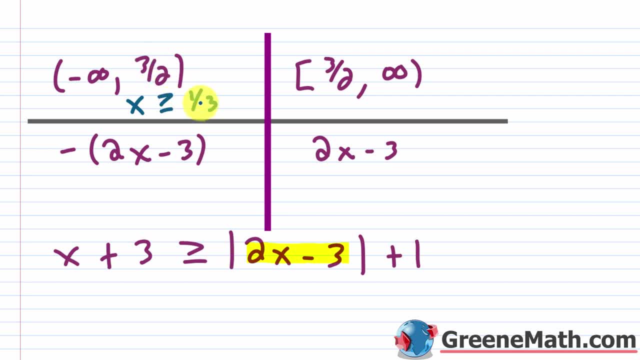 than three halves. So one third would be in this interval. The only problem is when you write it, you want to stop at anything that's less than three halves. So you would say that x is greater than or equal to one third and less than three halves. So that's what we want to do there. Okay, 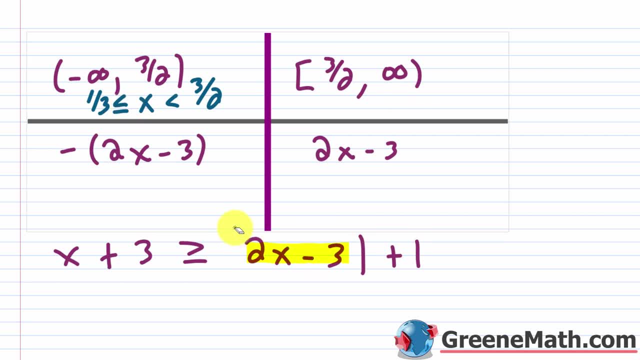 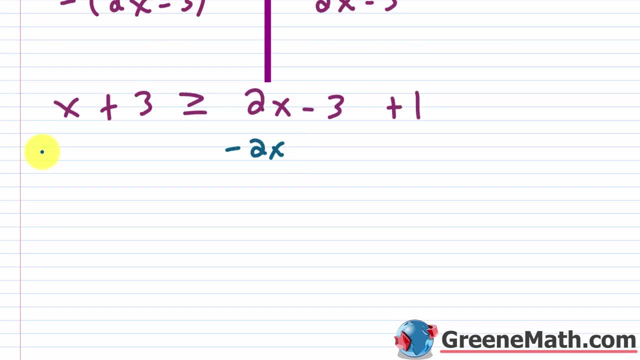 for the next guy here you're just going to drop the absolute value bars. So I'm just going to get rid of this and solve this inequality and see what that gives us. So here I will subtract two x away from each side of the inequality. cancel this. let's subtract three away from each side. 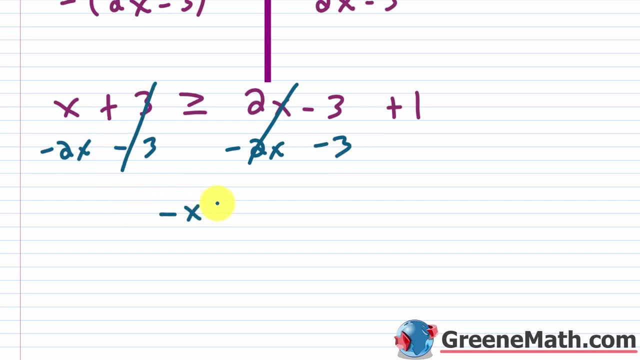 And so this would cancel and we'll say x minus two, x is negative, x, this is greater than or equal to. you basically have negative three minus three, which is negative six, and then plus one, that's gonna be negative five. Let's divide both sides of the inequality by negative one. 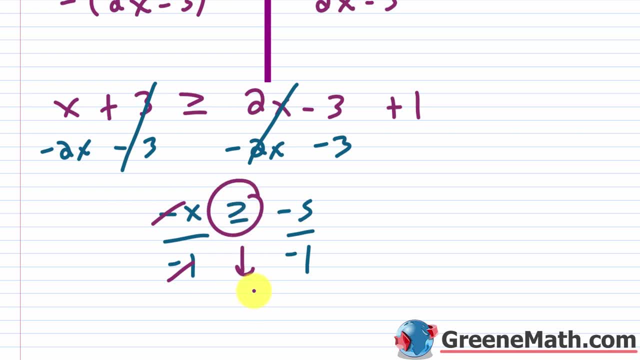 So this cancels. we're going to flip this because we divided by a negative, So this is going to be negative one. So we're going to flip this because we divided by a negative. This is less than or equal to- let me write my x in there and negative five over negative one is. 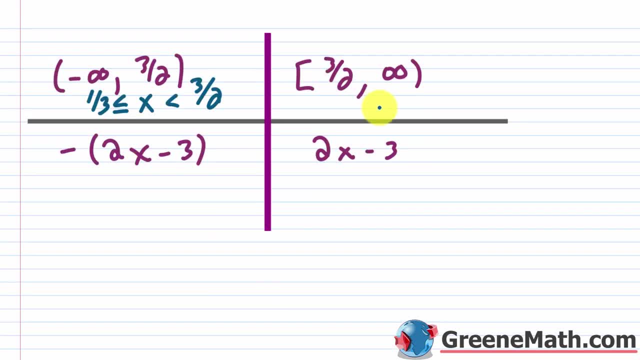 five. So you get: x is less than or equal to five. So let's write in here that x is less than or equal to five. Now again, you have to consider that this interval is going to start at three halves. So I'm going to basically rewrite this and say that x is greater than or equal to three. 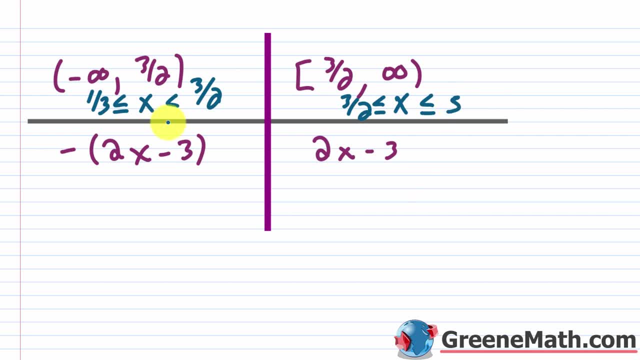 halves and less than or equal to five. So if you put these two together, you're basically saying that x is greater than or equal to one third And less than three halves. then, or x is greater than or equal to three halves. 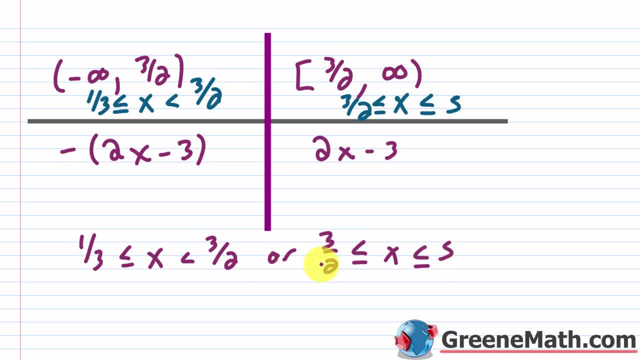 and less than or equal to five. Well, this guy right here includes the three halves, right? So three halves is included. So basically, if you put these together, you would say that x is greater than or equal to one third and less than or equal to five. 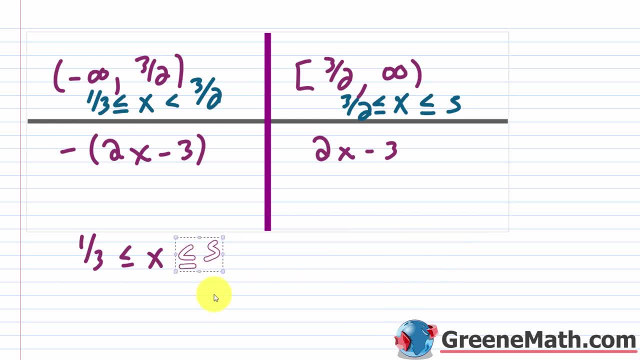 Okay, so let's just get rid of this And I'll just slide this down. So that would be your answer. So x is greater than or equal to one third and less than or equal to five. So in interval notation we're going to put a bracket. 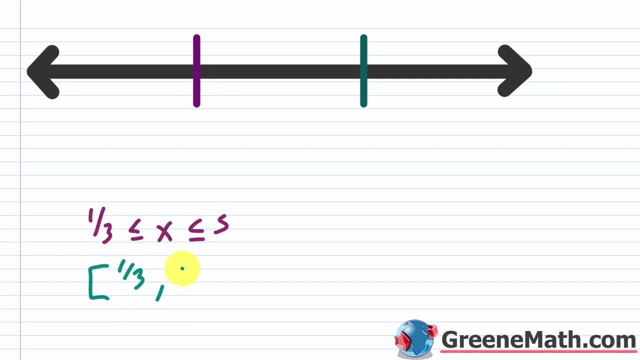 Next to one third because it's included, And then I'm going to put a bracket next to five because it's included. So basically, it's between one third and five where both are included. That's all we're saying. Let me put a one third here and a five here, And so I'm going to put a bracket here. 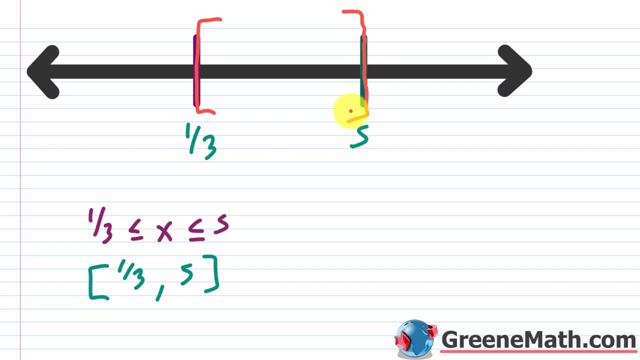 at one third to show what's included, and a bracket here at five to show that it's included Again. if you want to use a filled in circle, if your book does that, that's fine. it means the same thing, And so I'm just going to shade everything in between. So x here graphically. 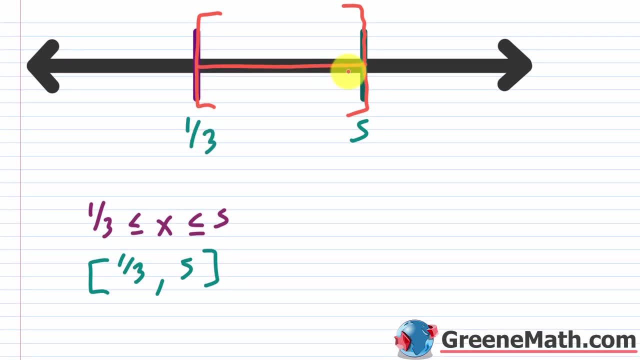 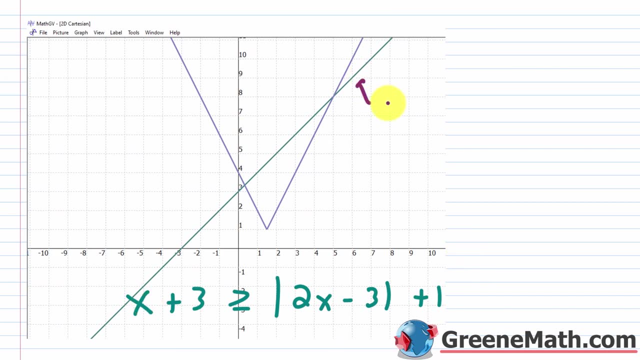 can be one third or anything going up to and including, So I'm going to put a bracket here at one third or anything going up to and including five, All right, so once again, you can look at this graphically. So you're going to graph this guy in green here. this is just a simple linear. 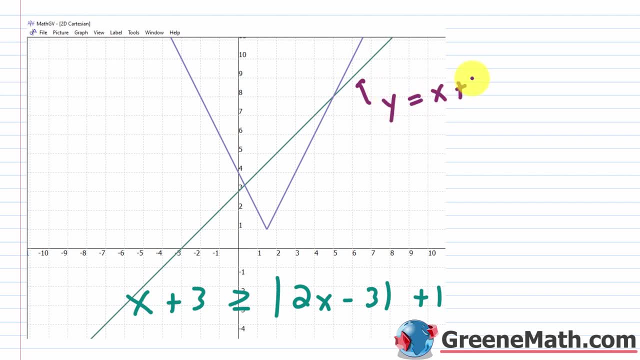 equation in two variables. This is y is equal to x plus three. a lot of us know how to graph that already. So the y intercept is at zero, comma three, and the slope is one right. so go up one to the right, one, so on and so forth. Then this other part here, the part on the right. this is this: 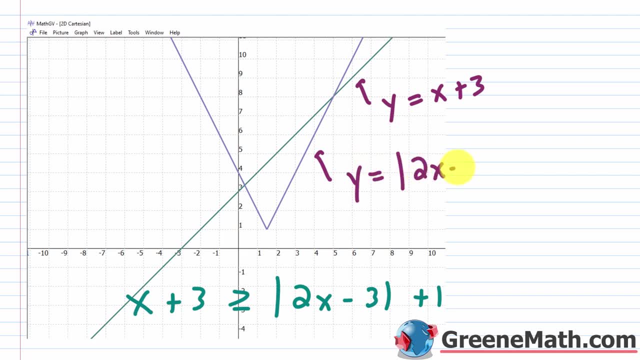 guy in purple. this is: y equals the absolute value of two x minus three and then plus one. Okay, so if you don't know how to do that, you can do that by looking at the graph here. So if you don't know how to graph this again, you can just use a computer generated graph for right now. 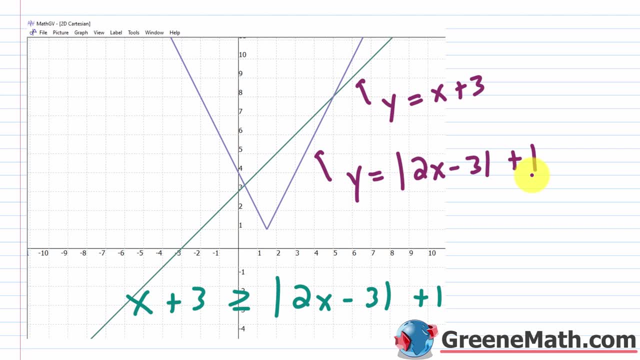 we'll talk about how to graph this stuff later on in the course, But I just want you to see that basically I'm asking: where is this guy, this x plus three, or this y equals x plus three, or this green graph above, or equal to this other guy here? this y equals the absolute value of two. 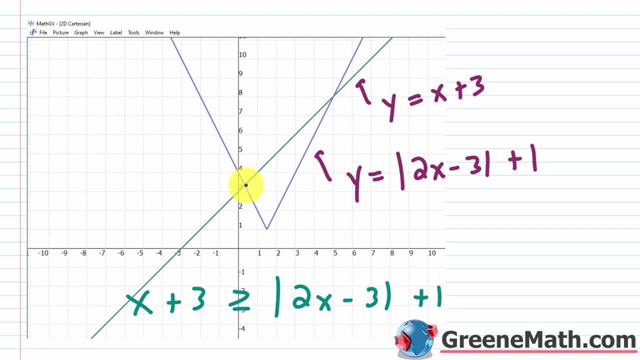 x minus three plus one, this purple graph. Well, you can see they're equal here and here, right. And so this right here, the x value would be one third, And this right here x value would be five. right, So that's where they're equal. And then, essentially, 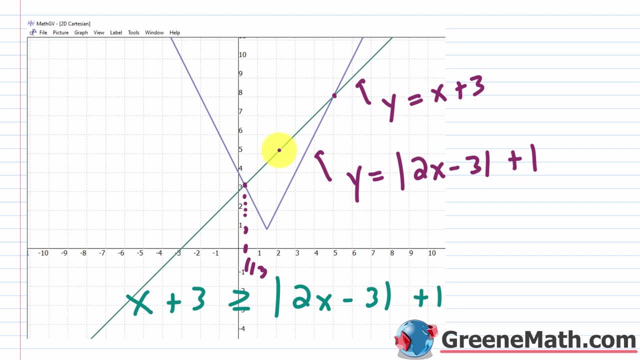 between those two values. you can see the green guy is going to be above the purple guy, but nowhere else, right? So we could say that the solution graphically is that x is greater than or equal to this one third and less than or equal to five. So this is exactly what we saw. 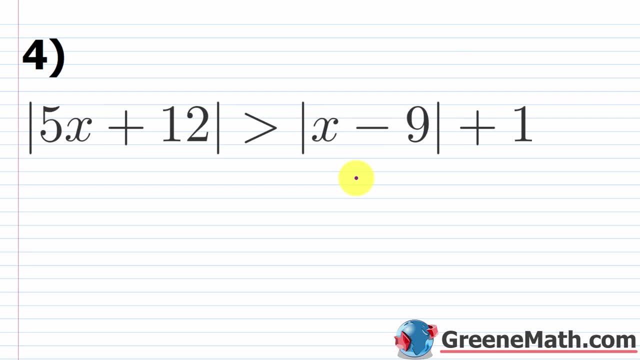 from solving the problem. All right, let's take a look at problem number four Now. so we have: the absolute value of five x plus 12 is greater than the absolute value of x minus nine, then plus one. right, let me copy this. So the absolute value of five x plus 12 is greater. 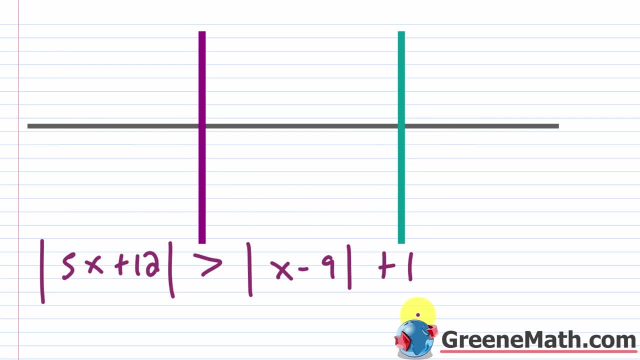 than the absolute value of x minus nine, then plus one. So again we're back to having two absolute value operations. So I've got to set this equal to zero and solve. and set this equal to zero and solve. let's go. five x plus 12 is equal to zero. I'll subtract 12 away from each side. I'll cancel. 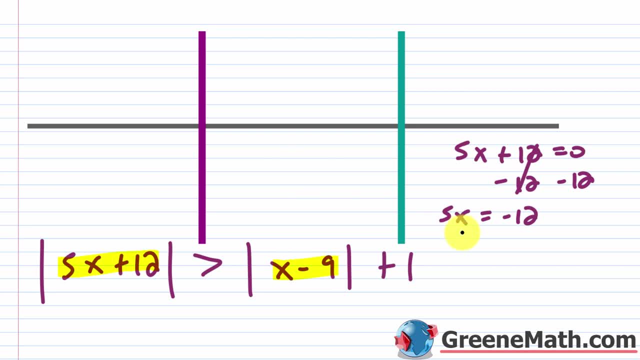 that five x is equal to negative 12.. And so what I'll do here is divide both sides by five. we'll cancel this And say x is going to be negative 12.. So I'm just going to write this right here. It's just: 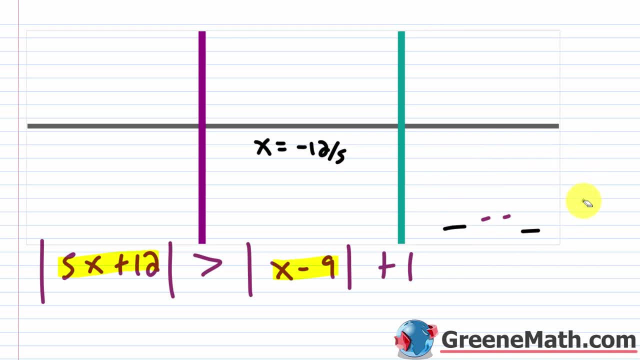 scratch work. I'll move it in a second. Let me get the other one going. So this is just: x minus nine is equal to zero. And of course we just add nine to both sides of the equation. we cancel that, we get x is equal to nine. So the leftmost value here is this: negative 12 fifths. So I'm going to say: 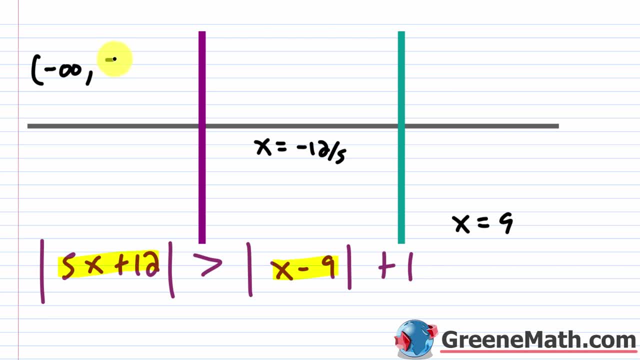 that, coming from negative infinity, going up to and excluding negative 12 fifths, And then again, here I'm going to include negative 12 fifths And we're going to go up to and exclude nine, and then here I'm going to include nine and then anything larger. Alright, so we've got the. 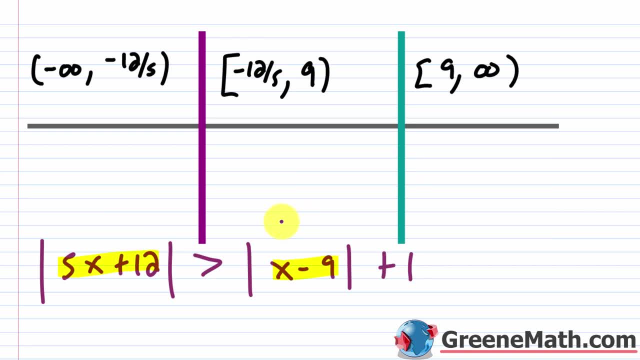 intervals. going In this leftmost interval, we know both of these guys are going to be negative, So I want the negative of the quantity five x plus 12.. Let me just speed this up and say this is negative: five x minus 12.. Just so we don't have to deal with that. So let's get rid of this. 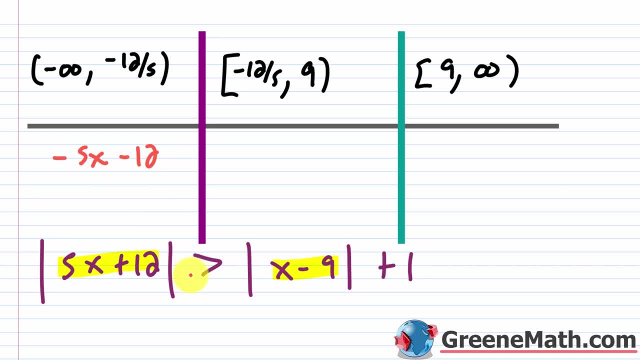 and scooch that up And then basically in this interval here this guy is going to be zero or positive, drop the absolute value bars, So this is five x plus 12. And then again here will be positive. So this is five x plus 12.. Okay, for the other guy this x minus nine. in this first interval, 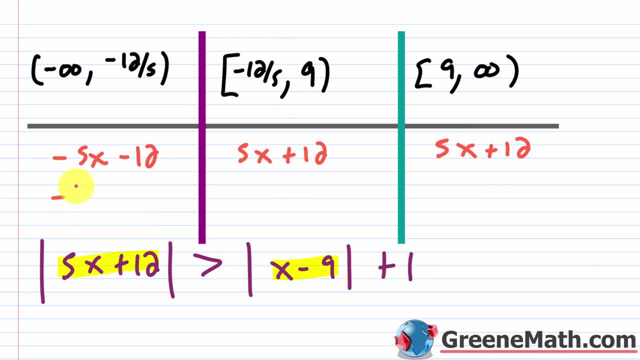 in the second interval it's going to be negative. So you want the negative of the quantity x minus nine, which is negative x plus nine. So negative x plus nine and then negative. let me make that better. So negative x plus nine. Okay, here it's either going to be nine, where it's zero. 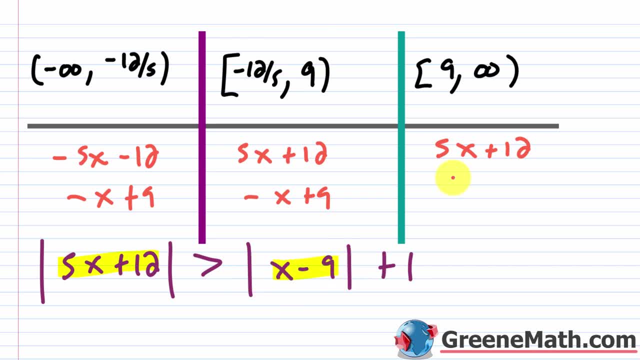 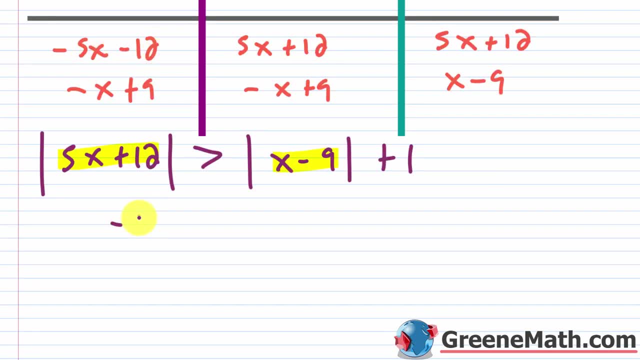 or it's going to be some positive value. So in that situation you can just drop the absolute value of negative x minus nine. Now we just have to go through and solve our inequalities. So for the first interval I'll just say negative five x minus 12 is greater than you'll have this negative. 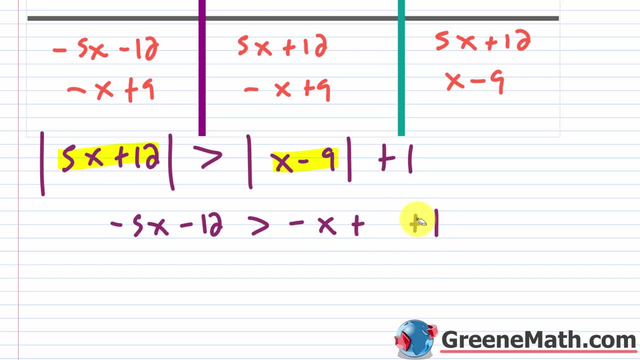 x plus nine and then plus one. So nine plus one is 10.. Let me just replace that now And so really quickly. I could just add 12 to both sides of the inequality. Let's cancel this. I'm going to add x. 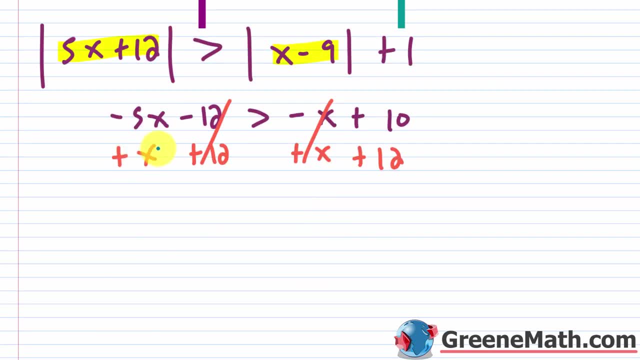 to both sides of the inequality. Let's cancel this And let's say negative five. x plus x is negative four. x, this is greater than 10 plus 12 is going to be 22.. Let's divide both sides of the inequality by negative four. we'll cancel this and say x is. 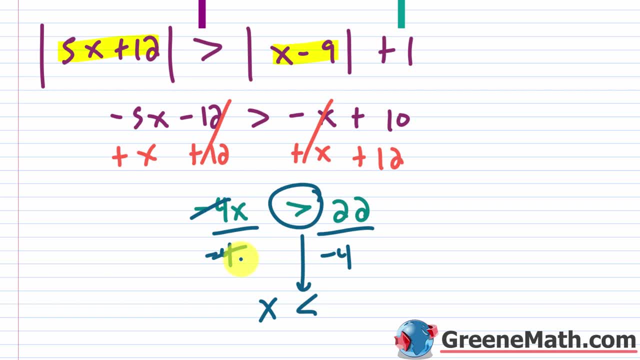 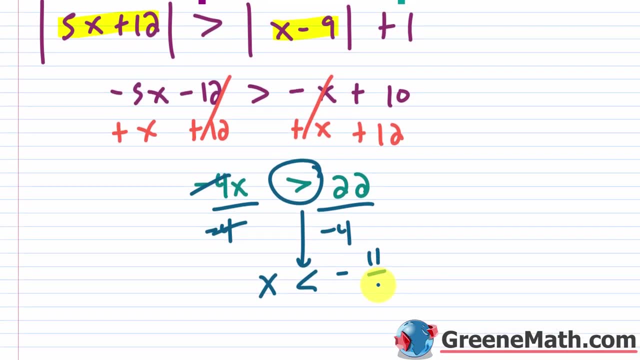 less than. let me show this: The reason I flipped this again is because we divided both sides by a negative And then 22 over negative four. we know that's negative. 22 divided by two is 11.. And four divided by two is two. So this is negative. 11 halves here. So let me grab this. So, coming back, 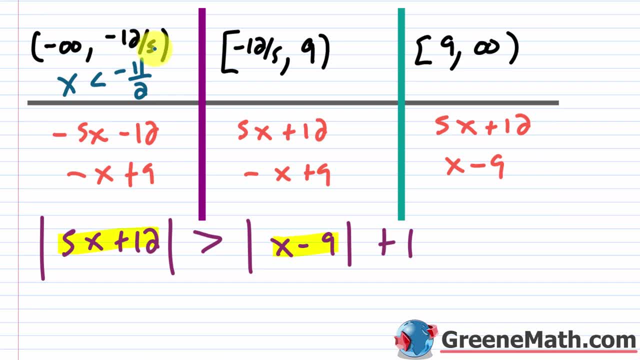 up here. this guy will be within this interval. If you do negative 12 divided by five on your calculator, you get negative 2.4.. If you do negative 11 divided by two on your calculator, that's negative 5.5.. So this solution we can just accept it. we don't need to modify it in. 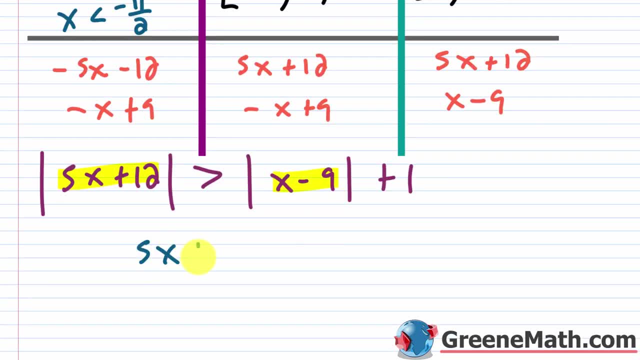 any way. So for this guy right here we can just say that five x plus 12,- just drop the absolute value bars- is greater than here. I want the negative, So negative x plus nine and then plus one. So again, nine plus one is 10.. So let me just replace that real quick, And so we'll add x to. 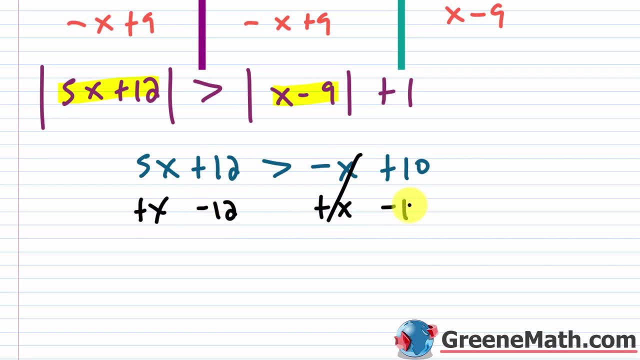 both sides of the inequality that cancels will subtract 12 away from each side of the inequality that cancels. So if you have five x plus x, that's six x and this is greater than 10. minus 12 is negative two. let's divide both sides of the inequality by six. this will cancel. 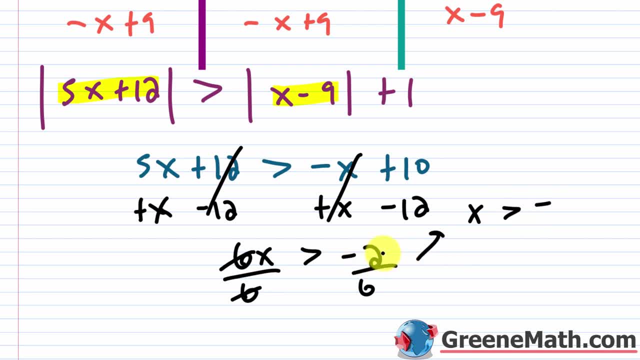 we get: x is greater than we know. this is negative. If you have two over six, each is divisible by two. two divided by two is one, and six divided by two is three. So x is greater than negative one third. So we have: x is greater than negative one third. Now again negative: 12 divided by five. 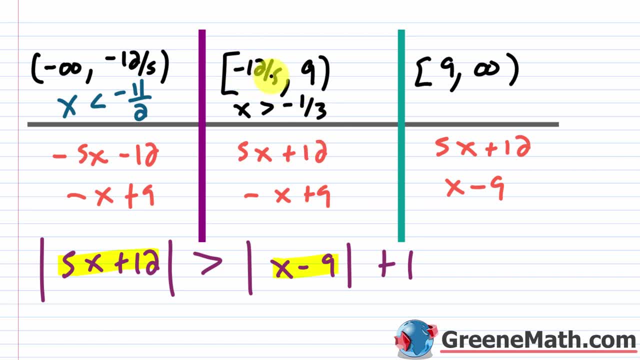 that's negative 2.4.. If I think about negative one third, that is greater than this. So I'm okay there. But again, you can only go up to anything that's less than nine to stay in this interval. So I'm going to say that x is greater. 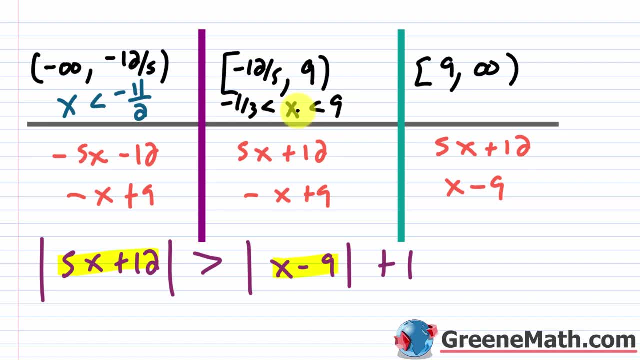 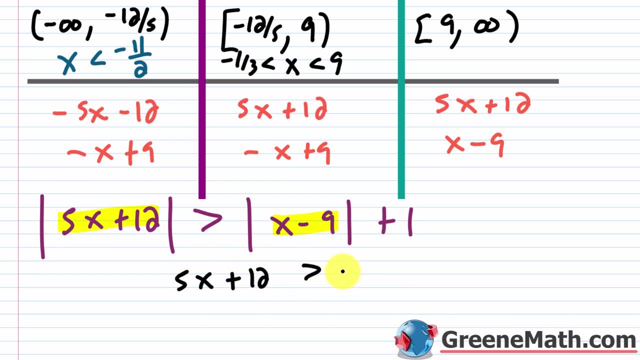 than negative, one third and less than nine. just to make that work in the interval over here, let's solve this one. So we're going to have five x plus 12.. And then this is greater than your x minus nine and then plus one. So we're just dropping the absolute value bars here, So negative. 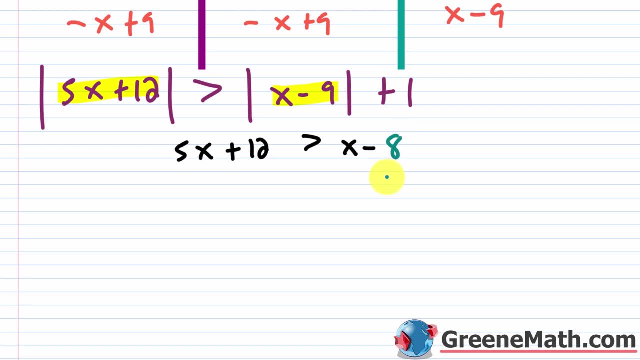 nine plus one is going to be negative eight. I'm just going to replace that, And then what I'll do is subtract 12 away from each side of the inequality that cancels. Let me subtract x away from each side of the inequality that cancels. So we think about five x. 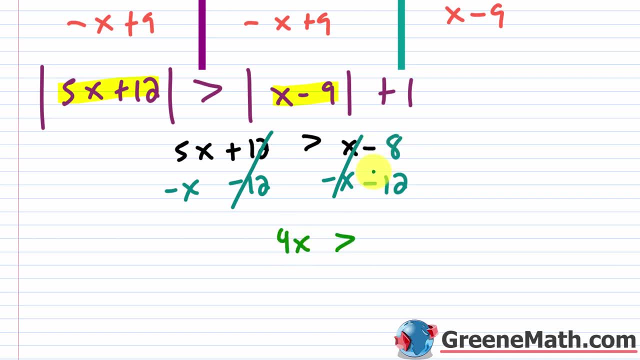 minus x, that's going to be four x and this is greater than negative. eight minus 12 is going to be negative 20.. Let's divide both sides of the inequality by four. So we're going to cancel this with this and say that x is greater than we know. this is a negative 20 divided by four is five. So 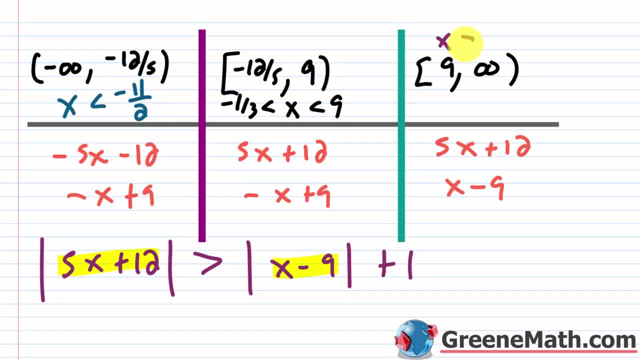 x here is greater than negative five. So we got a solution of x is greater than negative five. Now for this interval. this would only come into play nine. So we would only think about this as x is greater than or equal to nine. Because, again, 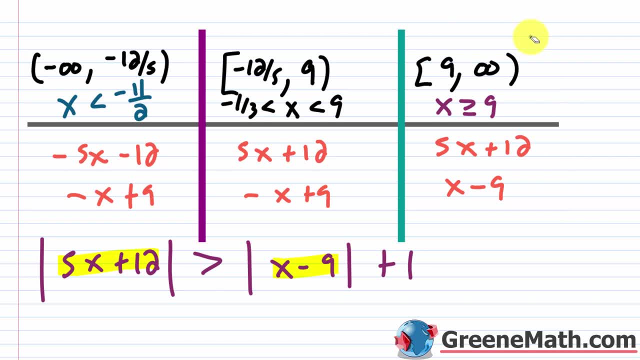 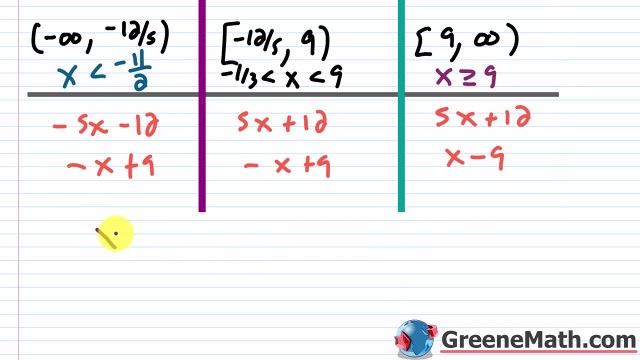 the rest of that is not in this interval. Okay, so we will get rid of this and use this. Okay, so let's put our solution together. And this is where people get confused. Let me erase this. So I have some room, So I'm going to start with. x is less than negative. 11 over two, that's easy. 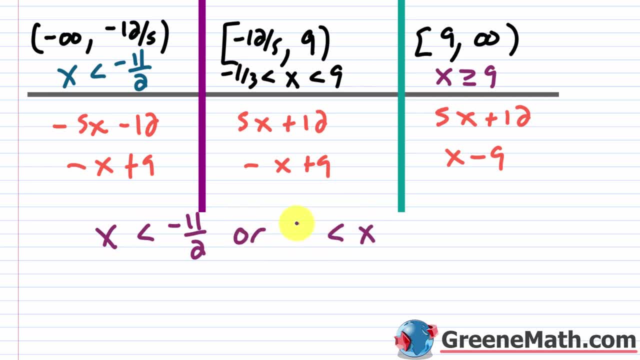 Then you're going to go, or this is where it gets complicated- So you have x is greater than negative one third and less than nine. then you have: or again you have: x is greater than or equal to nine- So I know this part right here- and then you have x is greater than or equal to nine, So I 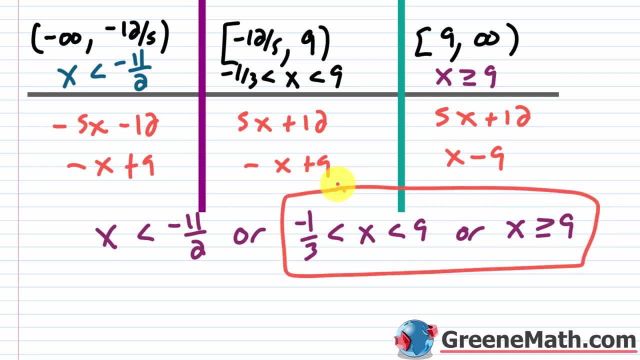 know this part here is super confusing for a lot of students, But just pause the video for a moment, just think about it. What's going on here? So this part is simple enough. So x is less than negative 11 over two. that's easy to understand. But here I want you to think about the fact that, although 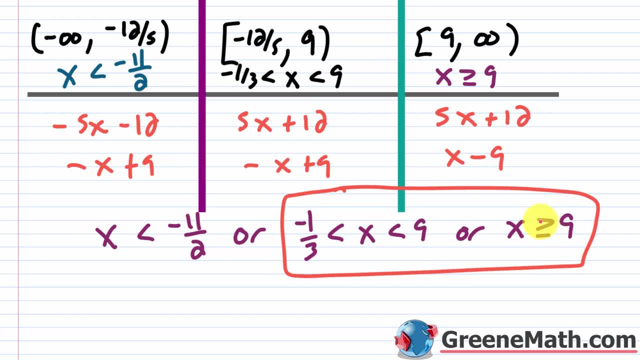 you have this: x is less than nine. here, here you have: x is greater than or equal to nine. So really you could just get rid of this right. You just not think about that. So if I had x was greater than negative one third, then, or x is greater than or equal to nine. Well, again this. 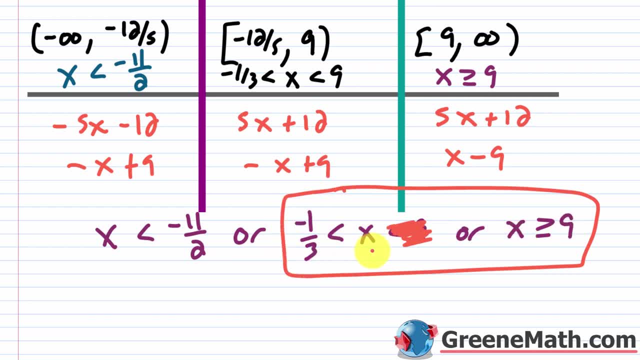 is or. so it can work in either. So I'm going to take the least restrictive right. So I'm going to go with x is greater than negative one third. So really you can get rid of this and just say: or x is greater than negative one third and an. 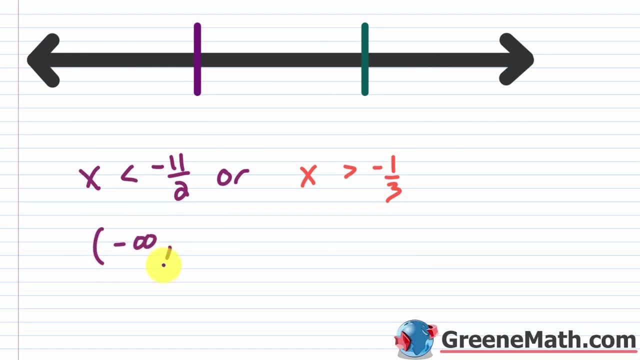 interval notation. So basically anything coming up from negative infinity going up to, but excluding negative 11 halves- I'll use a parenthesis there- And the union with anything that's larger than negative one third. So I'll use a parenthesis there. So this is going out to: 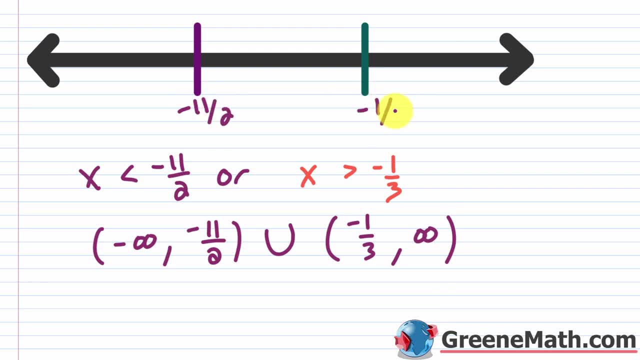 positive infinity. So let's say this is negative 11 halves and this is negative one third right. And again I'm going to use a parenthesis to exclude things. you can use an open circle if your book does that, So I'm just going to put a parenthesis here. facing to the left: 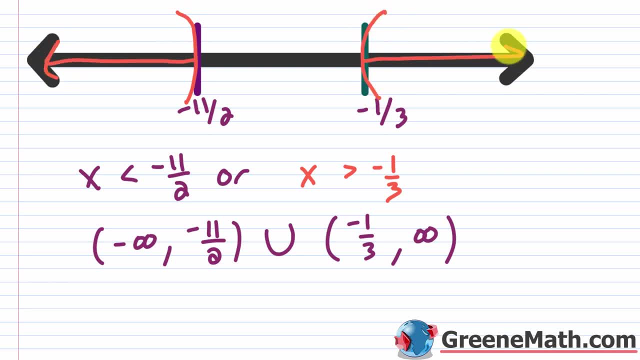 shade to the left and put a parenthesis here facing to the right shade to the right. So graphically, x is anything that's less than negative 11 halves, or anything that is greater than negative one third. Alright, so once again, if you're a little bit lost in this problem, 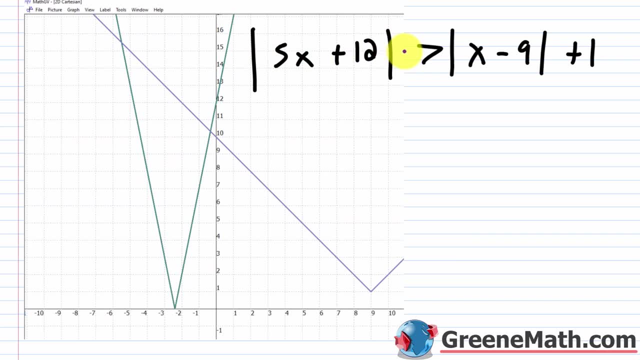 you can always graph it, So you're going to take the left side here. this is: y, equals the absolute value of x minus nine and then plus one, And this graph is cut off a little bit because it's kind of hard to display, But this would keep going up like that. it forms a V shape, But essentially 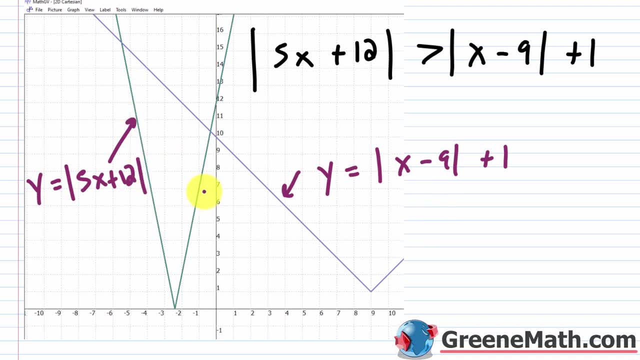 what you look at. here we're saying: where is the green graph above the purple graph? you can see where they intersect. So that's going to be here, And if you come down to the x value for that, it's going to be, let's say, negative, 5.5, or negative, or negative, or negative, or. 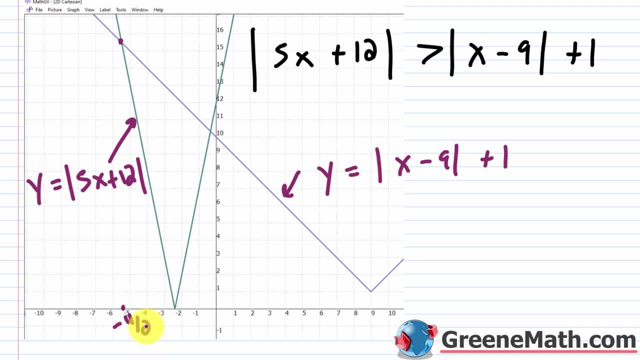 11 halves. I know that's not perfectly aligned there, But let's just say: that's good enough. And then here this is going to be our negative one third. Again, it's not perfectly aligned, but you can see. that's where it is. And then, basically, you can see that between these two, 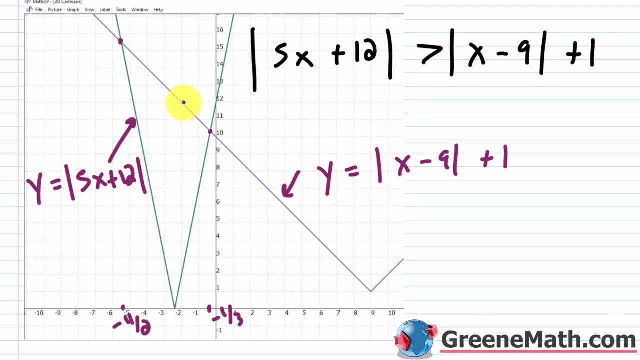 values. the purple graph, or the right side here, is actually above the green graph, But that's not what we want. We want the green graph to be above the purple graph, So that occurs anywhere to the left of negative 11 halves. So again we found that, as x is less than negative 11 halves, we're 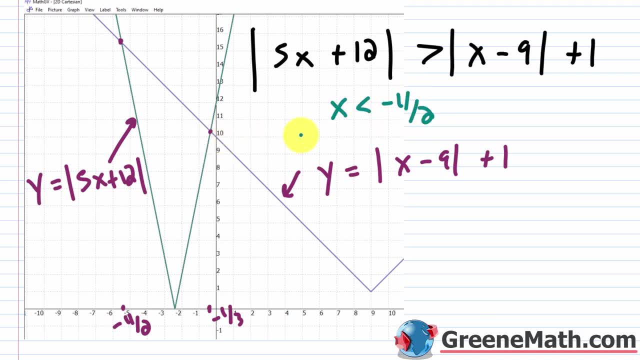 negative 11 halves, And that also occurs anywhere to the right of negative one third. So we'd say: or x is greater than negative one third. Okay, so this is how you can look at this graphically and make that a little bit better and find your same solution If you're confused about something. 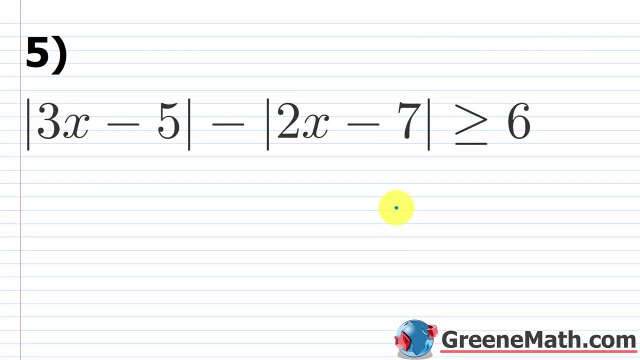 it's always good to stop and look at the graph. All right, let's take a look at problem number five now. So we have the absolute value of 3x minus five, then minus the absolute value of 2x minus seven. This is greater than or equal to six. 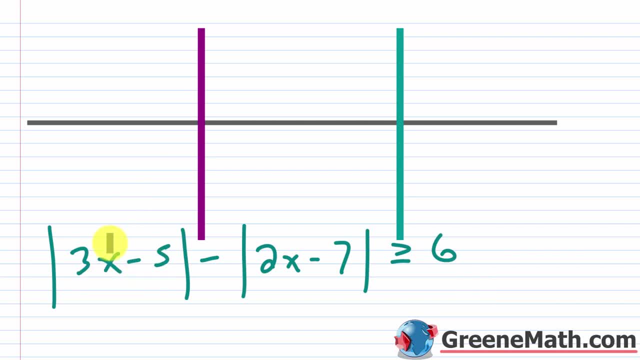 So, again coming to our table, we just want to think about where 3x minus five is equal to zero and where 2x minus seven is equal to zero. So we'll say 3x minus five is equal to zero. 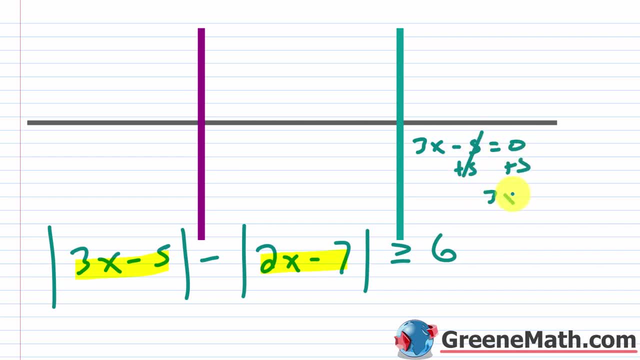 we'll add five to both sides of the equation. we'll cancel that and say 3x is equal to five. And then we'll divide both sides of the equation by three, So we get x is equal to five thirds. let me get rid of this. And then the other guy. we have 2x minus seven, So we'll say 2x minus seven. 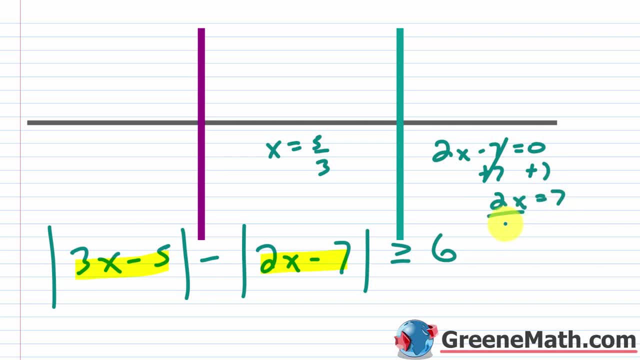 to both sides and cancel this, we get 2x is equal to seven. divide both sides by two, this cancels, and we get x is equal to seven halves. Okay, so if we think about five divided by three, that's basically one and two thirds, And if I think about seven halves, that's 3.5. 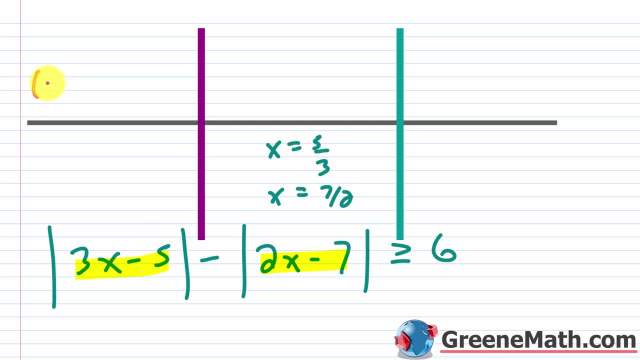 So five thirds is the smaller value. So let's say this first interval is coming from negative infinity, going up to and again excluding the five thirds and make this five a little bit better here. So for the first interval I will include five thirds And I'm going to go up to but exclude 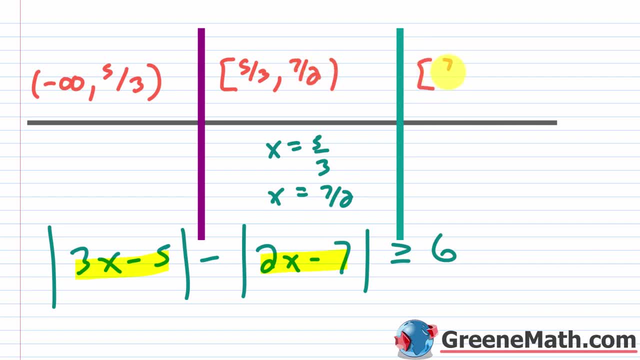 seven halves And then for the final interval, I will include seven halves and I will go out to positive infinity. Alright, so we already know how this works. in the leftmost interval they're both negative, So I'm going to want the negative of the quantity 3x minus five. So I want negative. 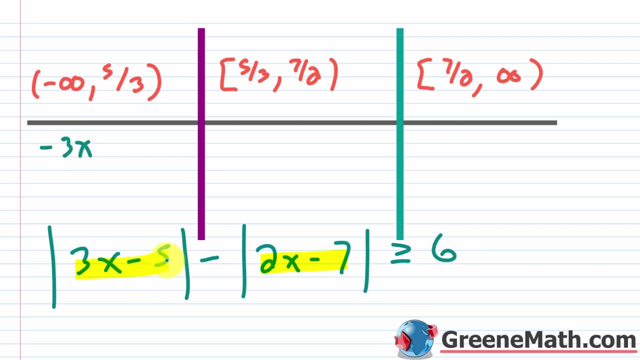 3x, So negative 3x, And then the negative of negative five is plus five. So all I did was distributed a negative to each term here. then this one would also be negative. So let's say this is negative, So this is negative. So I'm going to go ahead and say negative 3x, the negative of two x. 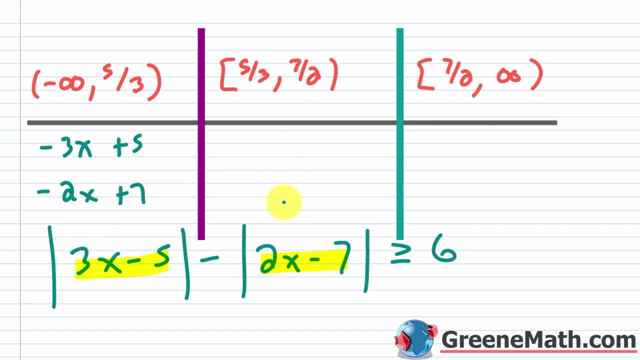 and the negative of negative seven is going to be plus seven. So this first interval is done. Now in the second interval we would say that this guy right here would be non negative, right? If it's five thirds, then it's zero. any other value would make it positive. So you can just drop the absolute. 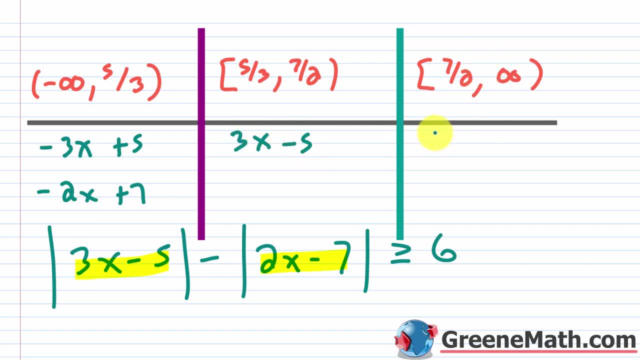 value bars. So this is just three x minus five here In this interval. this guy is positive. So again, just drop the absolute value bar. same rule. So three x minus five Now for this guy. it's still going to be. 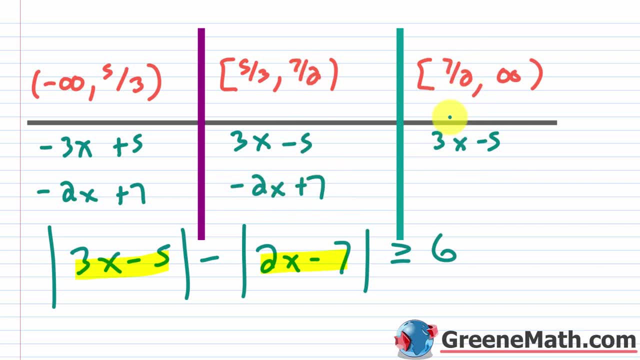 negative in this interval. This is negative two x plus seven. But then once we get here, it's non negative, right? If it's seven halves, then it's zero. anything larger is positive Again. same rule for that, So just drop. 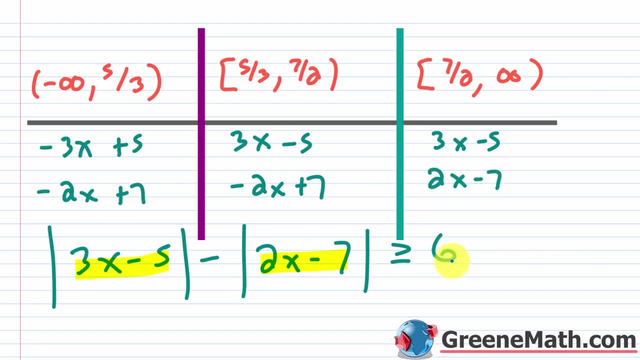 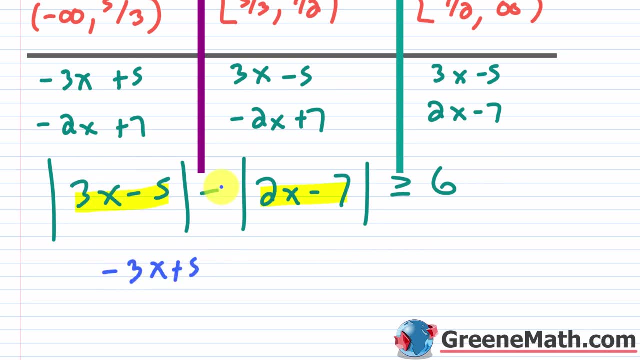 the absolute value bars, it's two x minus seven. All right, let's go ahead and set this up. So in the first interval we're going to have negative three x plus five in the place of this guy. then you have this minus here, And this is where you have to be really careful. You have to wrap whatever. 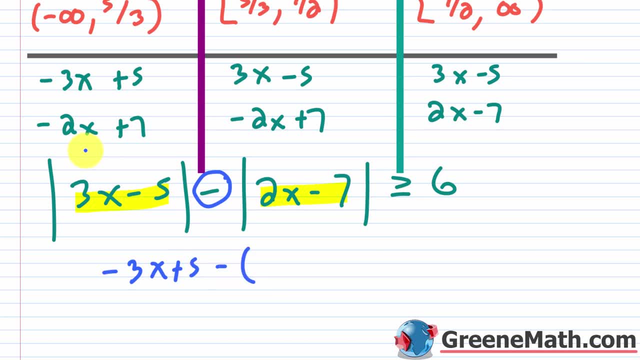 you're going to put here in parentheses. So I'm going to say: minus the quantity, negative two x plus seven, because this whole thing's being subtracted away. then this is greater than or equal to six. At this point I'm just going to say this is negative. three x plus five, the negative gets. 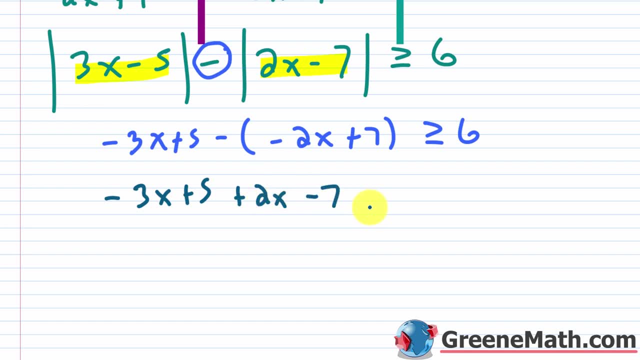 distributed to each, So this is plus two x and then minus seven. this is greater than or equal to six. So if you have negative three x plus two x, that's going to be negative x, And then five minus seven is going to be negative two, And again this is greater than or equal to six. Let's 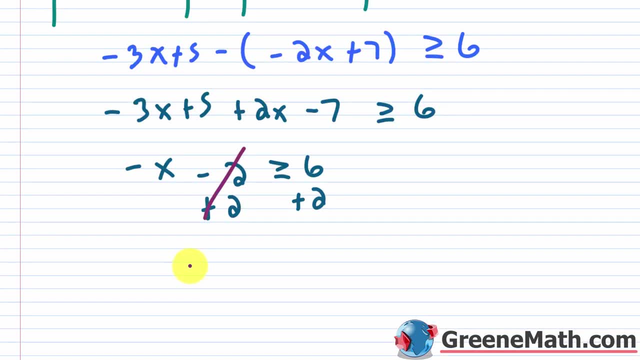 add two to both sides of the inequality. Let's cancel this away. we'll say: negative x is greater than or equal to six. So this is negative zero x plus nine degrees, which is life equal to one dot times negative zero x plus one. Alright, now let's do the last one. I'm gonna do so at each type of 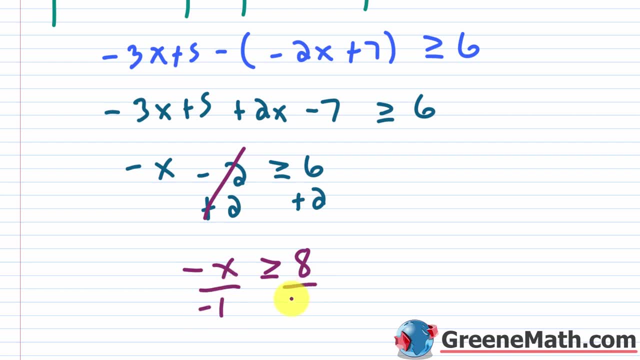 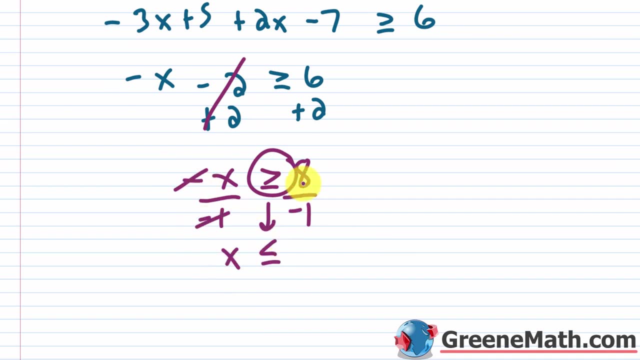 Six plus two is going to be eight. If we divide both sides by negative one, remember to flip the direction of the inequality symbol here. This would give us this: cancels X is less than or equal to eight. divided by negative one is going to be negative eight. 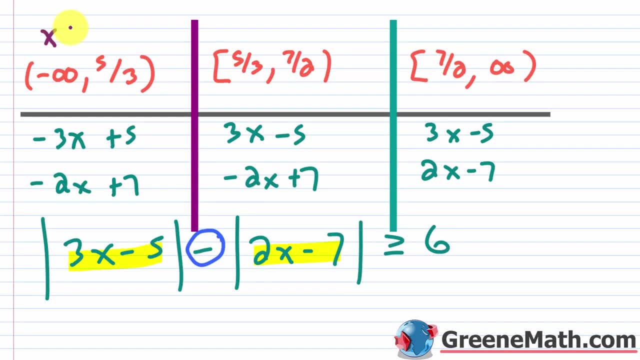 So X is less than or equal to negative eight. So coming back up here we have: X is less than or equal to negative eight, And does that fit in this interval? Yes, it does, So we can take this solution. Okay, for the next one, we're in this interval here. 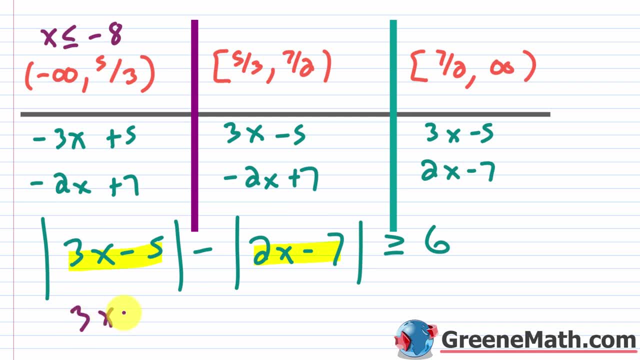 So let's think about dropping this and saying we have three X minus five, then minus. You have to be really careful with this minus sign. again, You're going to take this and put it in this place. So this would be the quantity negative: two X plus seven. 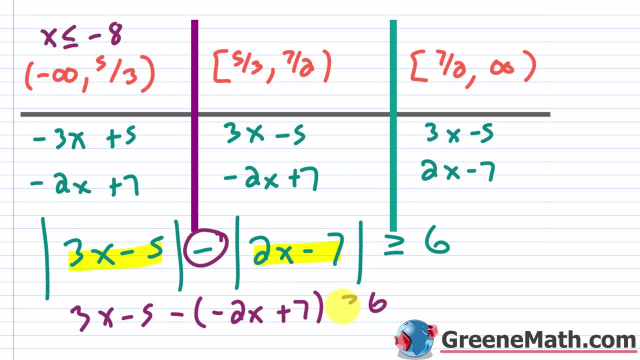 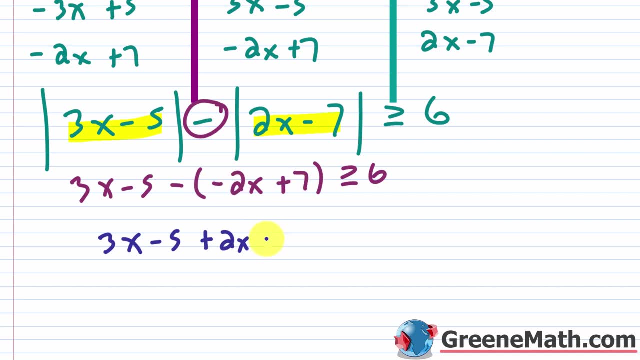 And this is greater than or equal to six. Let me make this a little bit better here. So we have three X minus five, and then the negative of negative two X is plus two X, And then the negative of seven is just minus seven. 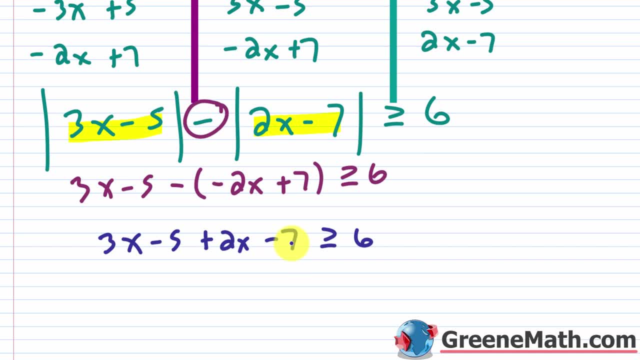 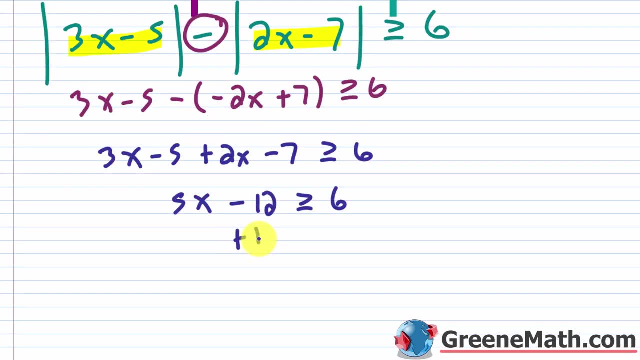 This is greater than or equal to six. So negative five minus seven is negative 12, and three X plus two X would be five. So this is five. X minus 12 is greater than or equal to six. Let's add 12 to both sides of the inequality. 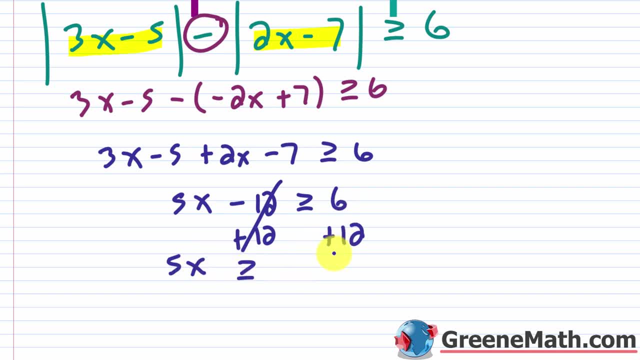 This cancels, You get five. X is greater than or equal to six plus 12 is 18.. If we divide both sides of the inequality by five, this cancels and you're going to have that X is greater than or equal to 18. fifths, 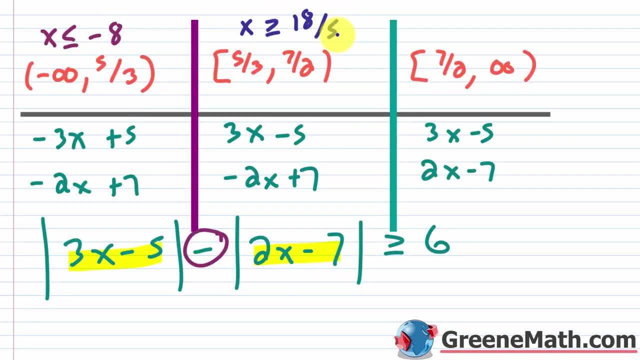 Okay, so let's write: X is greater than or equal to 18 fifths. Now does this work? Well, actually, no, it's not going to be in this interval. You can cross it out If you divide 18 by five on your calculator. 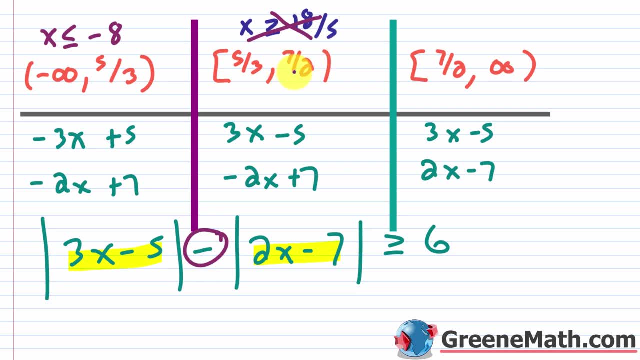 you get 3.6.. And remember, we're thinking about this seven halves. This is 3.5, right? So this value right here is outside of this interval. So you just reject it. Okay, let's look at this interval here. 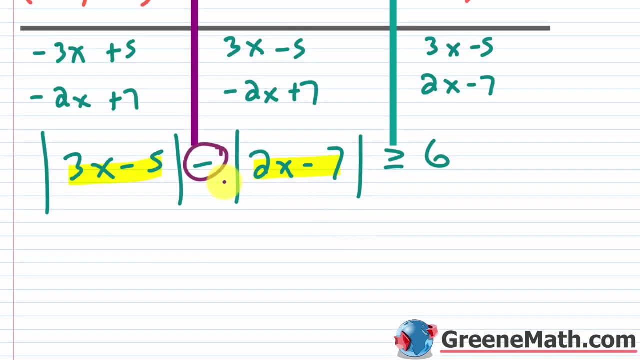 So in this case we could just drop the absolute value bars. but again you have to be really careful with that minus sign. So let's say this is three X minus five, and then minus the quantity two X minus seven, And this is greater than or equal to six. 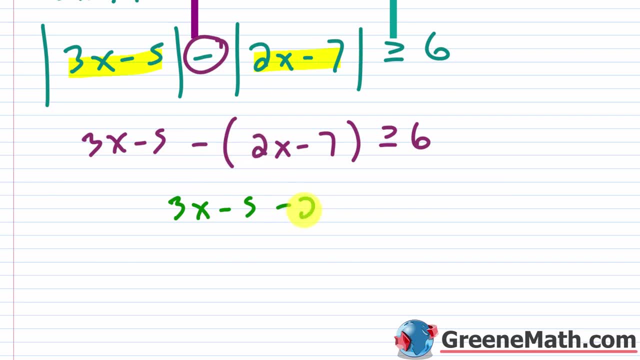 So we'll have three X minus five, and then you'll have minus two X and then plus seven, And this is greater than or equal to six. So here, three X minus two X would be X Negative. five plus seven is going to be two. 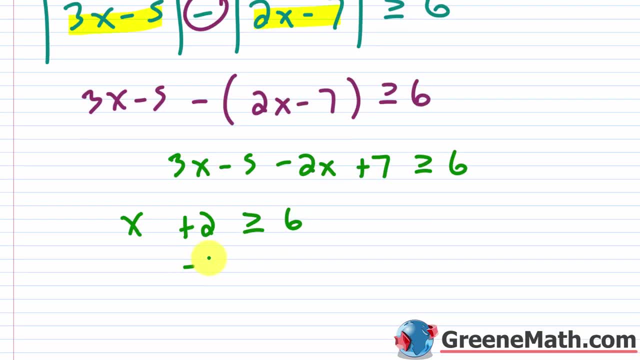 So let's put plus two, This is greater than or equal to six. For this one, let's subtract two away from each side of the inequality. This cancels, and we'll say X is greater than or equal to six minus two is four. 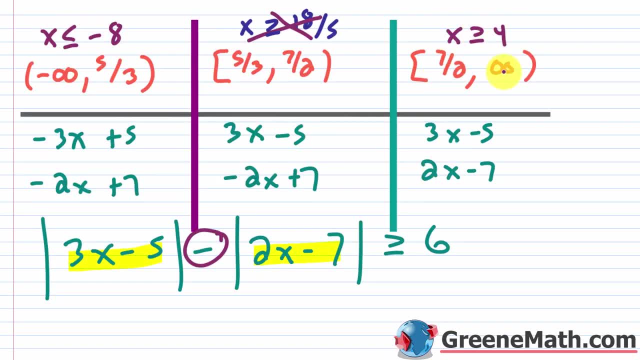 So let's put: X is greater than or equal to four, And this is in my interval right. This starts with 3.5 or seven halves and continues out to positive infinity. So I'll just say X is greater than or equal to four. 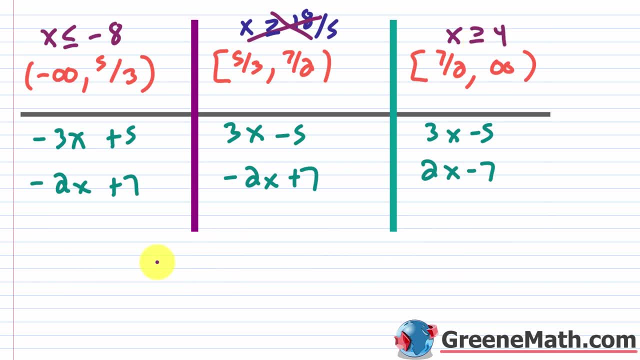 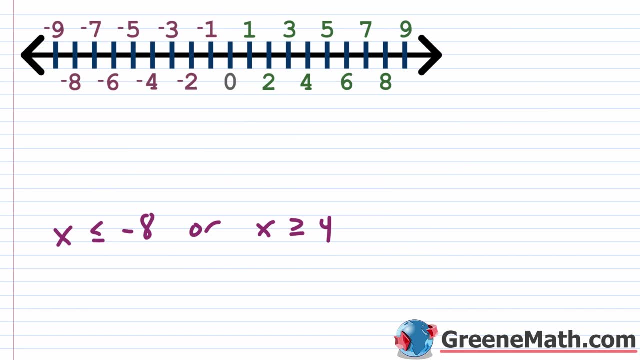 something I can accept. Let me get rid of this and we'll just write our solution. So here it's pretty easy. We just say X is less than or equal to negative eight, or X is greater than or equal to four. Okay, in interval notation. 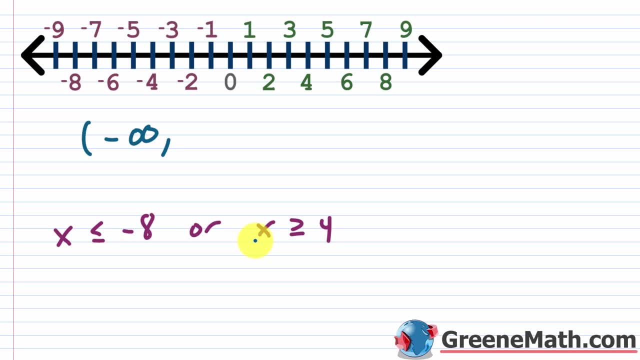 I'm going to say coming from negative infinity going up to and including negative eight. So you want to bracket next to negative eight and then the union with you want to bracket next to four, since it's included and it's going to go out to positive infinity. 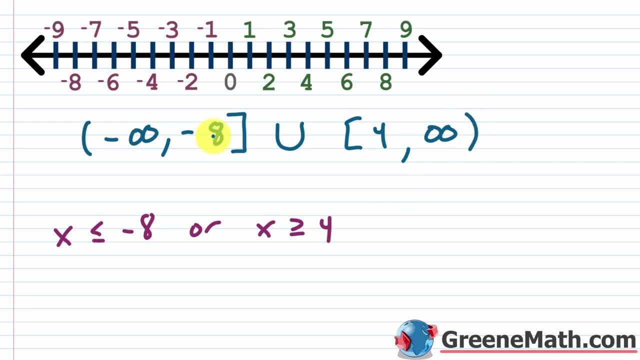 and then just put a parenthesis there. Okay, so at negative eight it's going to be included, So I'm going to put a bracket there. Again, you can use a filled in circle, if that's what your book does. We're going to shade everything to the left. 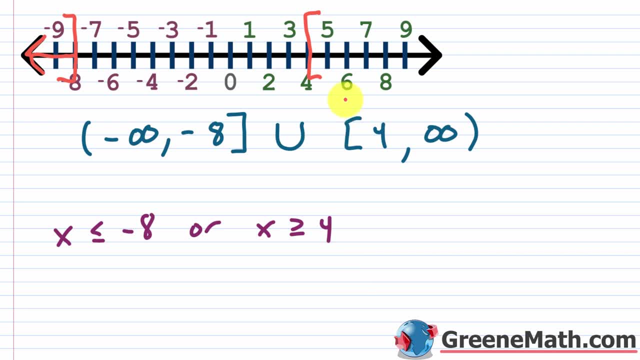 And then at four, we're going to put a bracket there, or, once again, you could use a filled in circle, And then I'm just going to shade everything to the right. So, graphically, X could be negative eight or anything less, or X could be four or anything greater. 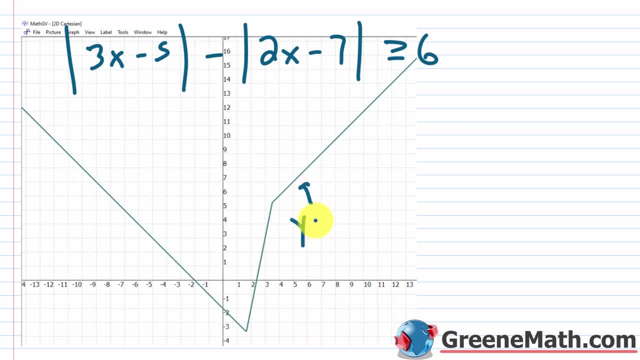 So this graph right here in green, this is, you could say: Y is equal to the absolute value of three X minus five, the absolute value of two X minus seven. So you're trying to see where this guy is greater than or equal to six. 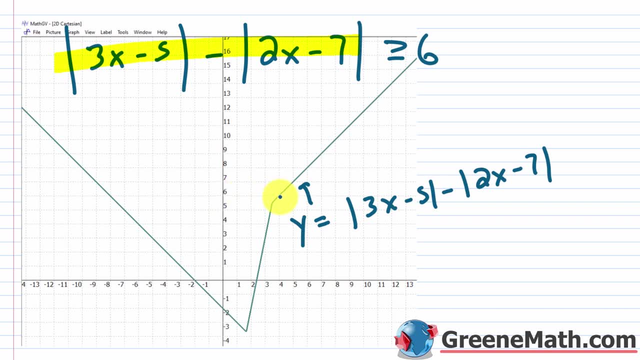 So you're looking for a Y value of six, So that's right here. So you come over. I'm just going to see where it intersects. So that's going to be right here. That's an X value of four, And also going over here. 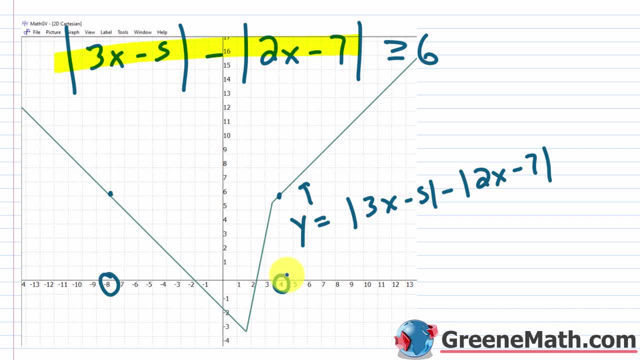 that's going to be an X value of negative eight, right, And that's what we found. So, basically, at negative eight or at four, it's going to be equal to six And then anything to the right of four in terms of the X values. 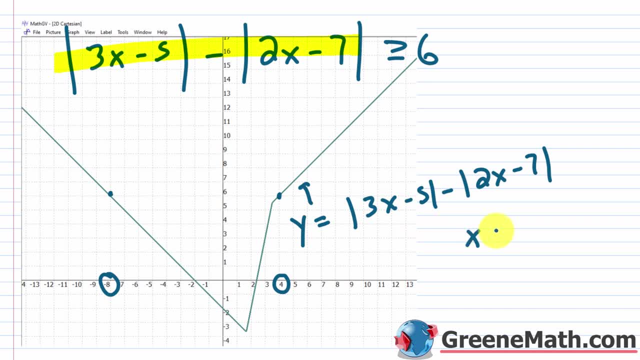 you can see that you're going to be above six. So you could say X is greater than or equal to four. That's that part, And then let me put or. here The other part is again: if you're at negative eight or anything less. 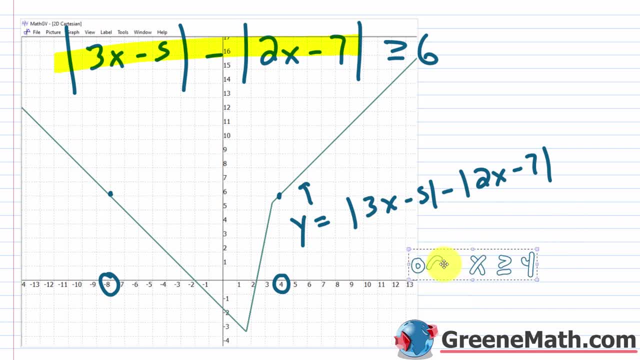 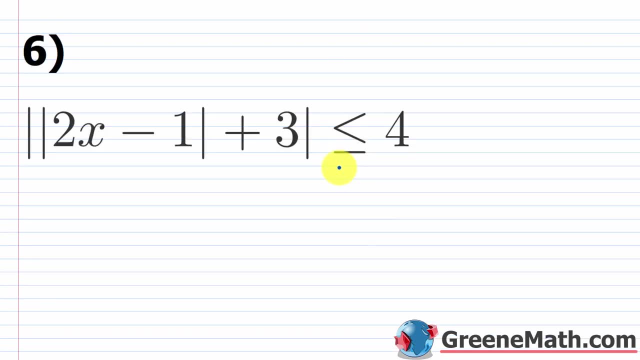 you're going to be above six, So let me actually slide this down just a little bit. I'll say also that X is less than or equal to negative eight. So again, that's how you could get your solution graphically. All right, let's take a look at problem number six now. 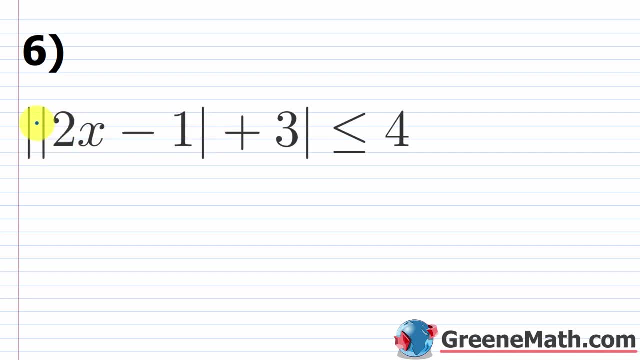 So here we have a problem with nested absolute value. So we have the absolute value of, and then the absolute value of, two X minus one, then plus three. This is going to be less than or equal to four. All right, so this one is a bit tricky. 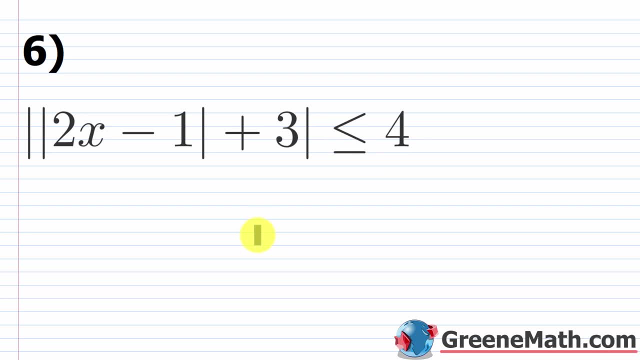 and we didn't do a problem like this in our lesson. but remember, in the previous section we talked about how to solve an absolute value equation of this type, So we're just going to extend that now to working with an inequality of this type. 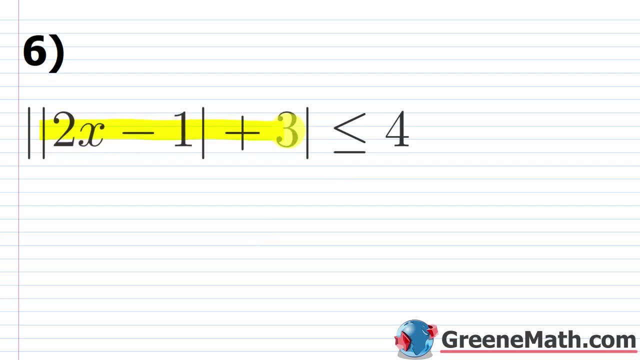 And the idea here is to first think about this guy right here. So I'm just going to say that that's some algebraic expression U. And if I had the absolute value of some algebraic expression U and if it was less than or equal to, 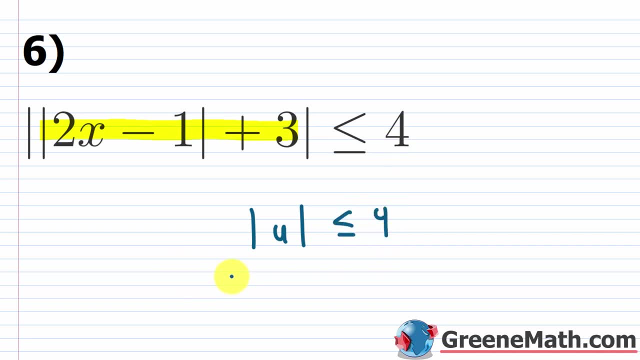 some positive number four. Well, we know this sets up to say that U is greater than or equal to negative four and it's less than or equal to positive four. So okay, we just have to translate that here. So this is my U here. 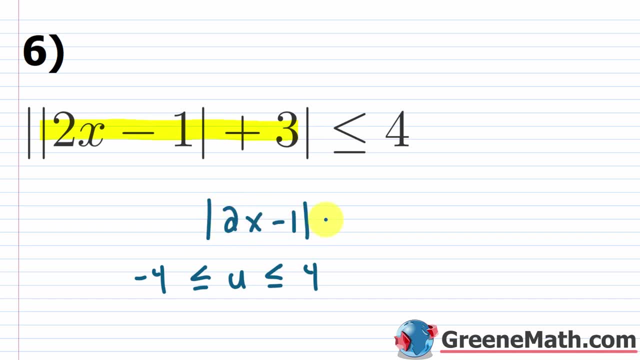 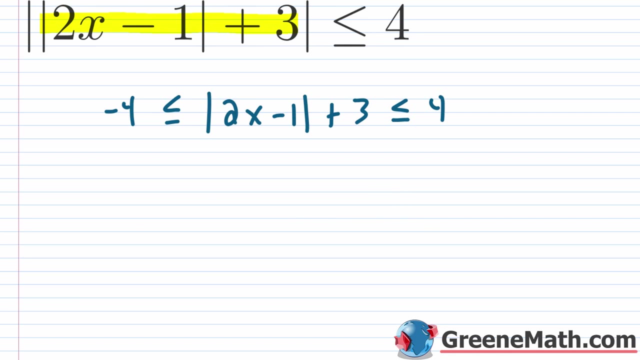 So I would say the absolute value of two X minus one, then plus three, is going to be greater than or equal to negative four and less than or equal to positive four. So this is going to be my setup. now, Because this is a three-part inequality, you can first subtract 3 away from each part. 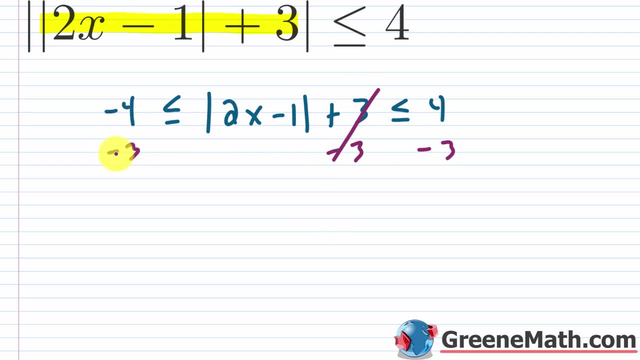 So remember you have to do it to each part. I'm going to cancel that. Negative 4 minus 3 is negative 7.. And we'll say this is less than or equal to. This is the absolute value of 2x minus 1, which is less than or equal to. 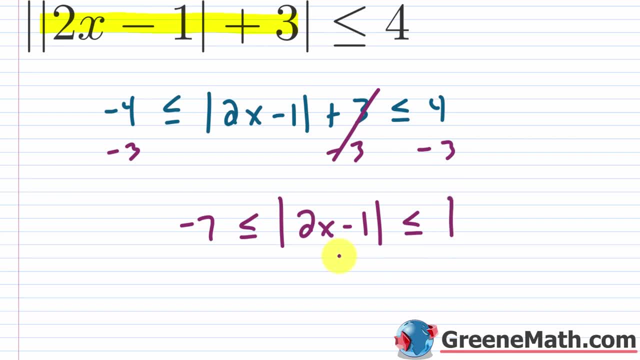 4 minus 3 is going to be 1.. Now you're going to break this up. Remember, when you have a three-part inequality, this is something you can write using the keyword AND, And so things have to work in both when you have the keyword AND. 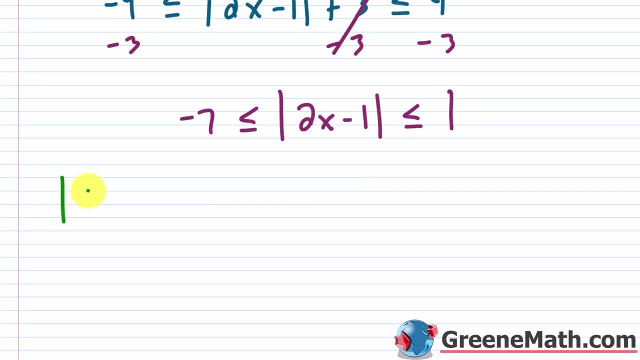 The first one here is going to be really simple. We have the absolute value of 2x minus 1.. And then we're saying this is greater than or equal to negative 7.. So it's greater than or equal to negative 7.. 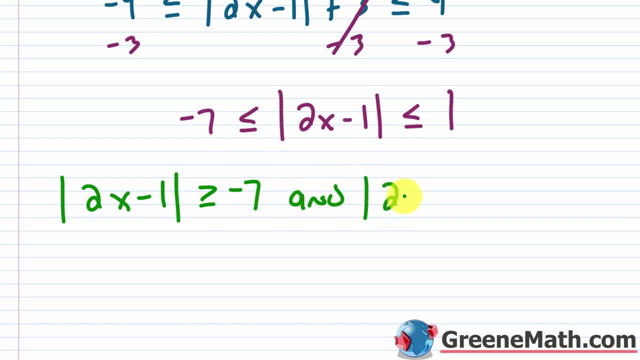 Then I'm going to say: AND We're going to say the absolute value of 2x minus 1.. This is less than or equal to 1.. Now this one right here: I think you can eyeball that and see that it's going to work. 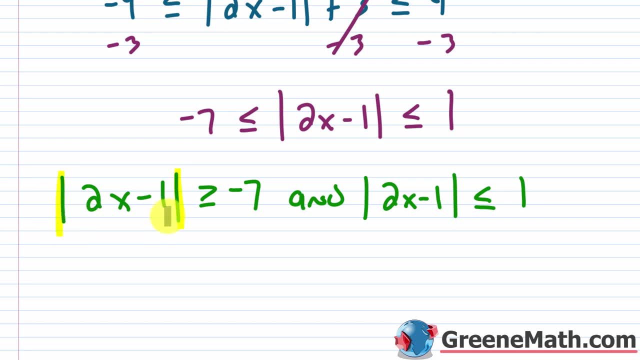 for all real numbers. OK, Because the absolute value operation is always going to give you something that is 0 or positive, so basically non-negative, And so that is always going to be greater than some negative 7.. So this guy right here is all real numbers. 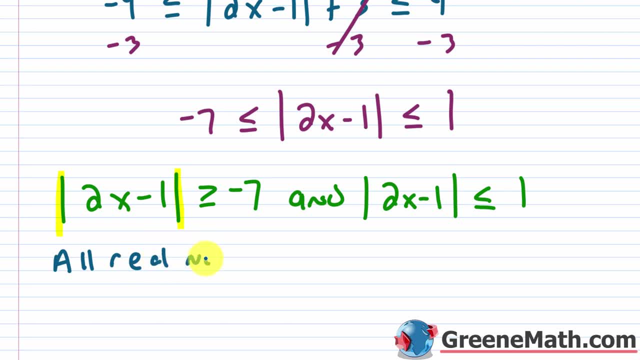 Let me just write this: So all real numbers. So then we have this keyword AND: OK. so basically, because this is all real numbers and there's an AND here, I'm just going to take the solution from this one as the solution for the problem, because it has 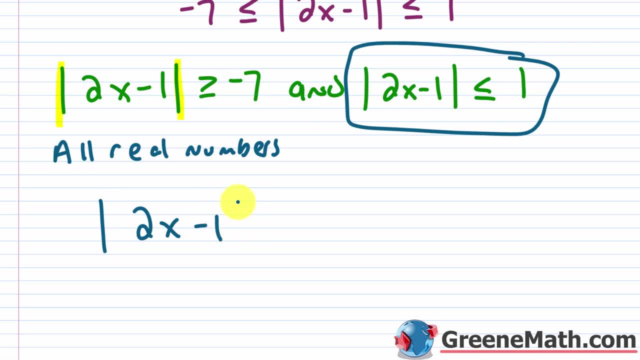 to work in both, We have the absolute value of 2x minus 1.. And this is less than or equal to 1.. So this is going to split up into 2x. So 2x minus 1 is greater than or equal to negative 1, and we'll say: AND, less than or. 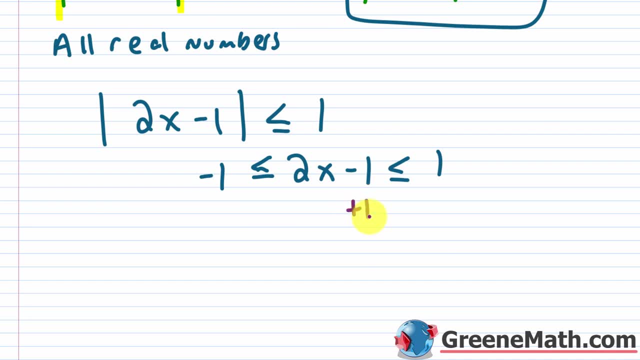 equal to positive 1.. So this is pretty quick to solve. We're just going to add 1 to each part here. So basically, this cancels and you get 0 is less than or equal to, This is going to cancel. 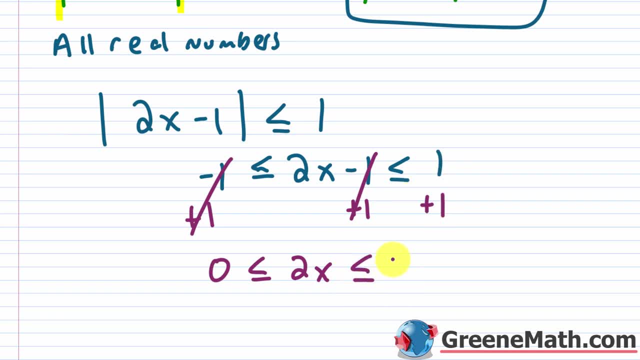 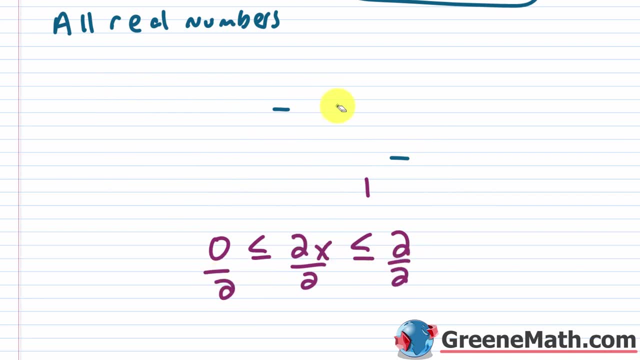 You get 2x, and this is less than or equal to 1 plus 1 is going to be 2.. Now here you can divide each part by 2.. And basically, let me actually just erase this. We don't need this information anymore. 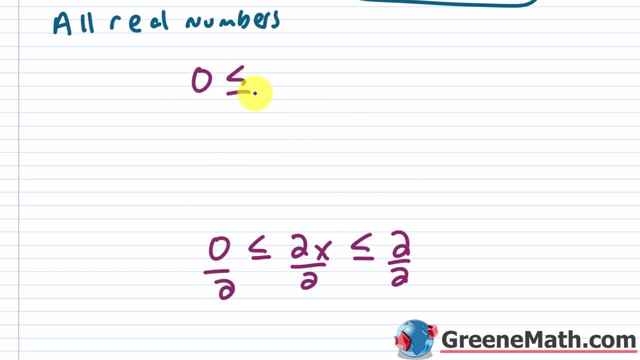 We'll say: 0 divided by 2 is 0, and this is less than or equal to. We have 2 over 2,, which is 1.. So this is x, which is less than or equal to. 2 over 2 is 1.. 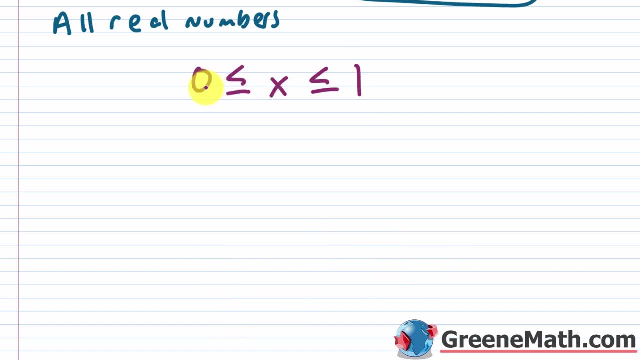 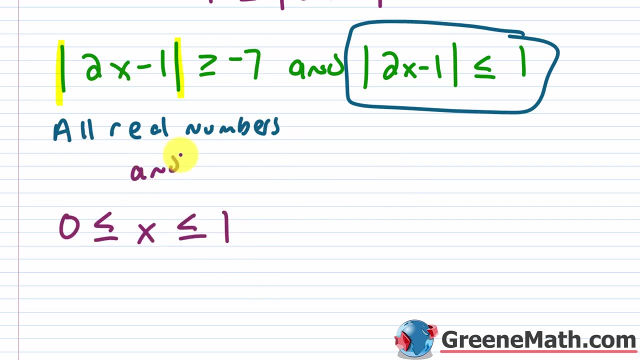 So this tells me that x is going to be anything that's greater than or equal to 0 and less than or equal to 1.. So basically you would write this like this: So you say all real numbers from this one, Then you say: AND you have x is greater than or equal to 0 and less than or equal to 1. 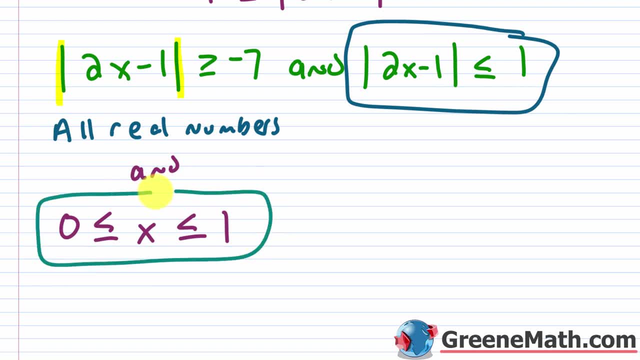 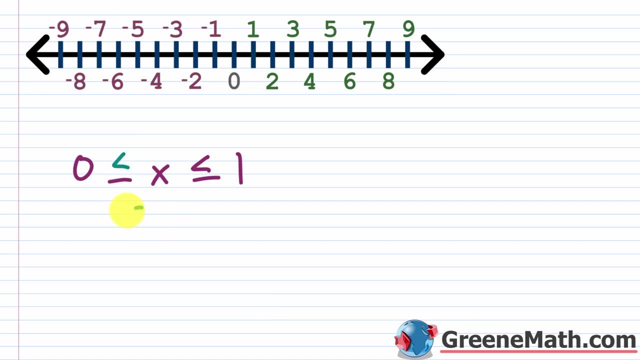 from this one Again, because you're using the keyboard AND you have to use this one as your solution because it has to work in both. Okay, So here let me make this a little bit better. We would say in interval notation. so basically, 0 is included up to and including 1.. 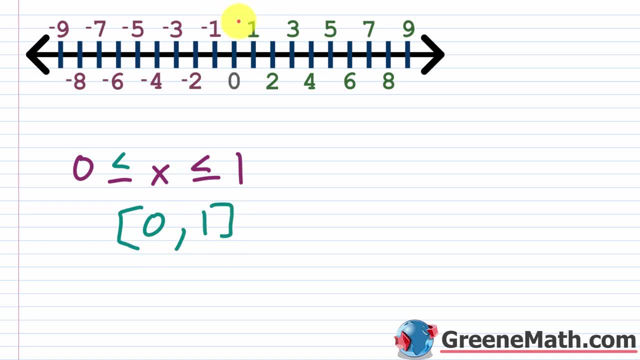 So you have a bracket next to each, And then this is going to be kind of tight to fit this here, But basically you want a bracket at 0 and a bracket at 1.. Again, you can always use a filled-in circle if that's what your book does. 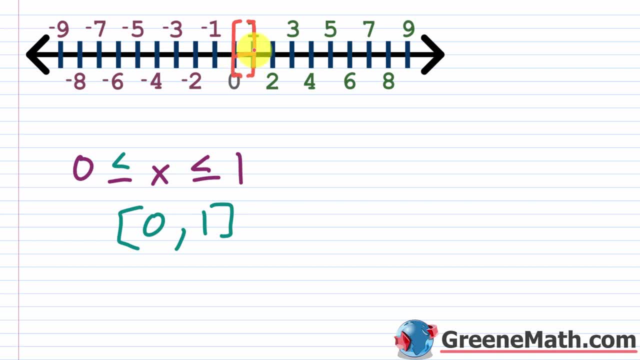 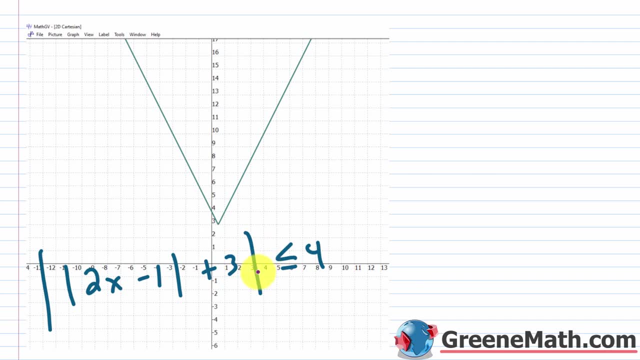 And then just shade everything in between. So x can be 0 or anything going up to and including 1.. So graphically, a lot of programs won't actually do this or you'll get trouble with it. But I've sketched a little graph here. 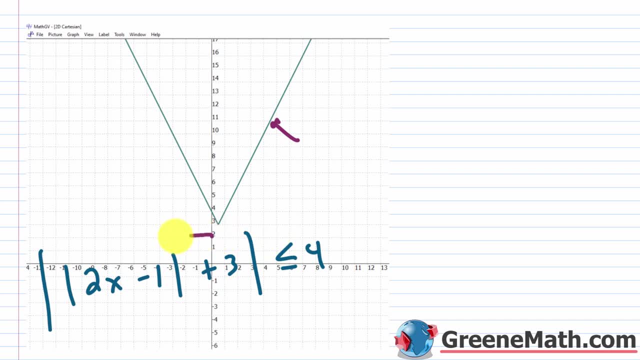 You can think about it. So this part right here is just this guy right here, Right, If you punch that in, you could even say that y is equal to the absolute value, of the absolute value of 2x minus 1.. And then basically you have plus 3.. 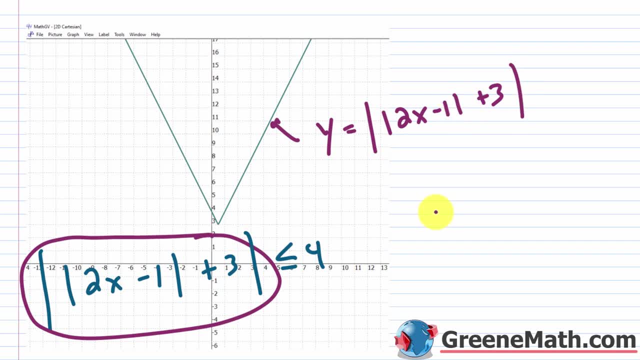 And maybe we'll make this a little bit shorter here- And then, essentially, you're saying: where is this less than or equal to 4?? Well, again, look at the y values. Here's 4.. Right, So let me actually get rid of this. 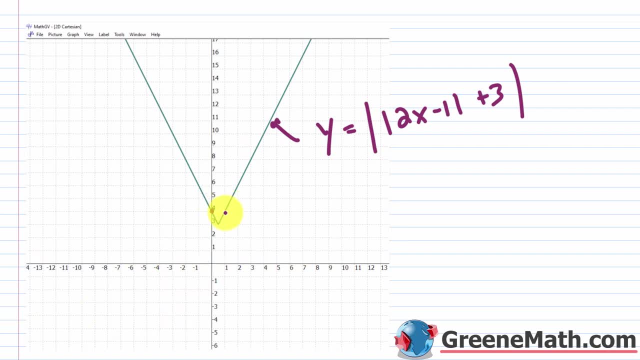 I think it's in the way here. So here's 4.. And this is where it crosses. And this is where it crosses In terms of having a y value of 4.. So come down here. This is an x value of 0.. 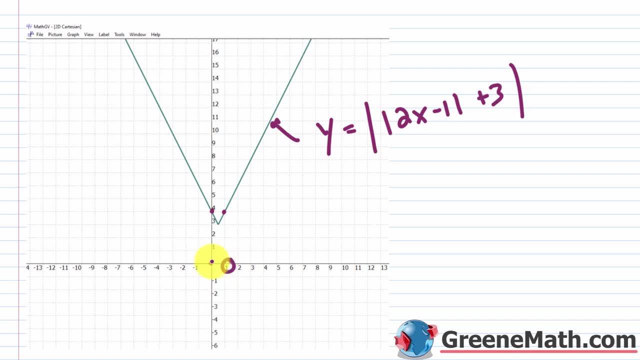 And this is an x value of 1.. So you can see that if you're between 0 and 1, the y value is going to be less than 4.. If you're at an x value of 0, or you're at an x value of 1, the y value is 4.. 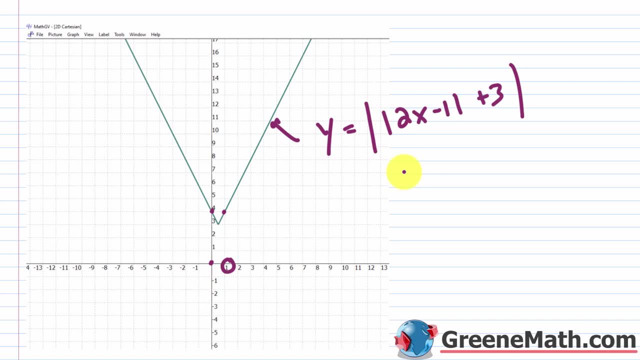 OK. So basically our solution: if you're saying, where is this guy? less than or equal to 4, it's x is greater than or equal to 0.. OK, So starting here, And then less than or equal to 1.. 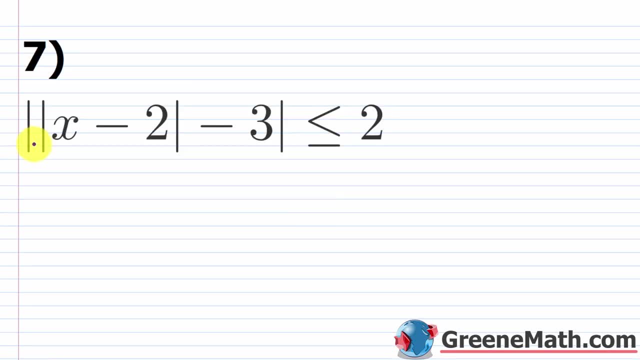 So ending here. All right, We're at number 7 now. So here we have the absolute value of the absolute value of x minus 2, then minus 3.. This is less than or equal to 2.. So again, another nested absolute value problem. 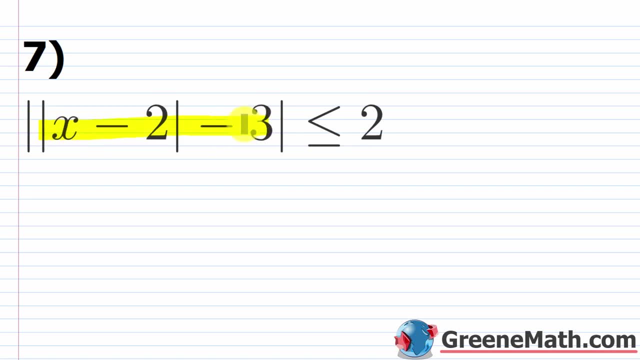 So just think about this guy right here. the expression inside of the outer absolute value bars Again. you can just think about that as being u. So if the absolute value of u is less than or equal to 2, then u is greater than or equal. 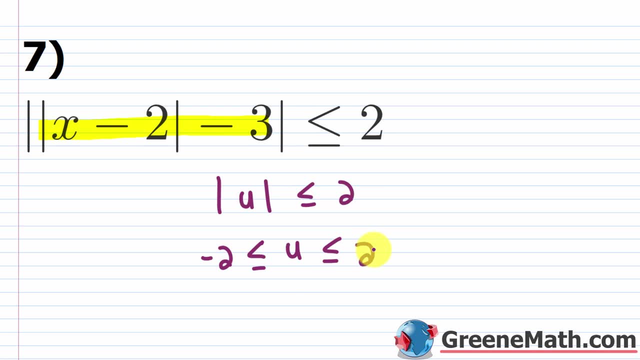 to negative 2 and less than or equal to positive 2.. So let's just write this out. So we would have the absolute value of x minus 2, then minus 3.. And this is going to be greater than or equal to negative 2 and less than or equal to 2.. 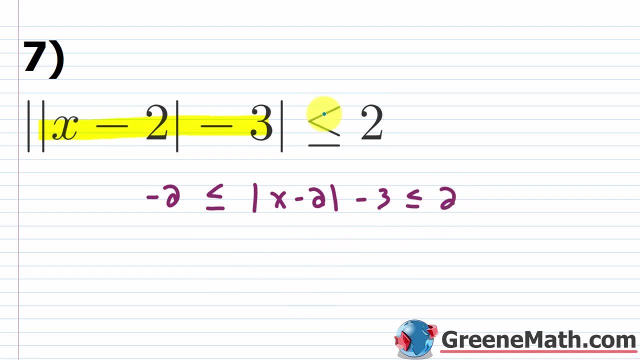 OK, So let's work on this now. So this is a three-part inequality. at this point We're going to end up splitting it, But for right now, let me add 3 to each part to make this a little bit easier to work with. 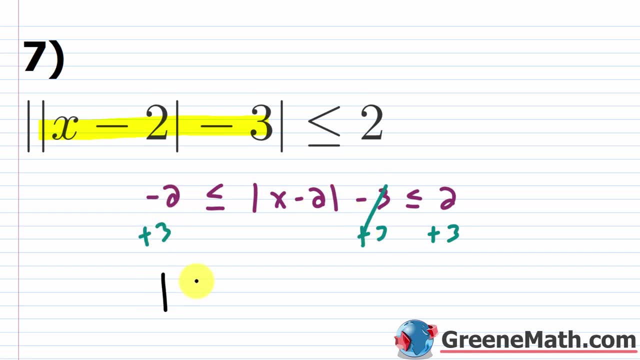 This will cancel. We'll have negative 2 plus 3, which is 1.. And this is less than or equal to, the absolute value of x minus 2.. And then this is less than or equal to 2 plus 3 is going to be 5.. 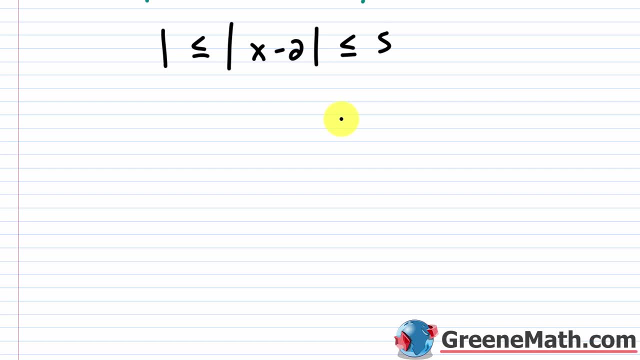 OK. So what I'm going to do now is split this up using my keyword AND. So I'm going to say that the absolute value of x minus 2 is greater than or equal to 1.. Then I'm going to say: AND the absolute value of x minus 2 is less than or equal to 5.. 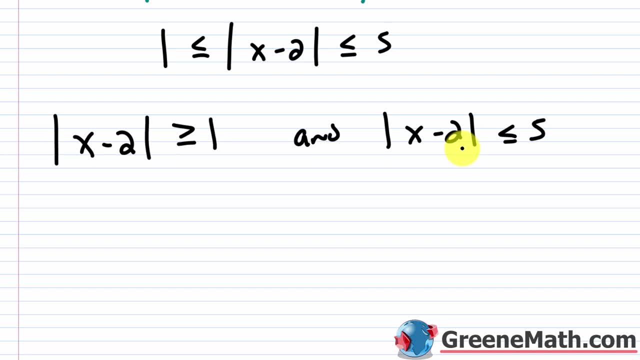 So this is more challenging, or I would actually say more tedious, than the last problem, Because in the last problem we had something with a solution of all real numbers, So we really only had to take the solution from the problem on the right. 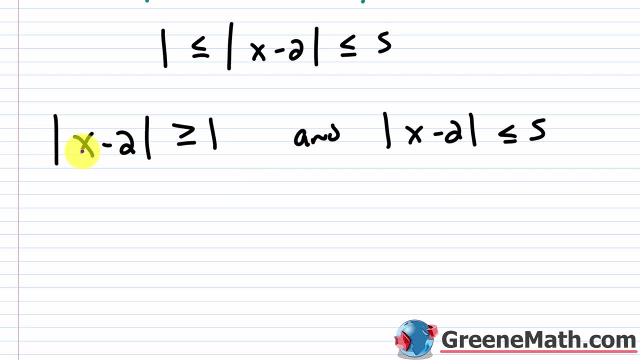 But here we're going to see that we have to do some combining. So on the left, if you have the absolute value of x minus 2 and it's greater than or equal to 1, you would say that x minus 2 is less than or equal to negative 1, or x minus 2. 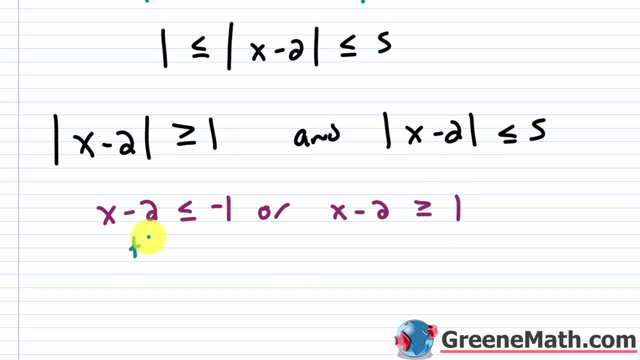 is greater than or equal to positive 1.. So for this one, let's add 2 to each side. This would cancel. You get x is less than or equal to. if you have negative 1 plus 2, that's just going. 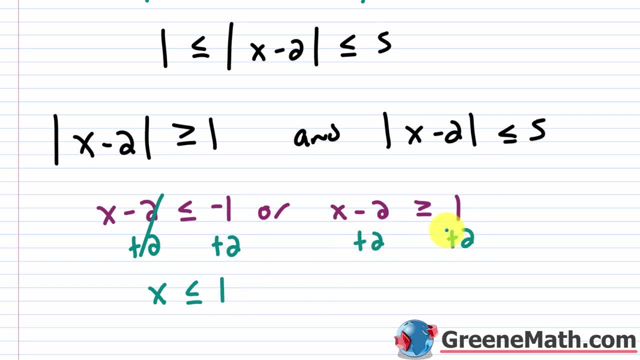 to be 1.. And then over here let's add 2 to each side. This will cancel And you're going to get negative 1 plus 2.. And you're going to get: or x is greater than or equal to 1 plus 2 is 3.. 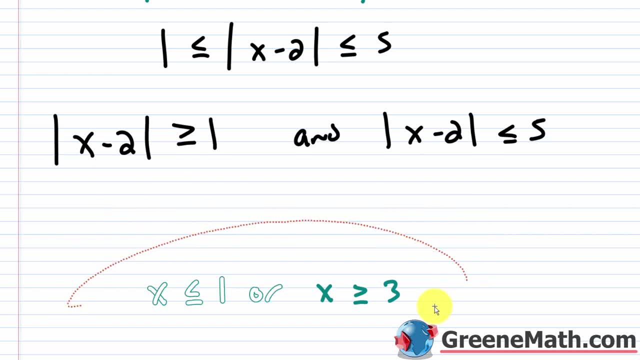 So that's for this one right here. Let me scooch this up here so we can keep this more organized. So you have: x is less than or equal to 1, or x is greater than or equal to 3.. OK, But you've got this keyword AND. 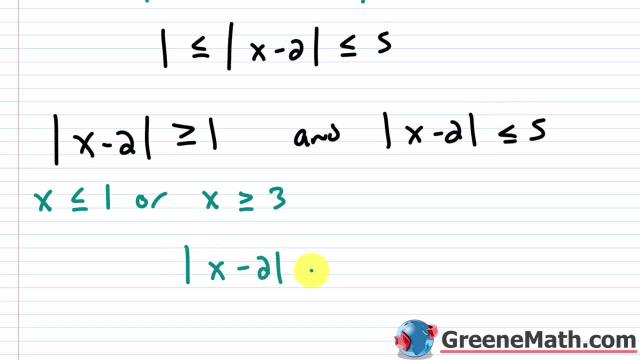 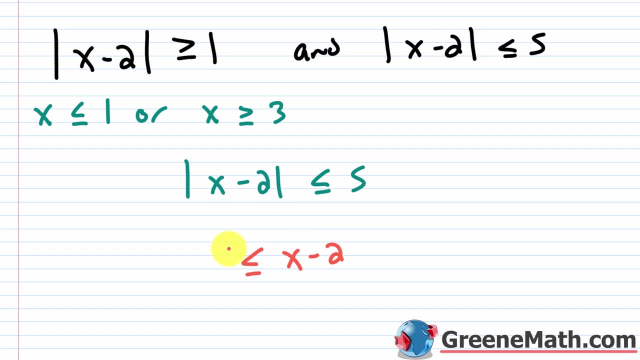 So let's work on this. You have the absolute value of x minus 2, and this is less than or equal to 5.. So this one has the setup where we say x minus 2 is greater than or equal to the negative of 5.. 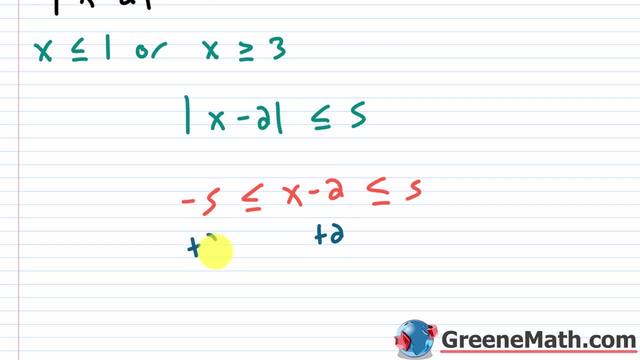 Less than or equal to 5.. Let's add 2 to each part here And cancel this. So let's say negative 5 plus 2 is going to be negative 3, and this is less than or equal to. You'll have your x here. 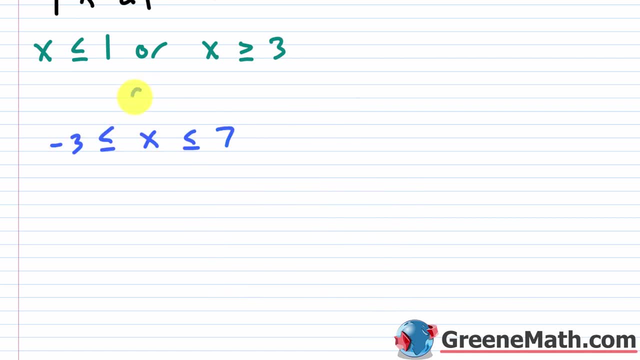 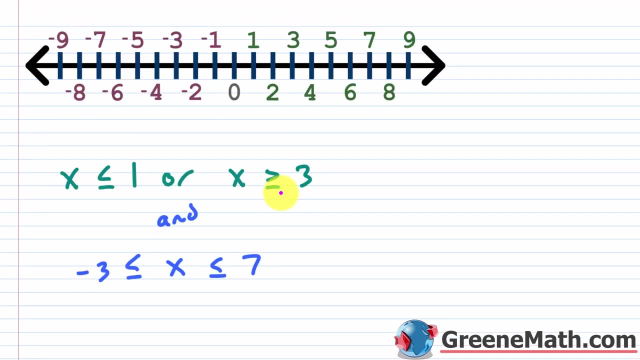 We'll say: which is less than or equal to 5 plus 2 is going to be 7.. And I'm going to put the keyword AND here, and this is going to be a little bit complex to figure out. So let's grab this and let's start with this guy up top. 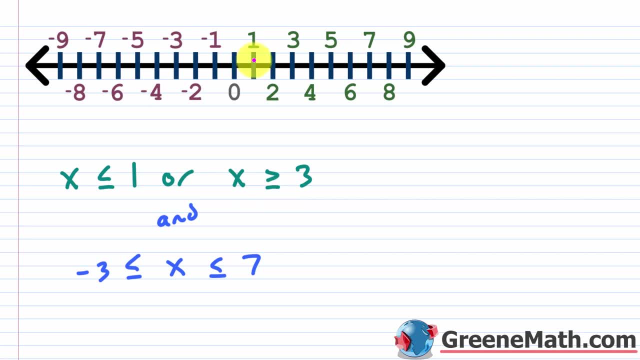 So if you had, x is less than or equal to 1,. I'm going to use a filled in circle here. I normally don't do that. I normally use a bracket. I'm going to do that in this case And I'm going to shade everything to the left here. 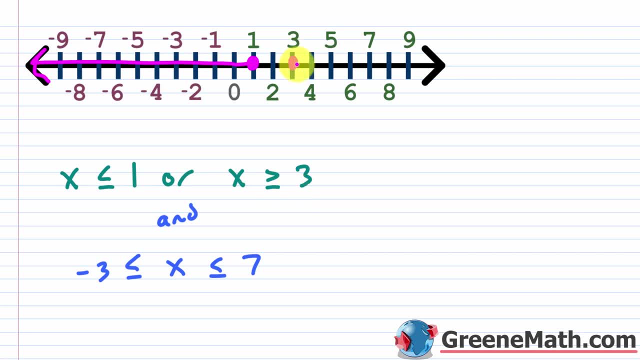 Then x is greater than or equal to 3,. I'm going to come to 3, filled in circle shade, everything to the right. So, thinking about this one we have, x is greater than or equal to negative 3, and less than. 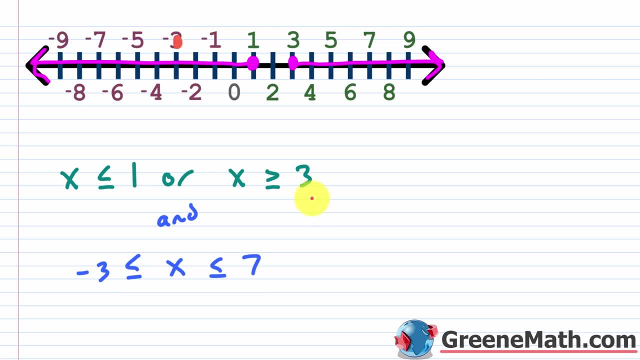 or equal to 7.. So at negative 3 I would put a filled in circle, and at 7 I would put a filled in circle and I would shade everything in between. So now you're thinking about the intersection or the overlap. 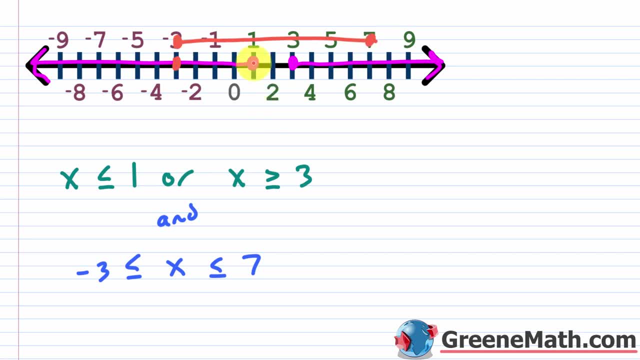 Well, this negative 3 would be included, And this 1 would be included, And then this 3 would be included and this 7 would be included. But basically it's just those areas and let's get rid of this. 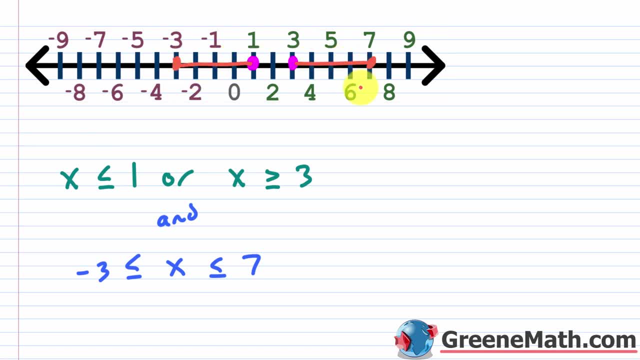 We would shade between here and between here. So let's get rid of this. I think we can see the solution graphically and then put it together. So basically, you would say that x is greater than or equal to negative 3, and less than. 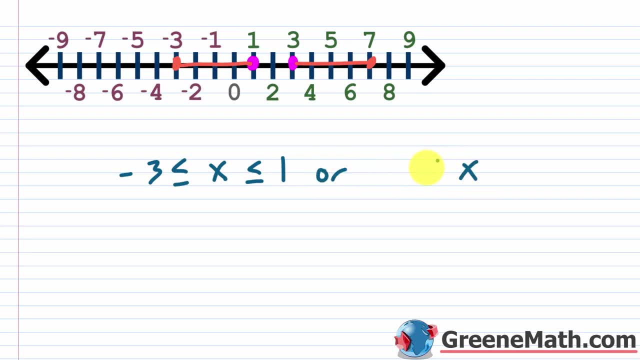 or equal to 1.. Then, or x is greater than or equal to 3, and less than or equal to 7.. So I'm going to put a filled in circle here. I'm going to put a filled in circle here. 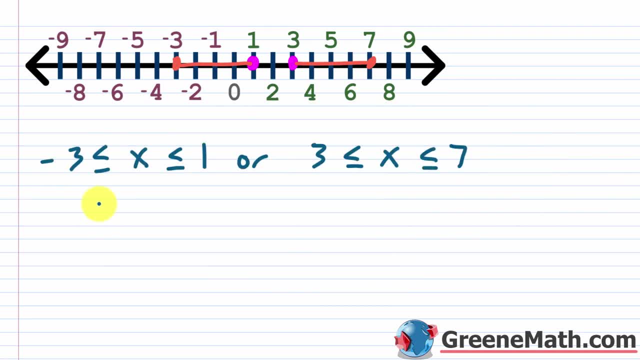 It's going to be greater than or equal to 7.. That's your solution there. And then an interval notation: you're going to put a bracket next to negative 3. This is going up to and including 1, so that you want to bracket there. 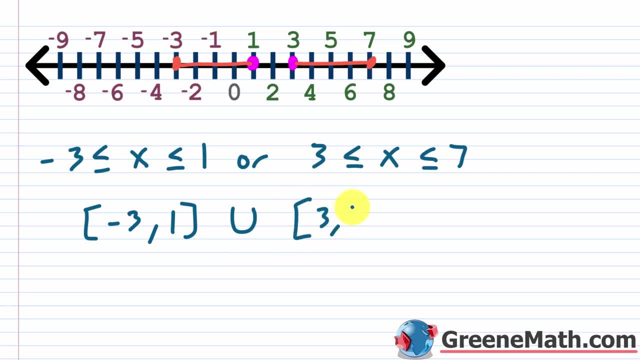 And the union with: again, everything's going to have a bracket. so the 3 and the 7, because they're both included. Ok, so this is your interval notation. Now, I like to use brackets when I graph these guys, so I'm just going to switch this over. 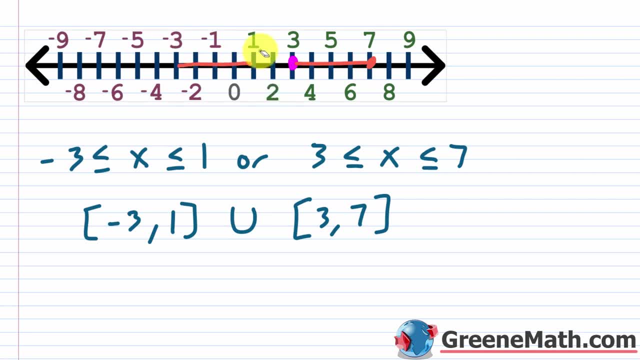 This is a perfectly acceptable way to do this. It's just not the way that I'm used to. So I'm going to put a bracket at negative 3, and put a bracket at 1.. then I'm going to put a bracket at three and a bracket at seven and just shade everything in. 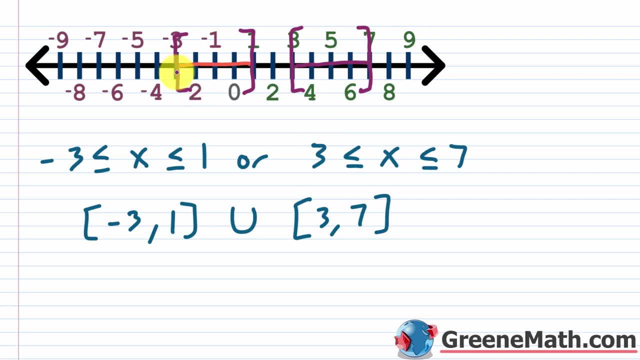 between there. So, graphically, x can be anything starting from negative three going up to and including positive one, or it could be anything starting with three and going up to and including seven. So, once again, thinking about this graphically, you can get rid of this part, right. 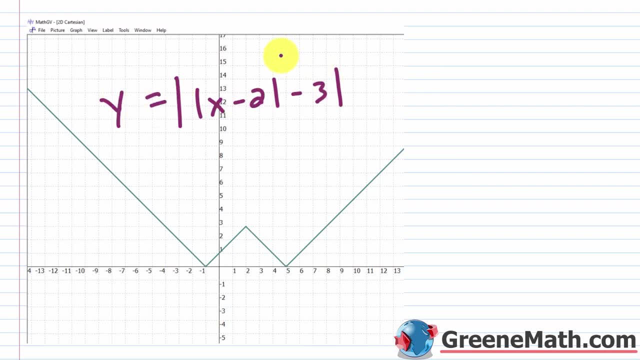 here And I'm just going to say that y is equal to this. this was the left side And so, basically, that's this graph here And you want to see where is it less than or equal to two? So where is the y value two or lower? So we can see that if we go here, this is at negative three, If we go. 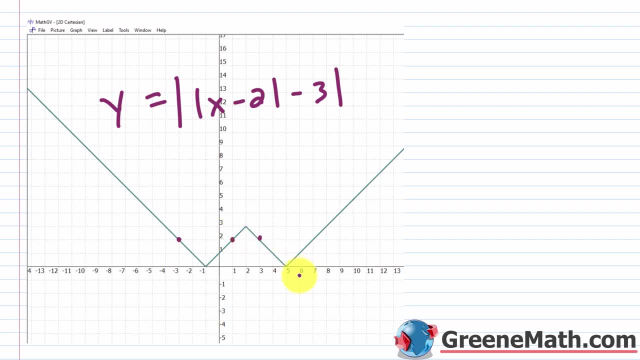 here, this is at positive one. If we go here, this is at positive three, And then, if we go here, it's at positive seven. So you would see that between an x value of negative three and an x value of positive one, the y value is two or less right. So that's this part right here. when you look 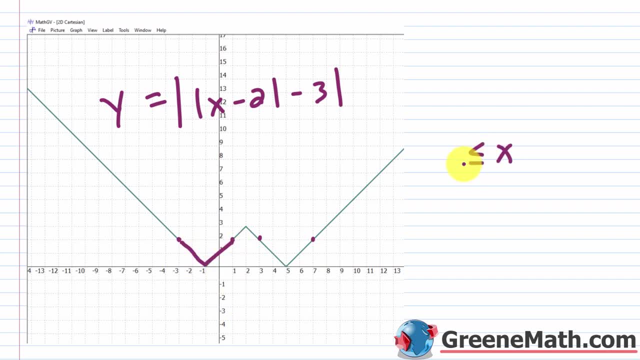 at the graph. Okay, so let me write: x is greater than or equal to this negative three, we'll say- and less than or equal to one. Now, as you move to the right here, between one and three, right, not including. 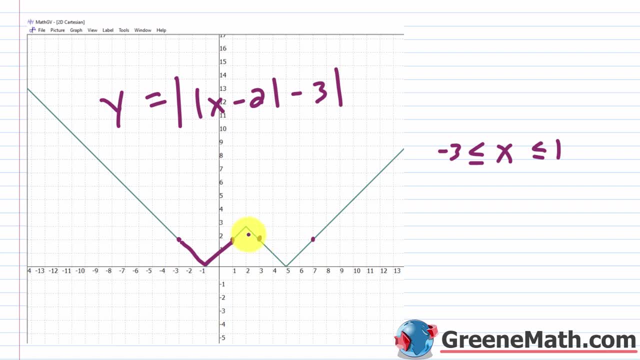 either one, you're going to be above two, But then, when you hit three, you're at two in terms of the y value. And then, as you continue to the right, right, as your x values increase, going up to and including seven, you're going to either be below two or equal to two when you get to seven. 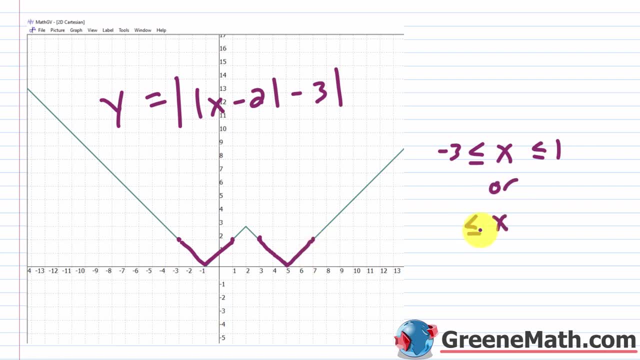 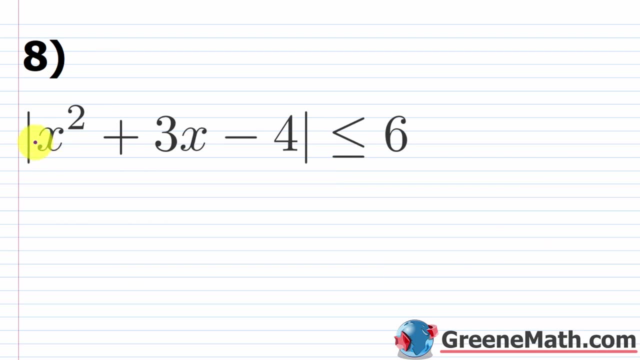 right, So you can say again: or x is greater than or equal to again this three and less than or equal to seven. All right, let's take a look at problem number eight now. So here we have the absolute value of x squared plus three, x minus. 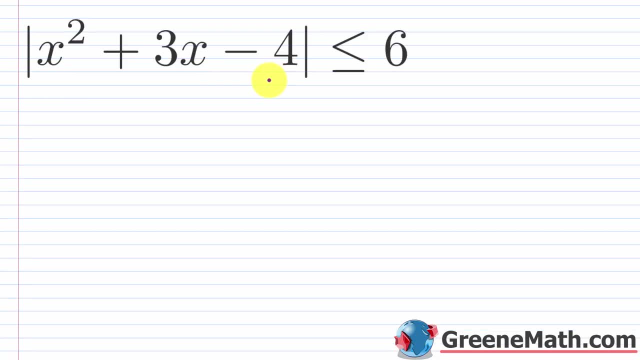 four, And this is less than or equal to six. So again, we didn't do an example of this in the lesson, But we can just use our rule. we say the absolute value of u is less than or equal to six where u is x squared plus three, x minus four. well then u is going to be greater than or equal. 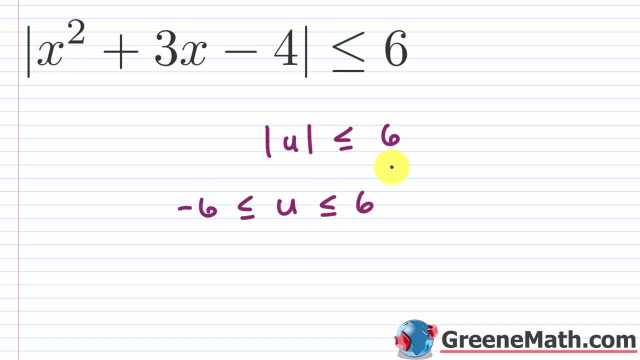 to negative six and less than or equal to six. So just set this up and say that we have x squared plus three, x minus four. that's going to be in the middle. we'll say this is greater than or equal to negative six, and then and less. 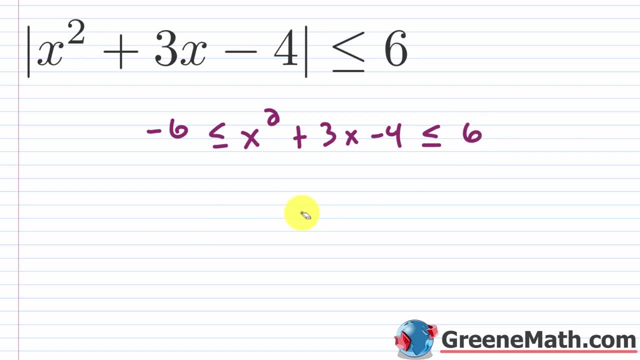 than or equal to six. Okay, what I'm going to do, since this is a three part inequality, I'm just going to add four to each part. I think that's going to make it a little bit easier. So this is going to cancel and you'll have x squared. then, plus three x, we'll say this is greater than. 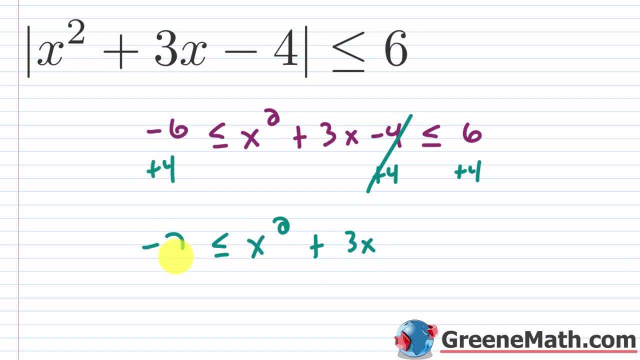 or equal to negative six, And then we're going to add four to each part and then we're going to negative six plus four is going to be negative two, And then, over here, six plus four is going to be 10.. So we'll say: this is less than or equal to 10.. So I'm going to split this up using the. 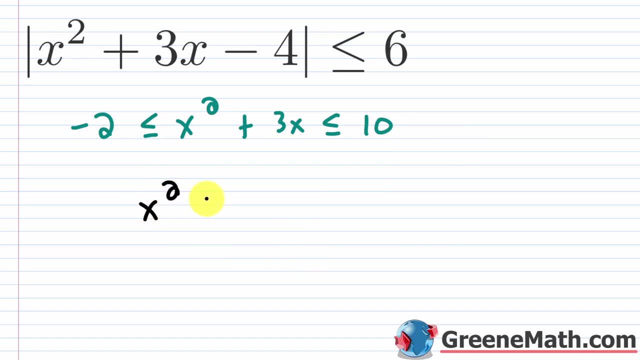 keyword, and So I'm going to first say that x squared plus three x is greater than or equal to negative two. Let me slide this over a little bit. And then I'll say: and we'll say that x squared plus three x is less than or equal to 10.. Let's start out with our guy on the left. 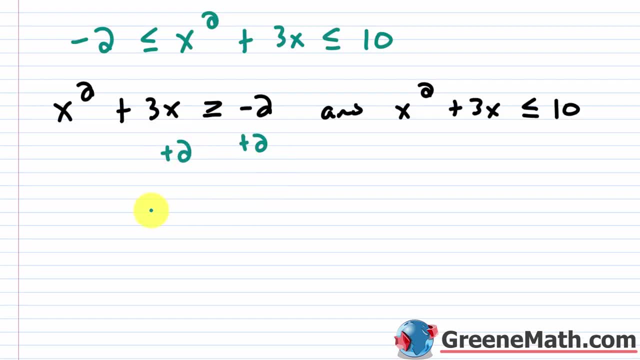 And what I'm going to do is just add two to both sides of the inequality. so this is x squared plus three. x then plus two is greater than or equal to zero. And then for this guy here, I can factor this: if you want two integers whose sum is three, 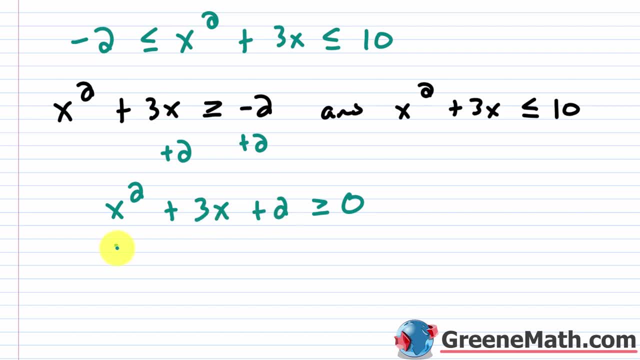 and whose product is positive two. well, that's two and one right. So I can say this is x plus two, that quantity times the quantity x plus one, and this guy would be greater than or equal to zero. we know, if we solve a quadratic inequality, the first thing you do is find the critical values. 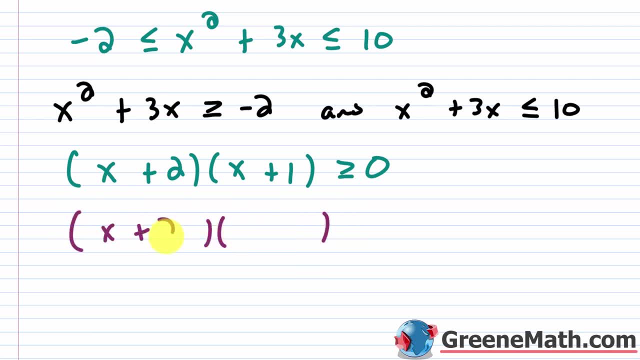 So you can just factor this like this: So x plus two here and then x plus one there, And we'll just say this is equal to zero. So you would say x plus two is equal to zero. you'd solve that. you get x is equal to. 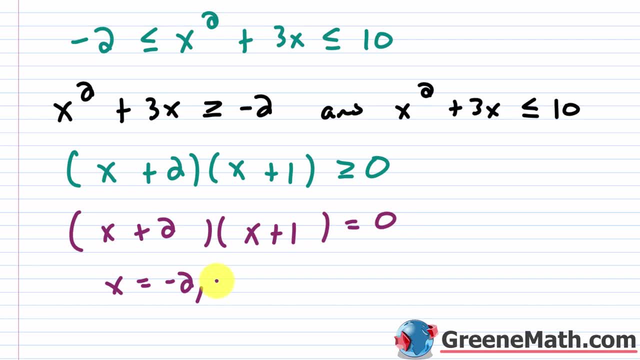 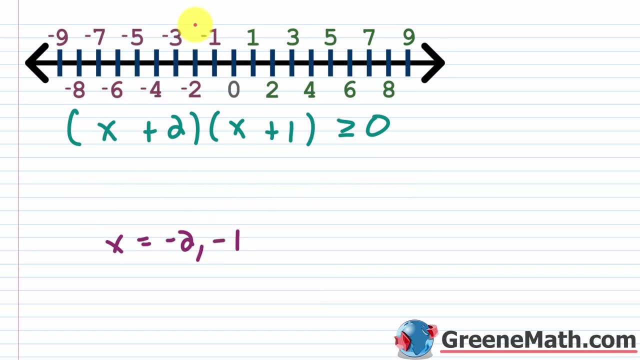 negative two. you would say: x plus one is equal to zero. you solve that. you get x equals negative one. Okay, so let's grab everything you want to come to your number line. you don't need this anymore. So then that's your critical value of negative two. let's put a vertical bar. 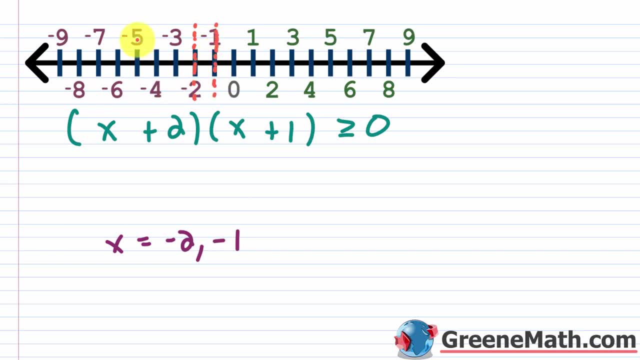 and then also at negative one. So anything less than negative two, let's say that's a- between negative two and negative one, that's b, And anything greater than negative one, that's c. So you have a, b and c. So you're just going to. 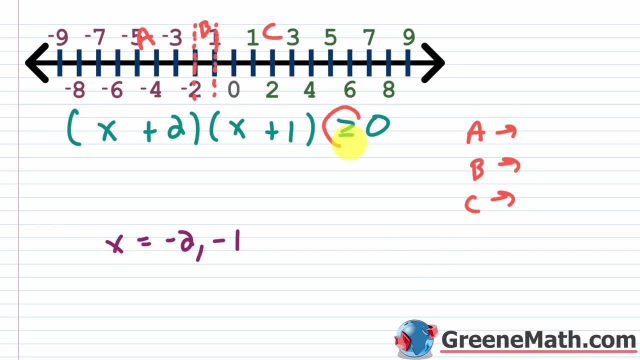 test inside of each. So we know here, because this is non strict, that negative two and negative one would be included. But let's just think about something that's in a. So let's pick negative three. So negative three plus two is going to be negative one, And then negative three plus one. 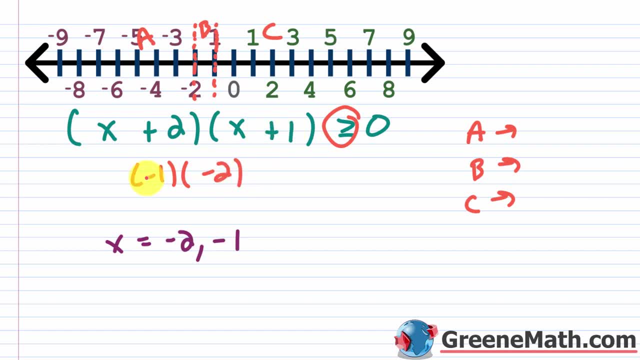 is going to be negative two. The main thing here is that it's a negative times a negative, which is a positive, which is always greater than zero. So this is true. Let's just say that negative one times negative two is two and two is greater than zero. So that's. 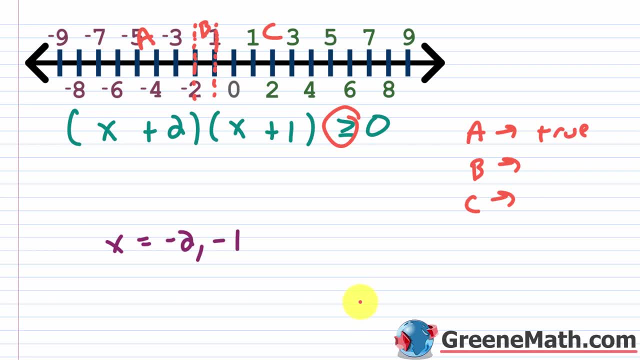 good to go. Okay, so for b we're between negative two and negative one. Now you could use something like negative 1.5.. And again, if you don't want to go through the calculation, just say: is going to be negative or is it going to be positive? Well, negative 1.5 plus two is positive 0.5.. So let's. 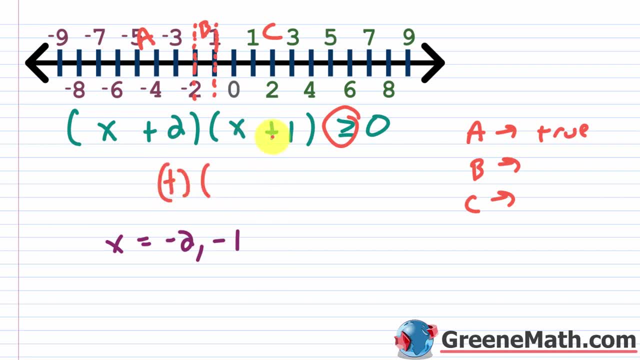 just say this is positive And then negative: 1.5 plus one is negative 0.5.. So this is negative. positive times. negative is negative and a negative is not going to be greater than zero or equal to, or it's going to be false. Now in c we can use zero And so this would be positive. two And this: 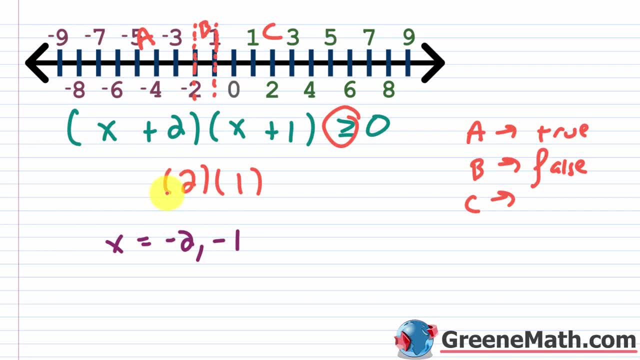 would be positive one, So it's two again. you can just think about the fact that this is positive times, positive which is positive, and a positive is greater than zero. you can say two is greater than zero, however you want to think about this, but this is true. Okay, so we know that. for the 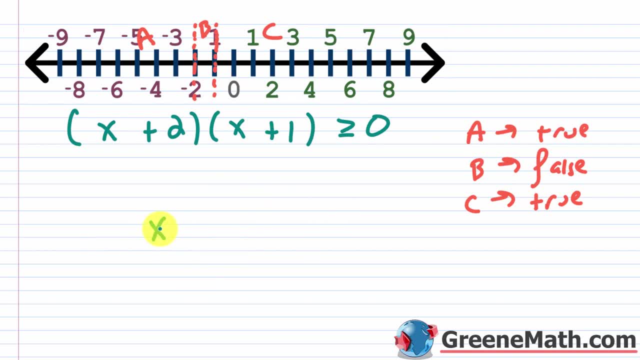 solution for this inequality now that, basically, x could be anything that's including negative two or less, so x is less than or equal to negative two. then, or x could be anything that includes negative one or is greater, so greater than or equal to negative one. Okay. 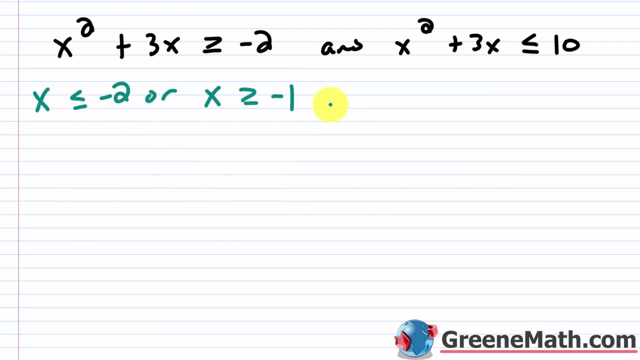 let's grab this And I'm just going to come back over here and put this right here. I'm going to use my keyword and, and then I'm going to look at the solution for this one. So let's put this down here. we're going to have x squared and then, plus three x, I'm going to subtract 10 away from each. 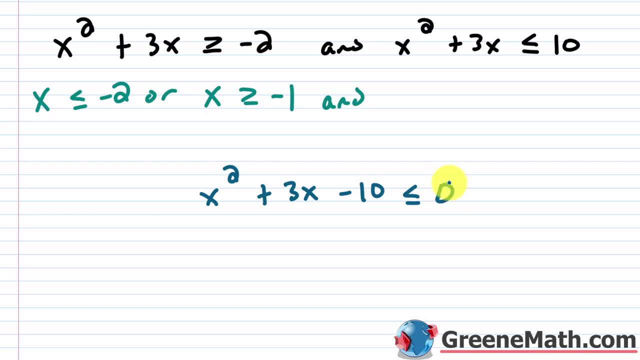 side. So minus 10, this is less than or equal to zero, And let's just factor this. I think it's a little bit easier that way. So let's put an x here and an x here And let's think about two integers. 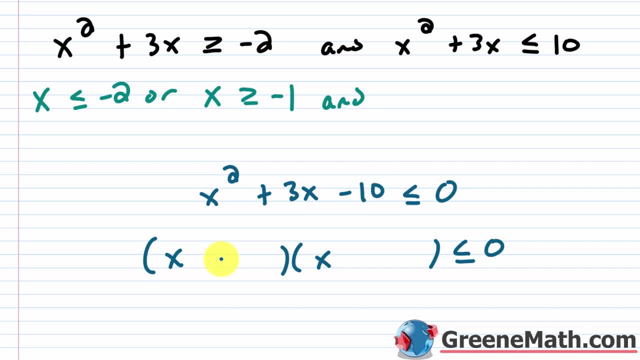 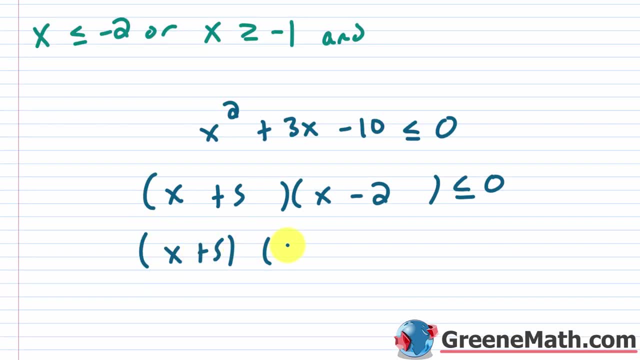 that sum to three and have a product of negative 10, where you can go positive five and then negative two, right? So if you set this up as this: quantity x plus five times the quantity x minus two is equal to zero, to get the critical values you solve: x plus five equals zero. well, that's. 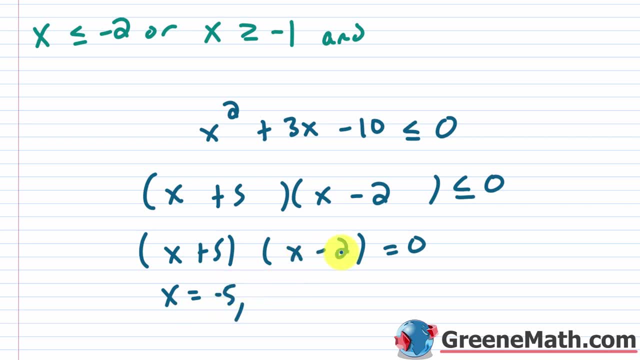 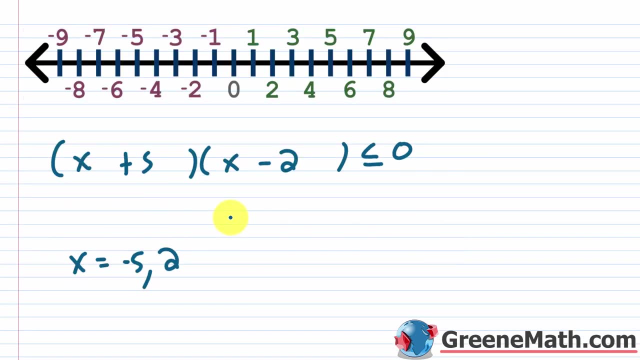 going to be: x is equal to negative five. And then you solve: x minus two is equal to zero. that's going to be x is equal to two. So let's grab everything And coming down here. we don't need this anymore. get rid of that, Your critical values here. you've got one at negative five. 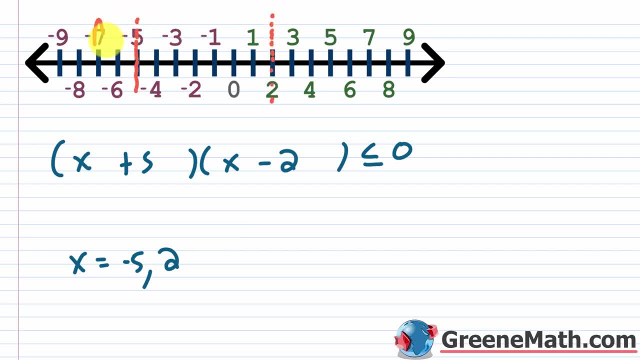 and then you've got one at positive two. So let's say: this is a, this is b and this is c. So let me write out a, b and c. So let's first start out in a and I'm just going to pick. let's say: 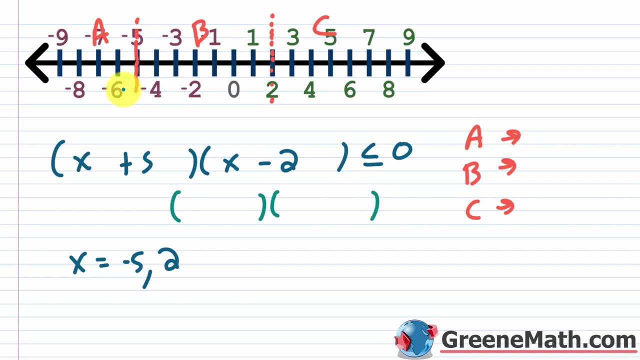 negative six. So again, you can just work with the sign if you want. So you'd have negative six plus five, that's negative one, And then negative six minus two is negative. eight, Again negative times. negative is positive And a positive is not less than zero and it's not equal to zero. So we would 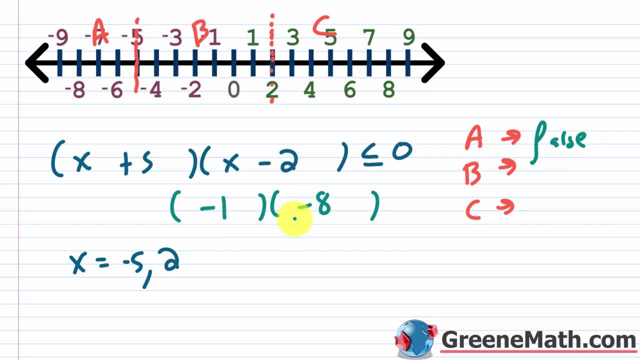 say here: this is going to be false. Again, if you wanted to say negative one times negative, eight is eight, and eight is not less than zero. that's another way you can do it. Okay, In b I'm going to pick zero. So this is five. 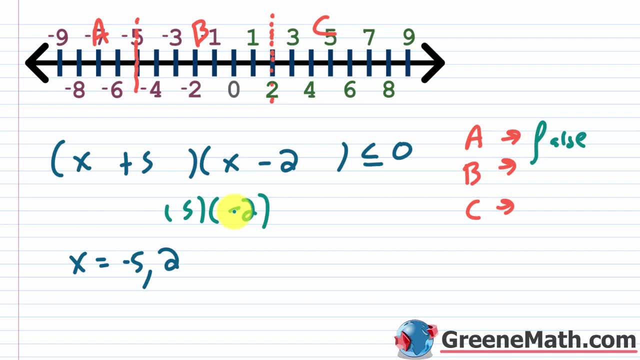 and then this is negative. two Positive times negative is going to be a negative, and a negative is always less than zero. So this is true. Or again you could say this is negative 10, and that's less than zero. It's true either way. Okay For c, you could pick three, So three. 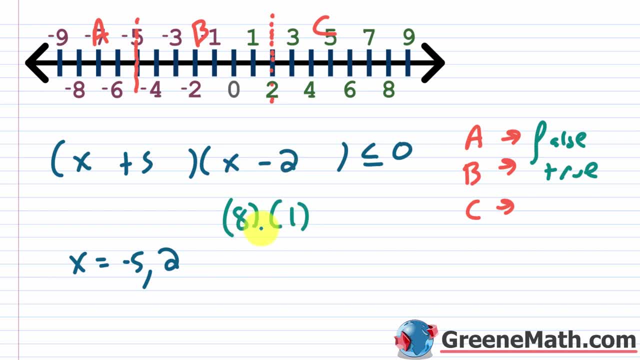 plus five is eight, And then three minus two is one, And again, this is going to be a positive and that's not less than zero. So this is false. Okay, Again, you could always say that this is eight and eight is not less than zero. So let's write our solution Here. it will. 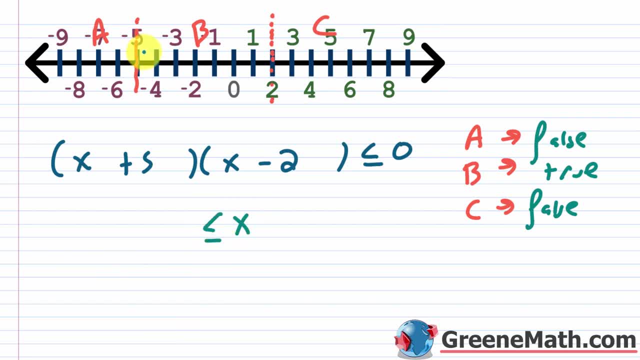 basically be that x is greater than or equal to, it would be equal to negative five, because this is non-strict, and less than or equal to this two- again because it's non-strict, the two would be included. Let me stack this up here so that it fits, And let me paste this in here, Okay, So. 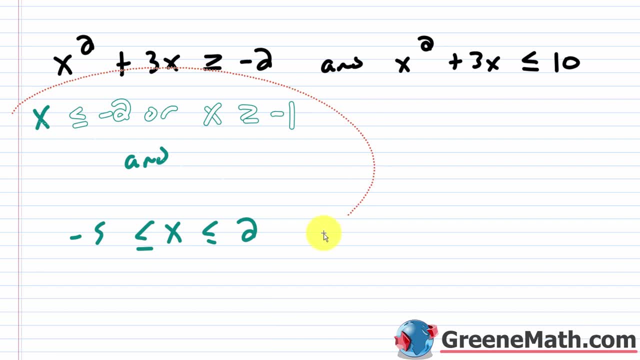 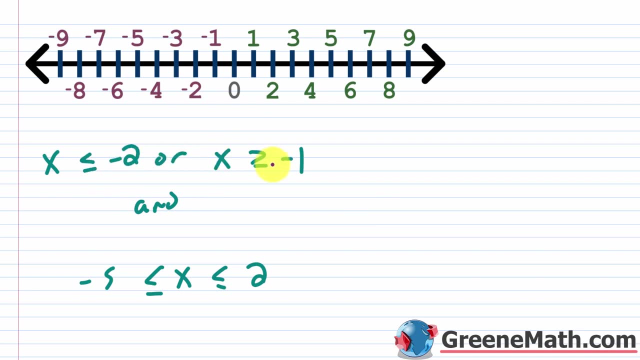 let's consider this. Remember, this is an and for the whole thing. So I'm just going to grab this and go back to the number line And we're going to think about where this works. Okay, So first I'm just going to graph this: So x is less than or equal to negative two. So let me put at negative. 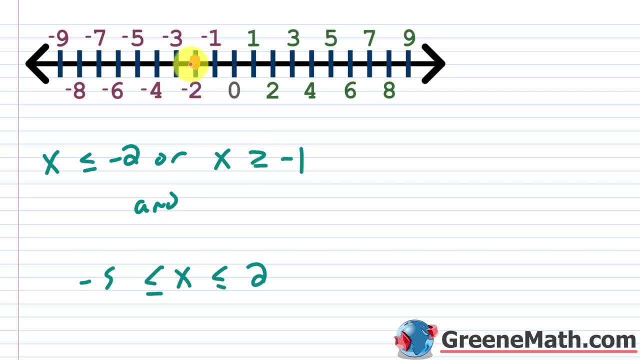 two, I'm just going to put a filled in circle. I don't normally do that, but for this one I think it's easier And I'm going to shade everything to the left. And then, for negative one, let's use a filled in circle there, And then, since it's a greater than or equal to, let's shade. 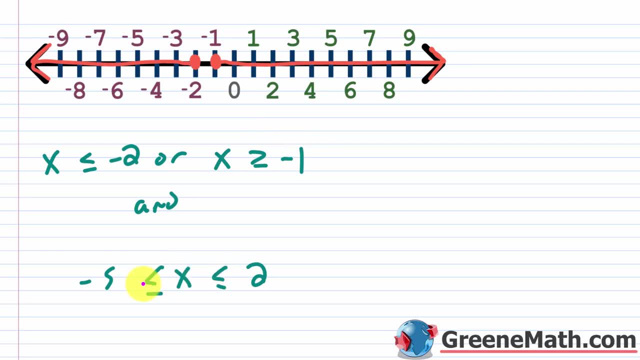 everything to the right. For the other guy you have, x is greater than or equal to negative five and less than or equal to two. So at negative five I would put a filled in circle, At two I would put a filled in circle, And again I would just shade everything in between. Now, 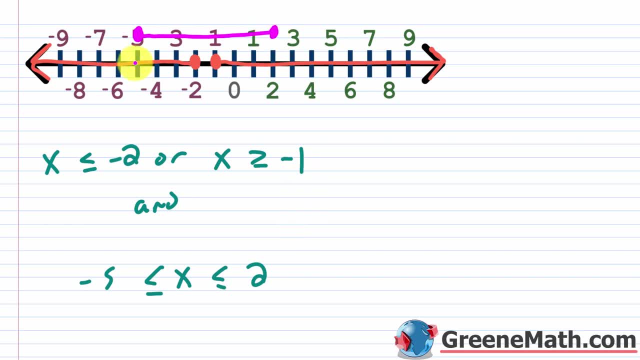 where's the overlap or the intersection? Well, this negative five would be a filled in circle there, This two would be a filled in circle there, And then, basically, what I would want to do is grab those guys in between right. So let me get rid of this, And so I'm just going to shade. 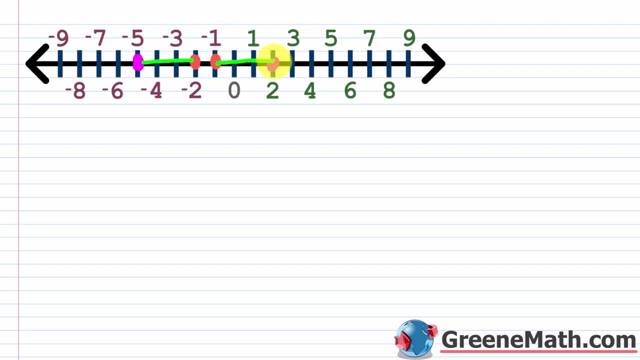 between negative five and negative two and between negative one and positive two. So our solution, if you wanted to write it, you would say: x is greater than or equal to negative two And less than or equal to negative two. Then you would say: or this would also work if x was. 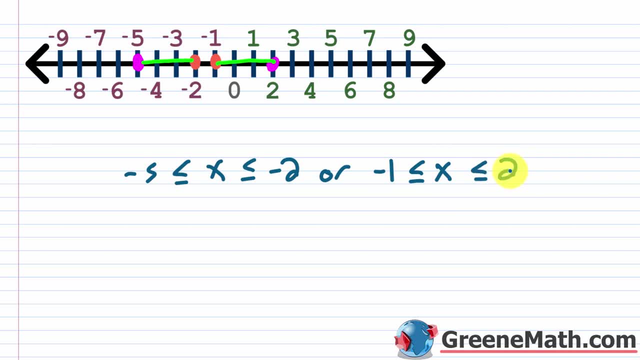 greater than or equal to negative one and less than or equal to two. So this would be our full solution here. In interval notation you would just put a negative five next to a bracket, then comma negative two next to a bracket. They're both included. And the union width: 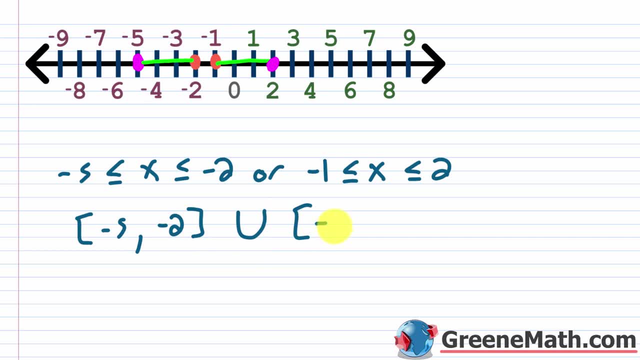 let me make that symbol a little bit better. So we would have a negative one next to a bracket and then comma a two next to a bracket. Okay, Now, graphically we have this already. I prefer to use a bracket versus a filled in circle, If you. 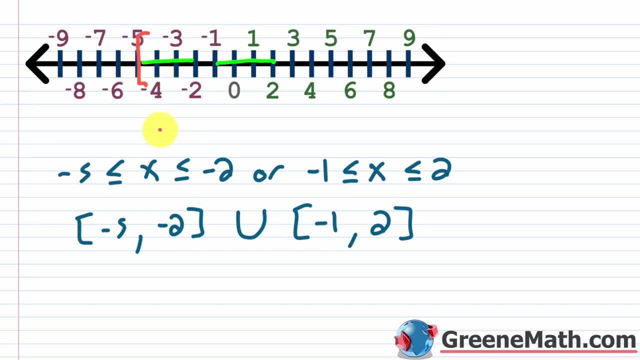 like the filled in circle. you can stick with that. It's just not what I usually do. So I want a bracket at negative five and a bracket at negative two, and then a bracket at negative one and a bracket at two. So let me make this a little bit better. I'll just use this same color. 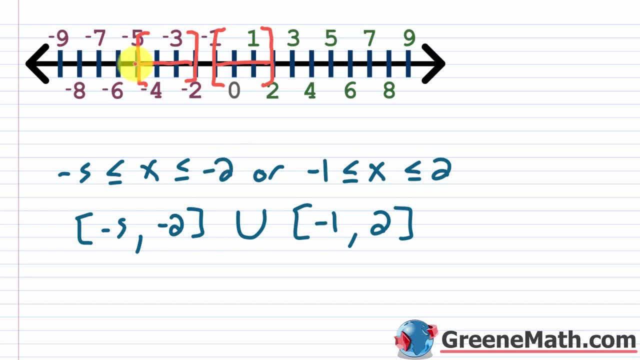 So, basically, x can be any number that is negative five and going up to and including negative two, or any number that starts with negative one and going up to and including negative two. Okay, So once again, I'm just going to look at the graph with you. We have graphed the left part. 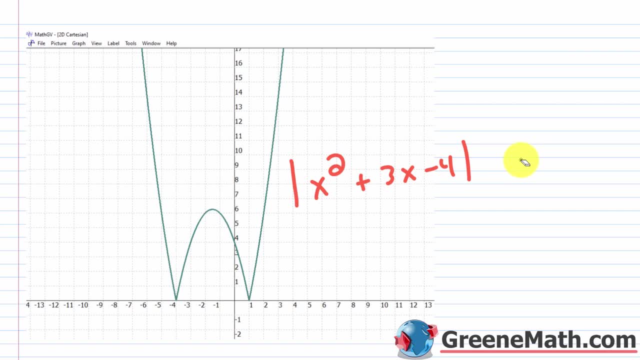 of this. We're trying to figure out where that's less than or equal to six. So let me just say that this right here. you could just punch this into Desmos or you could say y is equal to this. Either way it'll give you the same graph, But essentially you see a y value of six here. 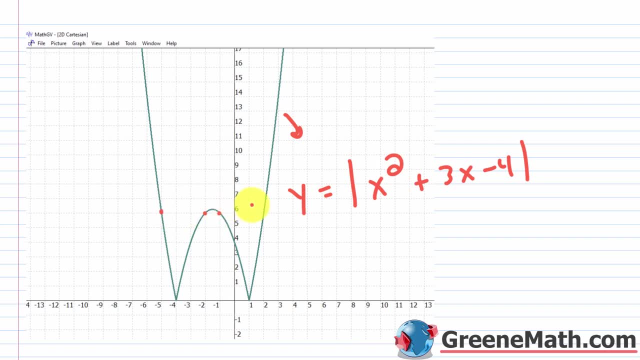 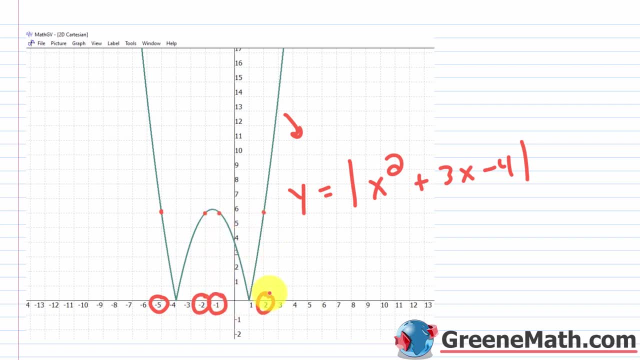 at an x value of negative one and then at an x value of two. Okay, So less than negative six. you would say between negative five and negative two. So x is greater than or equal to negative five and less than or equal to negative two, And then between negative two and negative one. 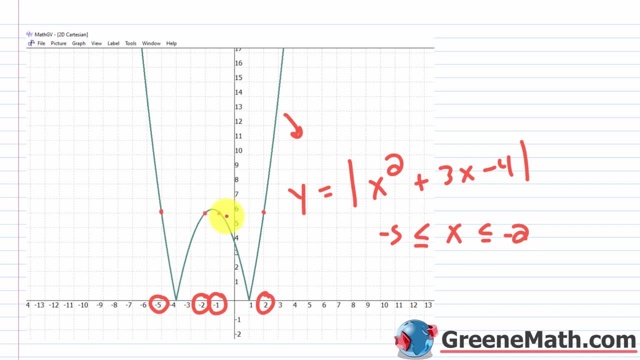 you can see, it goes above six right. So we're not interested in that piece. We're interested in this piece here, though, starting at negative one and then going out to and including this positive two right. Everywhere there would be either six. 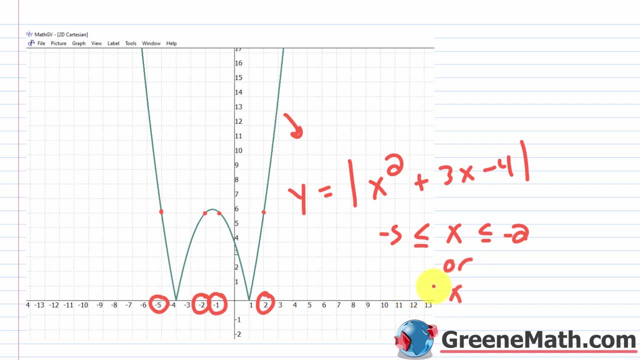 or less than six. So we'll say: or again, x is greater than or equal to this negative one and less than or equal to positive two. So that's how you can get your solution graphically. Again, we're interested in everywhere where this guy is going to be less than or equal to six. 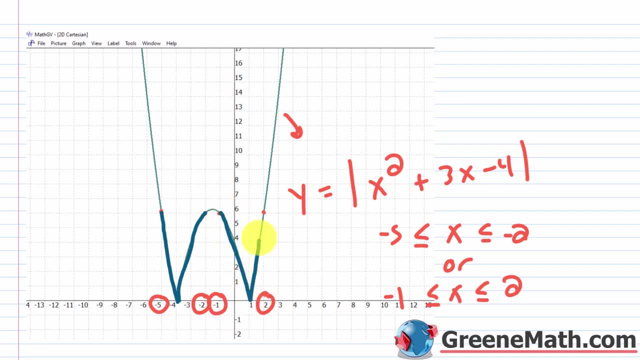 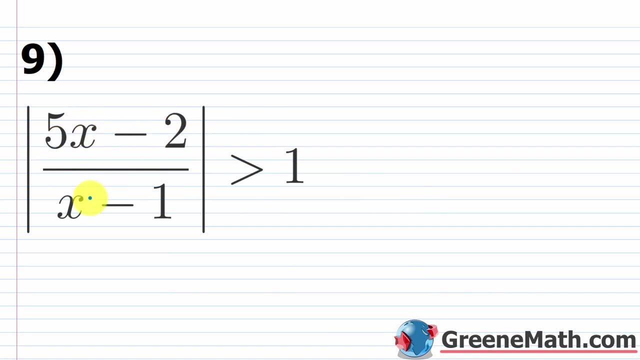 So that part right there and then also this part right here for your graph. All right, let's take a look at problem number nine now. So here we have the absolute value of five x minus two. this is over x minus one. 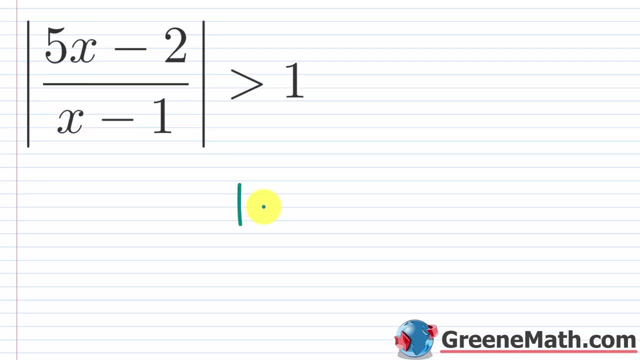 and this is greater than one. So we're going to use our rule and say: if we have some algebraic expression u and that's greater than some positive number, let's just use one. then here u is going to be less than negative one, or u is greater than one, So we're just going to use that. 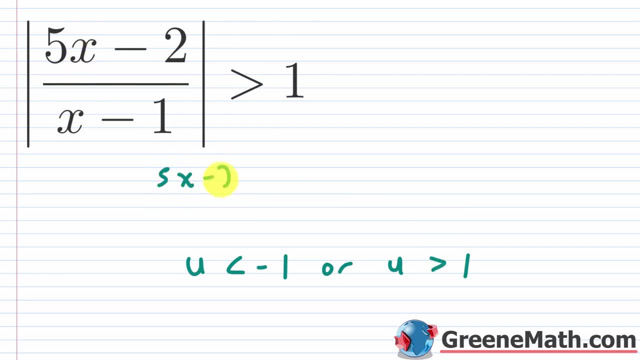 here And we'll take this guy, which is the five x minus two, over x minus one. that'll be our u, So we'll say it's less than negative one then, or we'll grab this guy again, So five x minus two over x minus one and we'll say it's greater than. 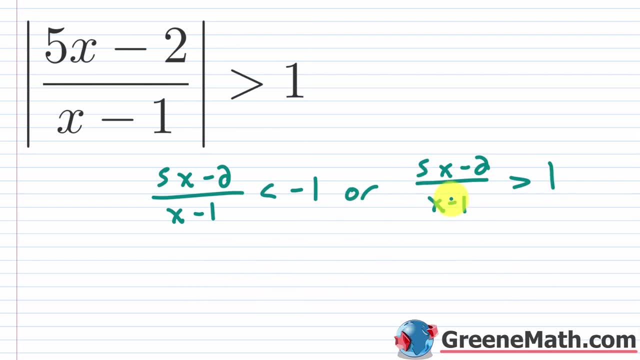 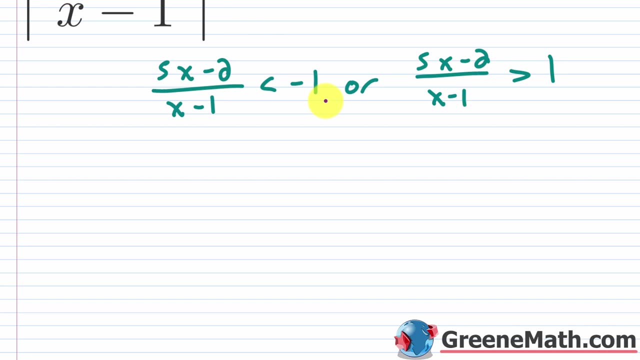 one, Okay. so now that we have this set up- we know that this is a tedious process- we have to solve two of these guys. I'm going to start with the one on the left. Remember, you want to get one single rational expression on the left and you want zero on the right. Okay, so that's the 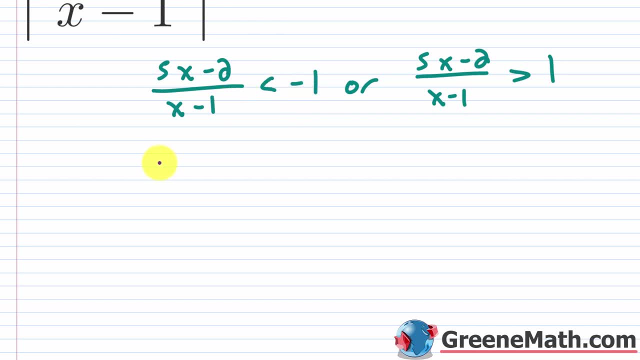 first step. So I would add one to both sides of the inequality. I would say this is five x minus two over x minus one Plus one, and this is less than zero. So I just added one to both sides. Now you need to get a. 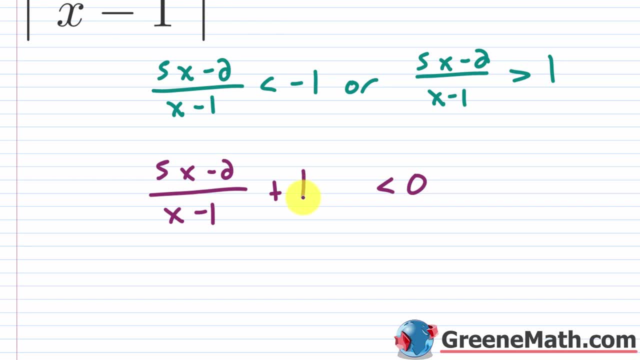 common denominator going And since this is one, I can just multiply by x minus one over x minus one. So in other words, I can just write this as x minus one over x minus one And since we have a common denominator now, I can actually just get rid of this and just extend this and just go plus. 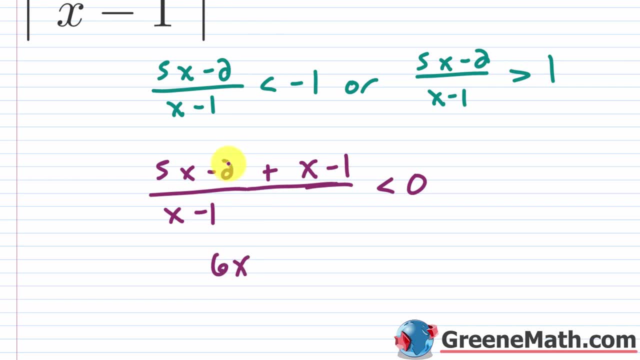 here. So, simplifying this, five x plus x would be six x, and then negative two minus one would be negative three. Let me actually just erase this. I'm going to write this more neatly up here. So the numerator is six x minus three and your. 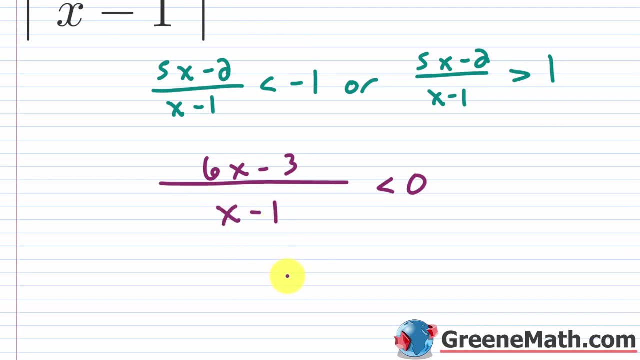 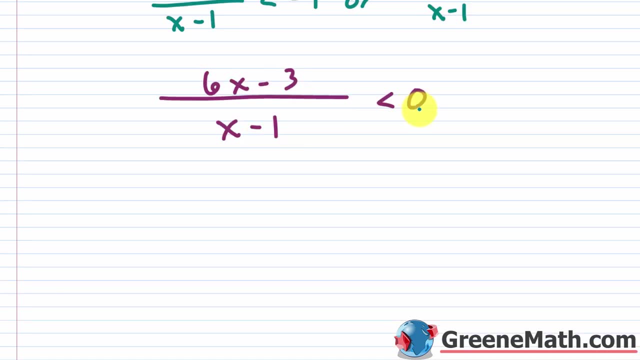 denominator is just the x minus one. Okay, when we think about this, we want to find the critical values. So this is where the numerator is going to be equal to zero or the denominator is equal to zero. So we say: six x minus three is equal to zero. we solve that And basically this gives us. 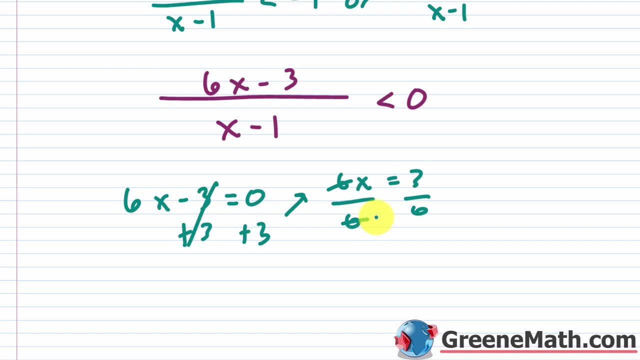 that six x is equal to three. divide both sides by six. this cancels, you get x is equal to a half. Okay, so that's your first critical value. If we had a non strict inequality, this would be part of your solution. you could just notate that. 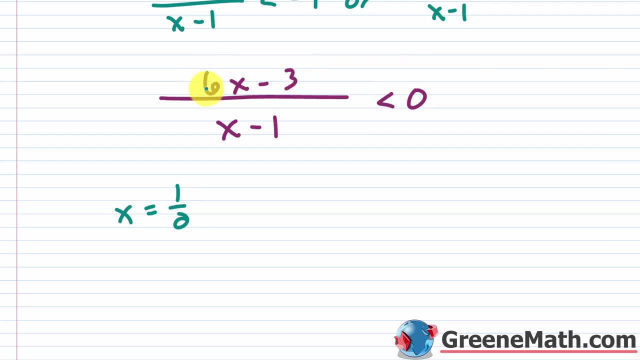 if you want, Because this is a strict inequality Here. when you plug this in, this one half the numerator is zero, the denominator is not zero. So zero over some non zero number is zero and you get zero is less than zero, which is a false statement. Okay, so this is not going to. 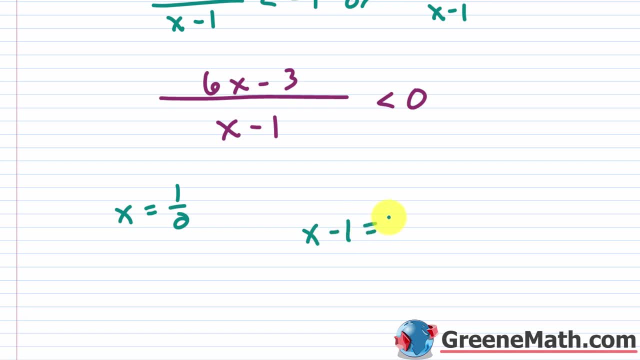 work as a solution. And the other guy where we say x minus one is equal to zero, the solution here, if we add one to both sides, we're going to say x is equal to one. Now that guy, right, there is definitely not going to be a solution because that results in division by zero, right? So if we 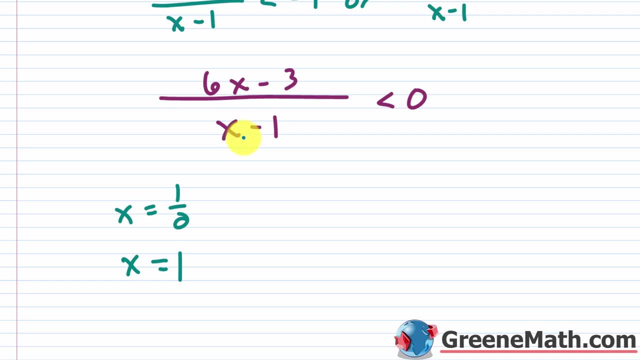 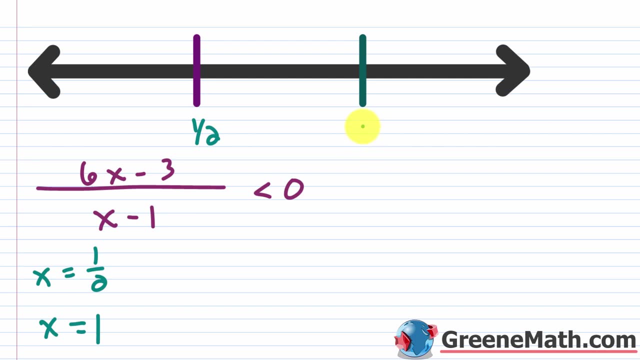 made a domain statement. we would say it's the set of all x, such that x is not equal to one. Okay, so let's grab this real quick And we'll just come to a little number line and test. I'll say: this is one half and this is one. you can get rid of this now And again. 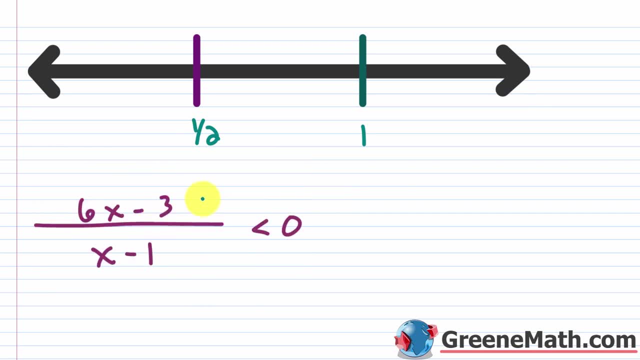 we know they're both not going to be included. And you could factor this: this would be three times the quantity two x minus one. So let me write this like this: So three times the quantity two x minus one. just easier to do, Okay, so we're going to do this. So we're going to do this. 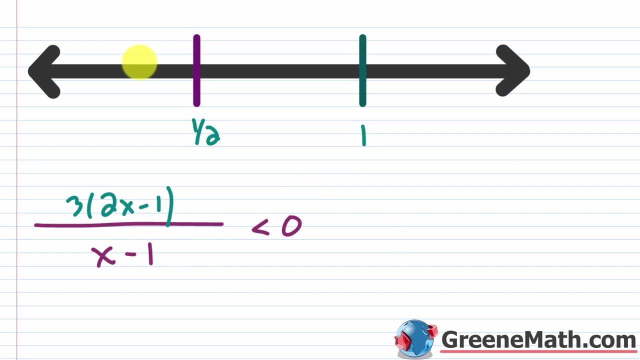 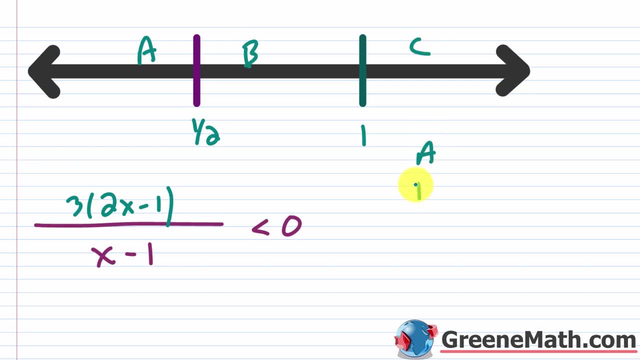 B is between a half and one and C is greater than one. So we have A, B and C And let's first test an A So I can pick zero. So two times zero is zero. So basically you would have negative one. 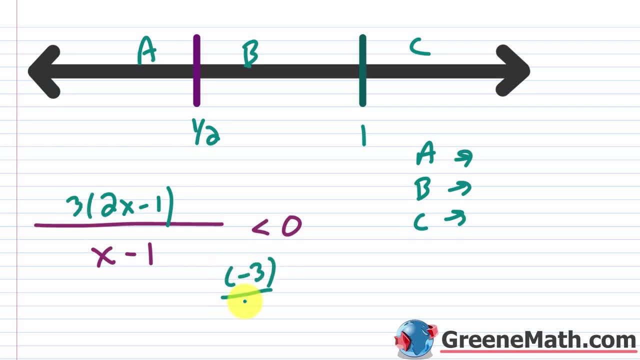 times three, which is negative three. this would be over. you have zero minus one, which is negative one, And so a negative over negative is a positive, And so a positive is not less than zero. So this is false. And again you can always just say that negative three divided by negative one is: 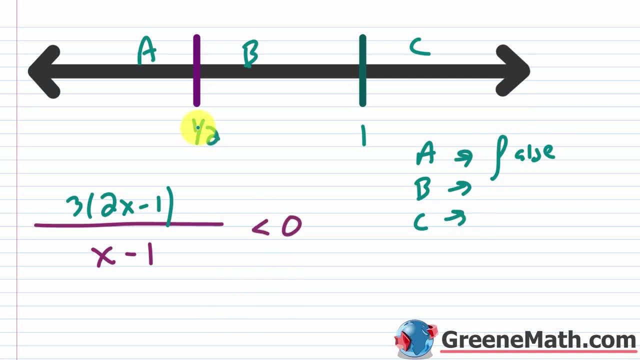 three three is not less than zero, whatever you want to do. So for B I need something between one half, or you could say point five and one. you could pick point seven five. I know that's hard to work with, But let's just use a calculator. So let's just say that's point seven five. 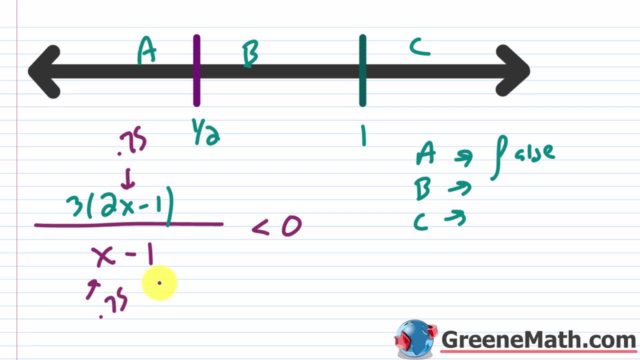 you could also say three, fourths. Let's go point seven, five there. So two times point seven, five, that's 1.5, then minus one is point five, then times three is 1.5.. Right, so you could say three. 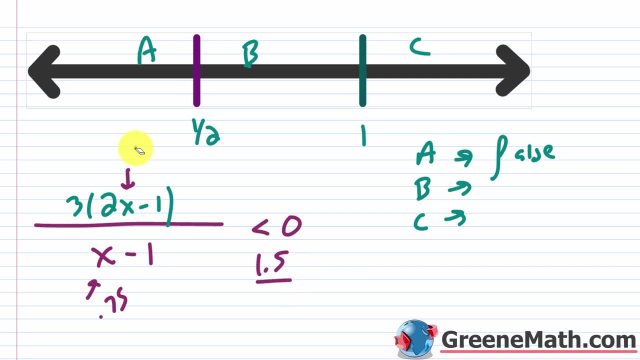 halves or 1.5, whatever you want to do. So you could say three halves or 1.5,, whatever you want to do. then this is over. let me actually just get rid of this Point. seven five minus one. 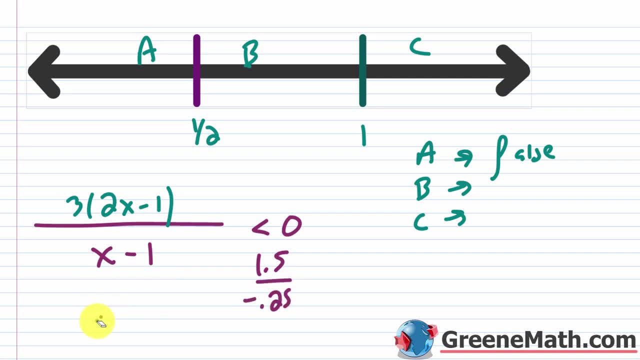 is negative. point two: five. Now you don't even need to know what the result of this is, because you know it's going to be negative, right, And the negative is always less than zero. So this is true. If you did punch this into your calculator, you would get negative six. 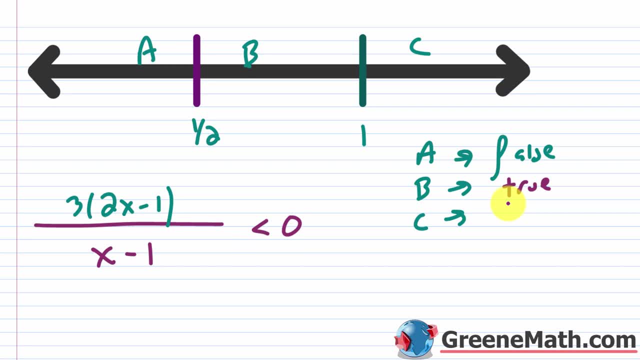 So you could just say: negative six is less than zero. That's a true statement. So either way then. for C, let's just pick two. So two times two is four, four minus one is three. three times three is nine, And this is over. 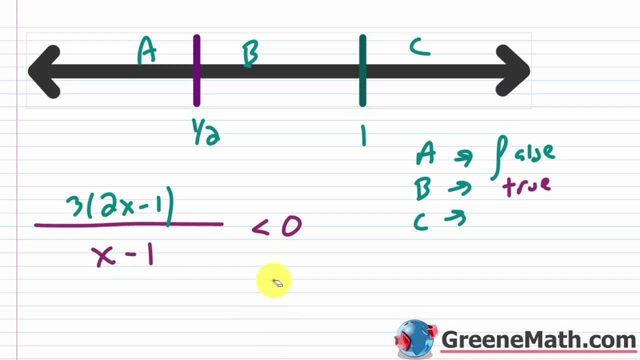 Two minus one, that's going to be one. So this is nine or a positive value, And that's not going to be less than zero. So this is false. So your solution here is between one half and one, with neither included. So we'll say x is strictly greater than a half and strictly less than one. 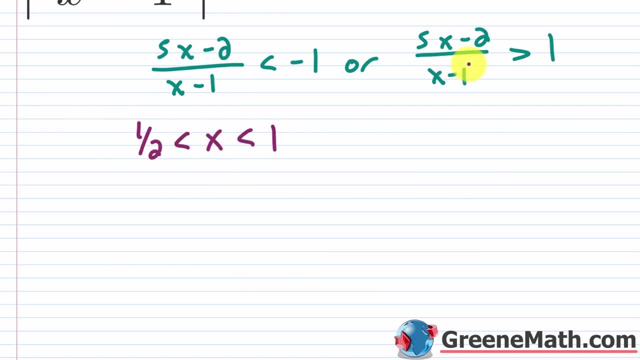 a coming back here. So I'm gonna put that as the solution for this one, And then we're dealing with this one now. So let me put my keyword, or So I'm going to have this: five x minus two over x minus. 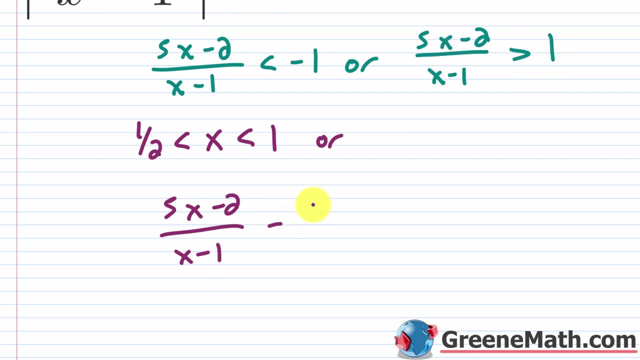 one. Now I'm going to subtract one away from each side of the inequality. So minus one over here is greater than zero. So this again you could just write as x minus one over x minus one, Because this is subtraction. let me take the time. 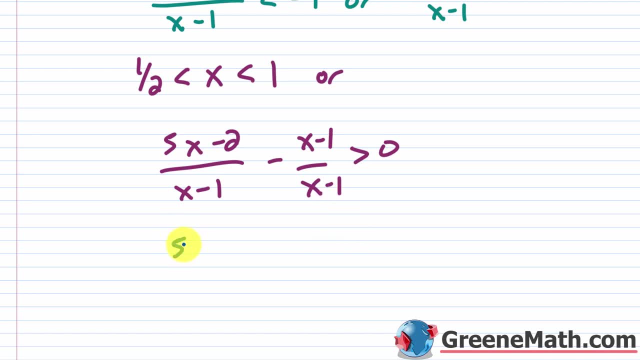 to do an additional step here, because a lot of people get lost. So let's say: this is five x minus two, and then minus the quantity x minus one, because this whole thing needs to be subtracted away. So I'm going to put the subtraction sign and then put the x minus one inside of parentheses. 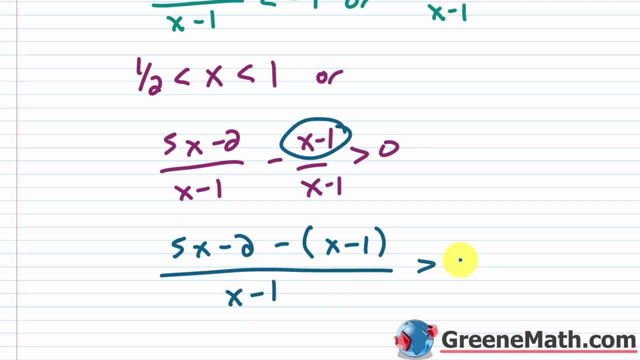 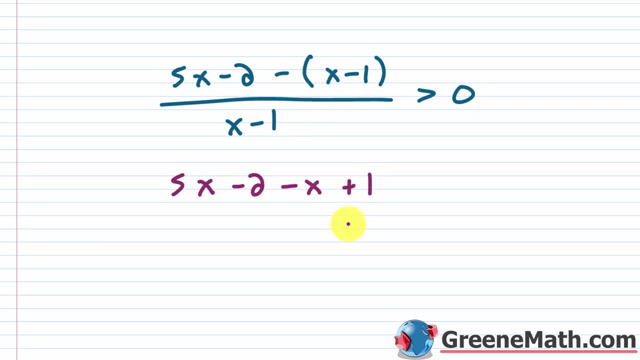 Speaker: 1, Then this: This is over the common denominator of x minus 1, and this is greater than 0.. All right, so let's write this as 5x minus 2, and this would be minus x and then plus 1.. 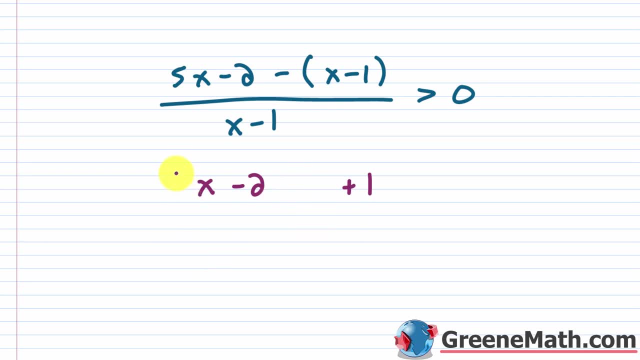 So 5x minus x would be 4x, so this is 4x, and then negative 2 plus 1 would be negative 1.. So this is 4x minus 1 over x minus 1, and again this is greater than 0.. 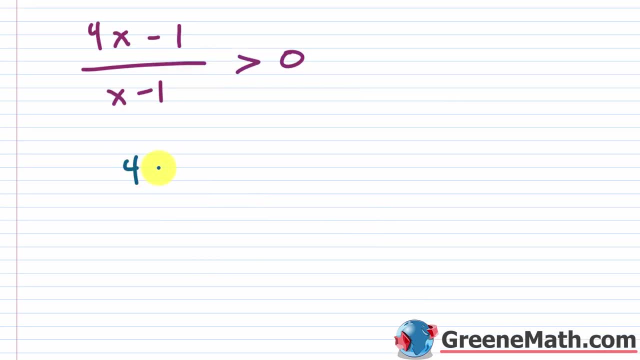 So what are the critical values here? Well, we would set the numerator 4x minus 1 equal to 0, and solve that. Let's add 1 to each side. This would be: 4x is equal to 1.. 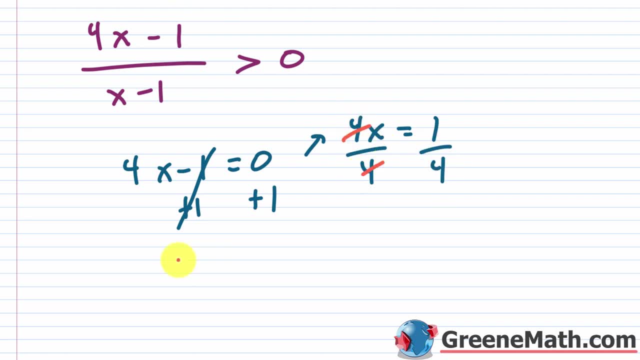 Divide both sides by 4.. Let's cancel this and say x is equal to 1: 4th, So that's one critical value and again this is going to be excluded because this is a strict inequality You would end up with: 0 is greater than 0, which is false. 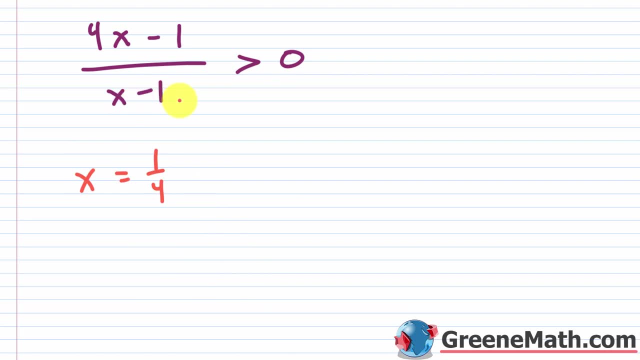 So let's put this over here. The other one is the x minus 1 that we saw earlier. If we set that equal to 0 and solve, we get x equals 1.. So x equals 1.. Remember, this is automatically. 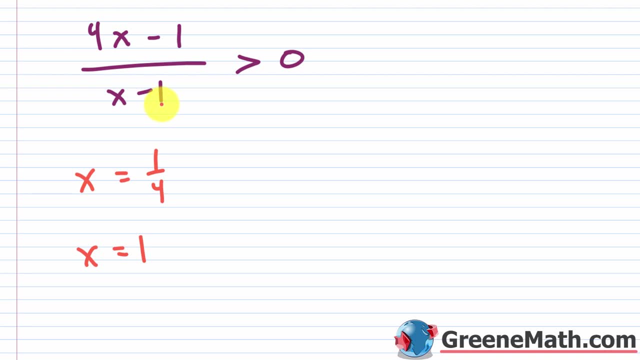 It's not going to be excluded because it makes the denominator 0, so it would violate the domain. So let's grab this, So we'll come down here and test. So this is a 4th and this is 1.. 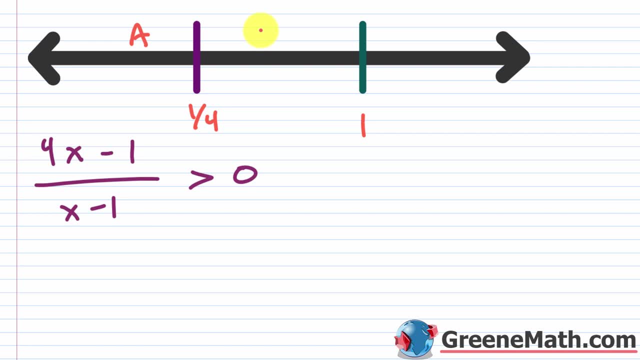 So let's think about this as a, so anything less than a 4th. This is b, anything between a 4th and 1, and this is c, anything greater than 1.. Okay, so in a you could pick 0, and again you could just think about the sign. 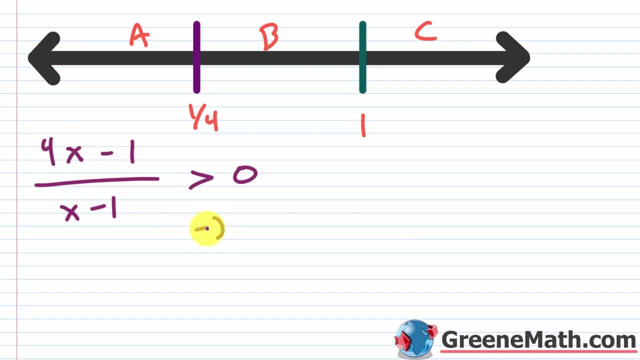 This is really easy. This would go away. You'd have negative 1, or just a negative over this would be negative 1, or just a negative, and a negative divided by a negative is a positive and a positive is always greater. 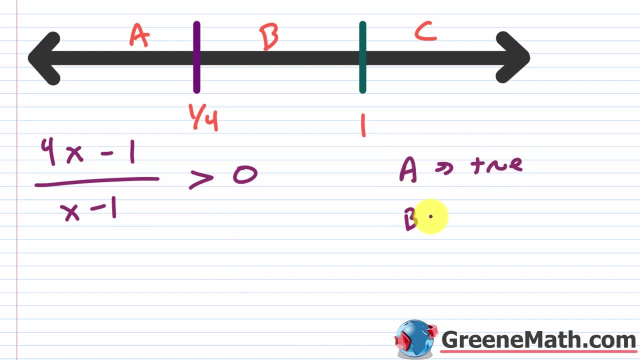 than 0. So for a, this is going to be true Again. if you want to calculate the value, you can do that as well. This would be negative 1 over negative 1, which is 1, and 1 is greater than 0.. 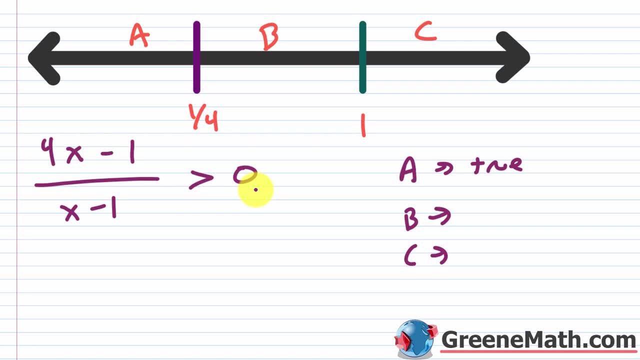 So either way. Now for b, I would just use something like a half, or you could say 0.5.. So 4 times a half is 2, and then 2 minus 1 is 1.. So you could say it's 1, or you could just say it's positive. 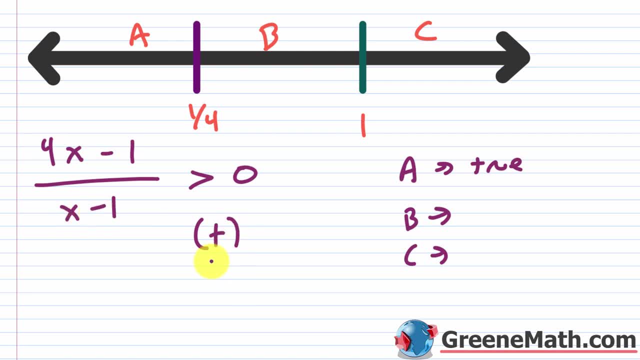 Then, additionally, if I did a half minus 1, that's negative 1.. So I would just use something like a half, or you could say 0.5.. If I did a negative 1 half, more importantly, it's negative right. 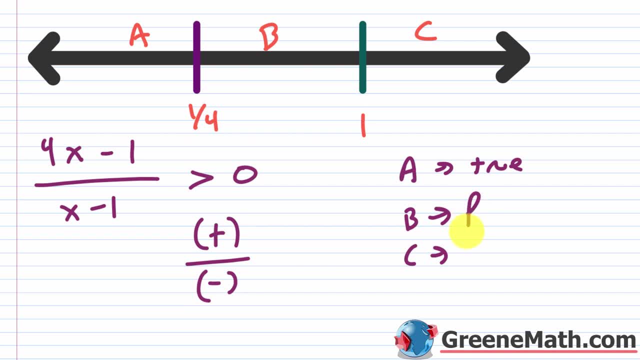 So positive over negative is negative. a negative is not greater than 0, so this is false. Again, if you want to calculate that, 1 divided by negative 0.5 would be negative 2, and that's not greater than 0.. 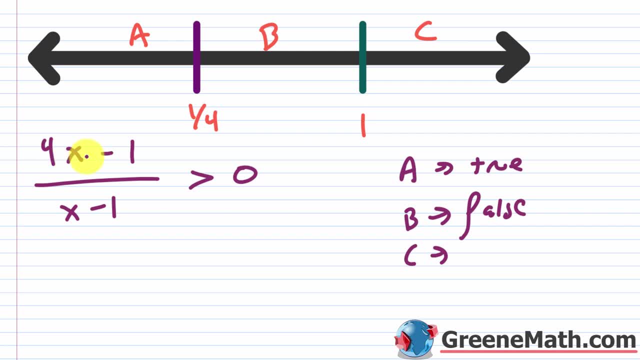 Okay, for c let's just use 2.. So 4 times 2 is 8,, 8 minus 1 is 7, or again you could just say it's positive and this is over. 2 minus 1 is 1, right. 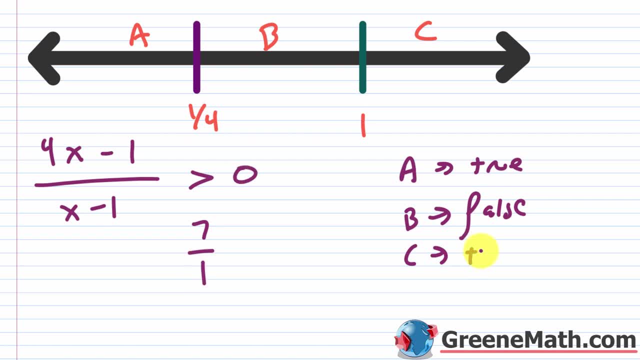 So you would say positive over positive is positive, that's greater than 0, so this is true. Or you could just say 7 over 1 is 7,, 7 is greater than 0. That's true. So either way, 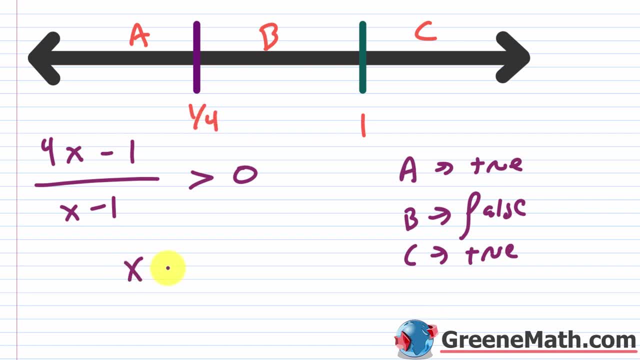 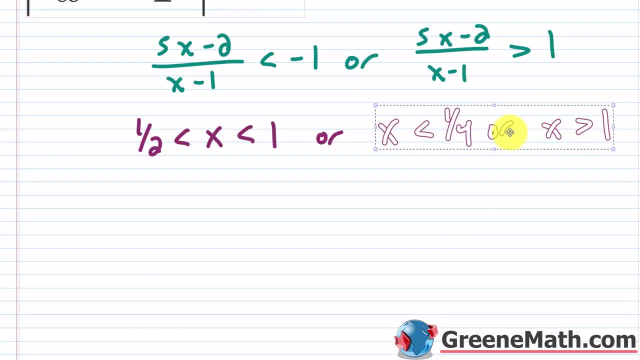 So we know that the solution here would be anything where x is less than a fourth or anything where x is greater than 1.. Okay, let's grab this and we'll paste that in there And basically this is our solution. 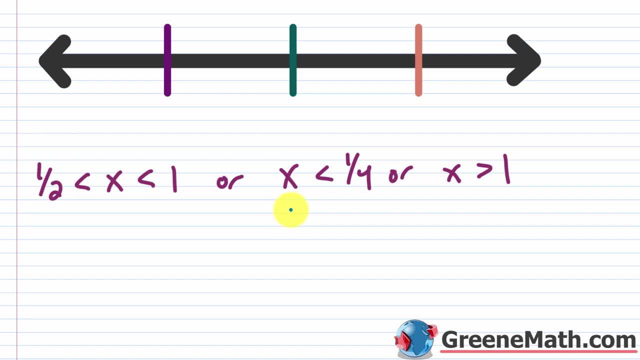 So, putting this together, it might be more helpful to graph it before you do your interval notation. So if you look through, you're going to see 1 fourth, 1 half and 1, okay. So you need a notch for 1 fourth, you need a notch for 1 half and you need a notch for. 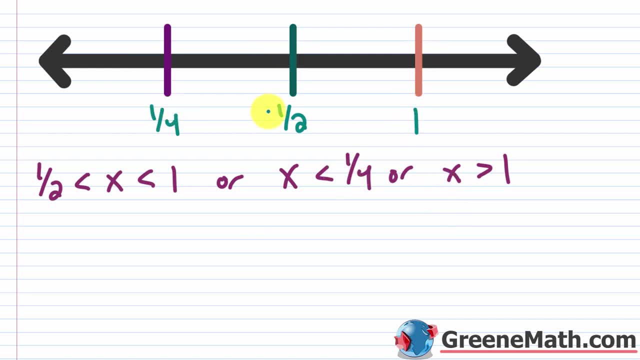 1.. So if you're using something generic like this, don't worry too much about the spacing. just make sure it's in the order of the number line. So in other words, 1 fourth is the leftmost value, 1 half is the middle value and 1 is 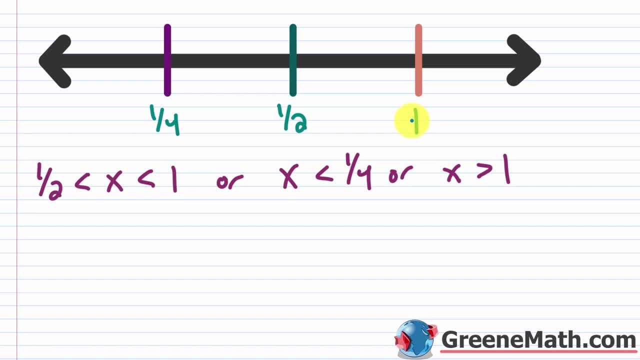 the rightmost value or the largest value. So now, thinking about this, this part right here tells me that x is less than 1 fourth. So let me just start with that. Graphically, I would put a parenthesis at 1 fourth to show it's not included and I 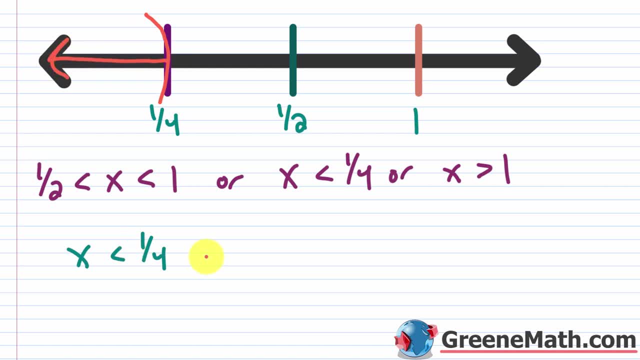 would just shade everything to the left. So that takes care of that. Then I'm going to say: OR I'm just going to get rid of stuff as I go. You have this part right here where x is greater than 1 half and less than 1.. 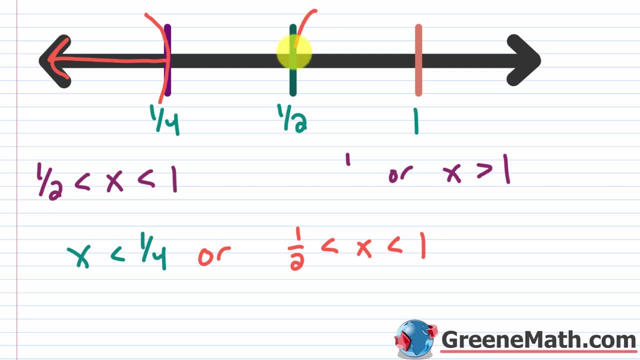 Okay, so what does that look like? Well, I would put a parenthesis at 1 half and I would put a parenthesis at 1, that color's not going to show up there, so let me change, And then I would shade everything in between here. okay. 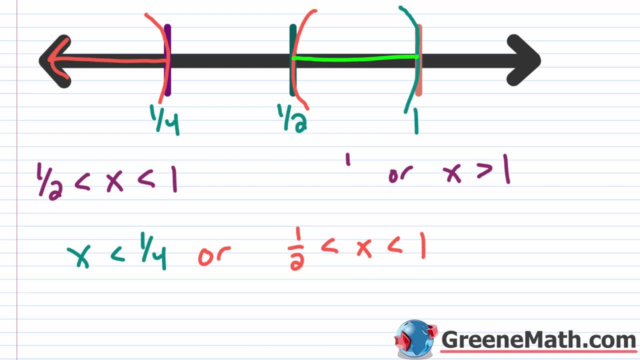 So that would be that part there. Then you have this OR this, OR let me get rid of this. so far you have, x is greater than 1.. Okay, so for that one, let me use a different color here, maybe this red, and so I'm going. 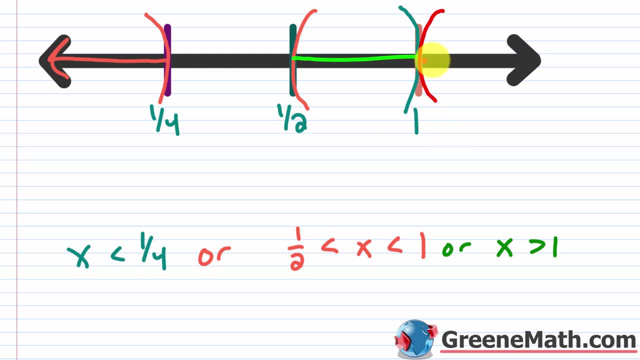 to put a parenthesis facing to the right here, and then I'm just going to shade everything to the right. So 1 is excluded, and if you go back to your original rational expression, remember the denominator was x minus 1, and if x minus 1 was set equal to 0, you get a value of 1.. 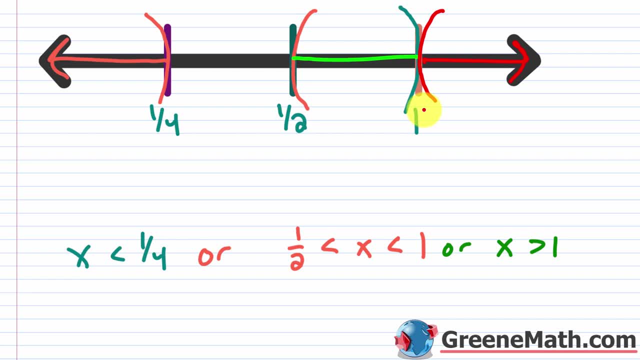 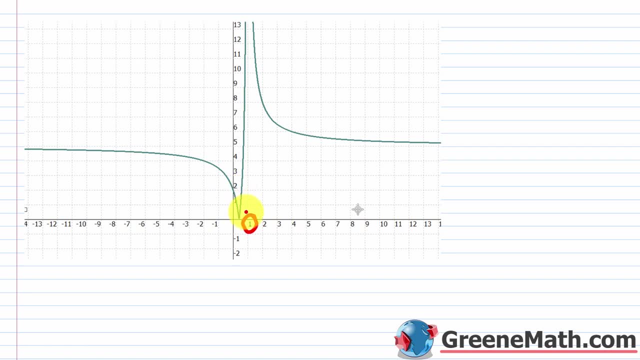 In other words, if you plug 1 in, you're going to get division by 0, and that's not defined. If we come to the graph, you're going to see at 1, you have this strange behavior, This strange behavior where the graph is going to approach an x value of 1, but it's never. 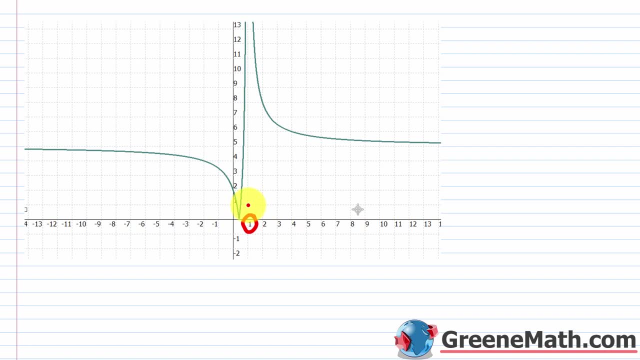 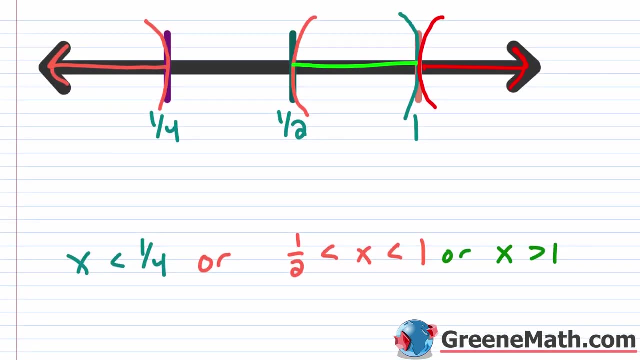 going to quite get there, okay, And this is called an asymptote, and we'll talk about this later on in the course. Right now, let's go back and let's think about this guy in interval notation. So basically, I would start with this one. 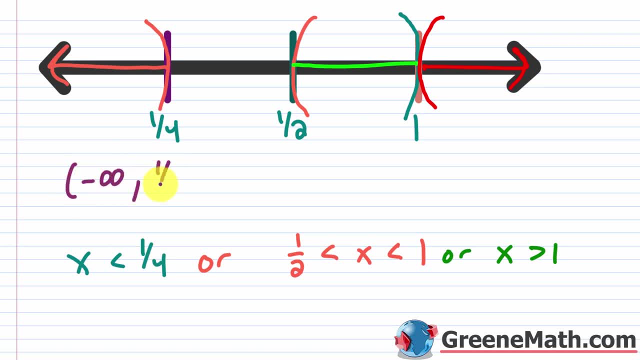 So you have from negative infinity going up to and excluding 1 fourth, so a parenthesis with each and then the union width. you have anything between 1, half and 1, so basically a parenthesis next to 1 half and a parenthesis next to 1, and then basically a union with. 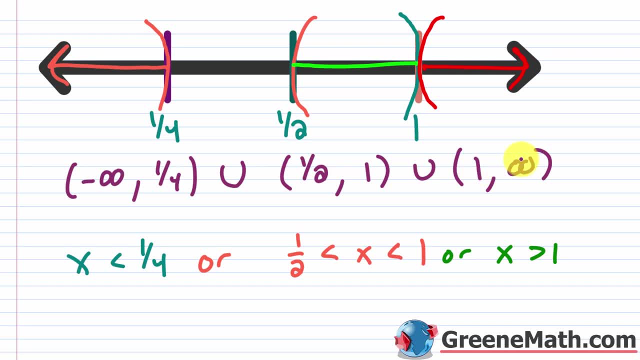 anything that's greater than 1,. okay, So a parenthesis next to each, So nothing here, when you go through, is actually included. That's why there's a parenthesis basically everywhere, and if you wanted to replace this with an open circle instead of the parenthesis, that's fine in each case, right? 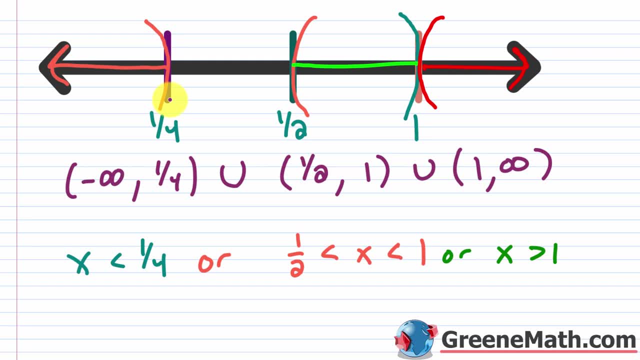 So that's what a lot of books will do. I'm just used to this notation, So this would be your full answer. This is graphically So: anything less than a fourth, Or anything that's between a half and 1. Or anything greater than 1.. 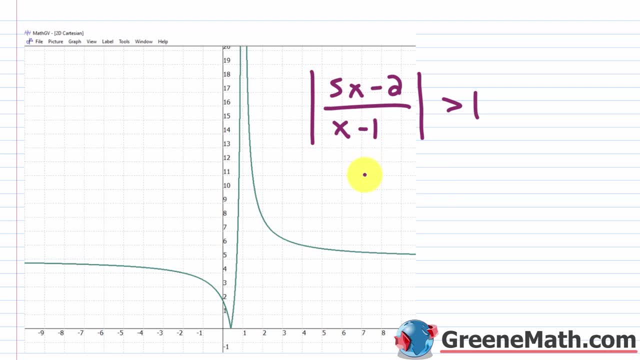 All right. so, additionally, if you want to come back to this graph and think about it, if you punch in this guy right here, this left side, into Desmos- or you could just say that y is equal to this- it'll produce the same graph essentially you're looking for. 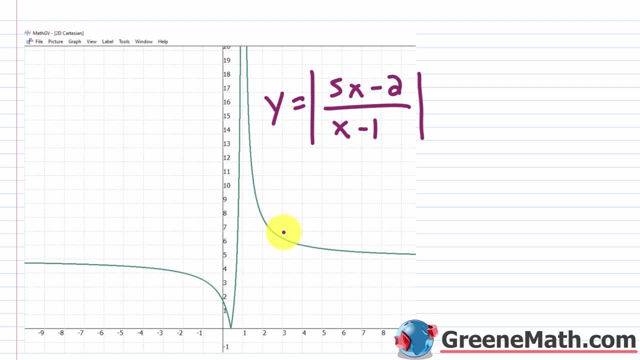 where the y value is greater than 1.. Not equal to 1, but greater than 1.. It would be equal to 1 here and also here, right? So essentially, if you come down here- and this is not going to be perfect- this x value. 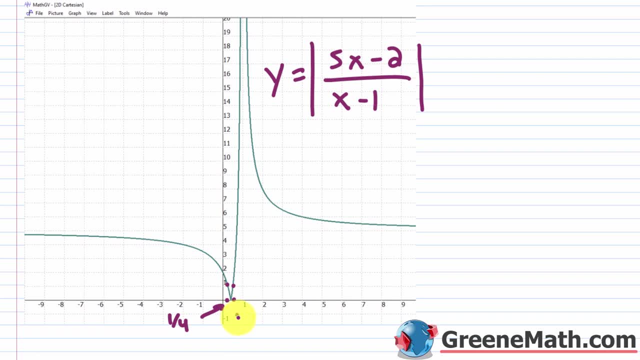 is 1 fourth, And then this guy coming down here, this is going to be 1 half, And so essentially you'll see that anything to the left of an x value of 1 fourth, well, the y value here is going to be greater than 1.. 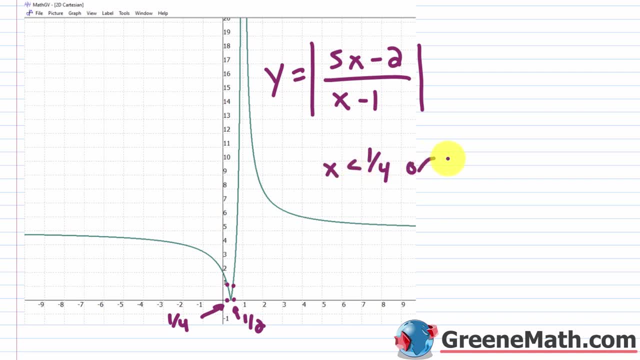 So that's where we got the x is less than 1, fourth part. Then we said: or Well, here, anything that's greater than a half, you can see that the y value would be greater than 1.. But there's a problem. 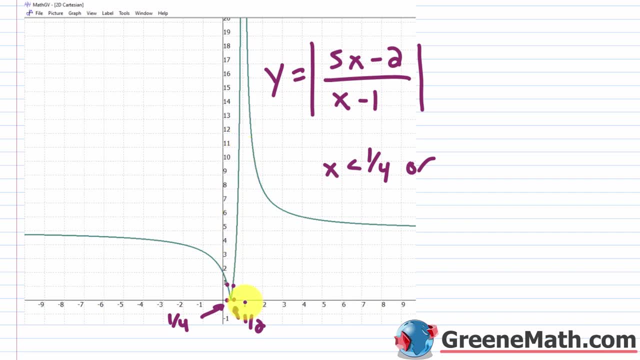 We keep going up, up up like this, because, again, at an x value of 1. You're dividing by 0, right? So that's why we can never actually obtain an x value of 1.. So you have to say that x is greater than a half and less than 1, right to account. 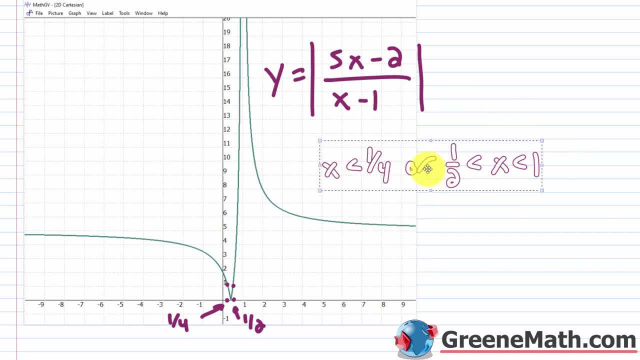 for that fact. But anything greater than 1 starts to work again. okay, So we're just going to exclude 1.. So we'll say: or x is greater than 1.. So that's how you could get your solution graphically. 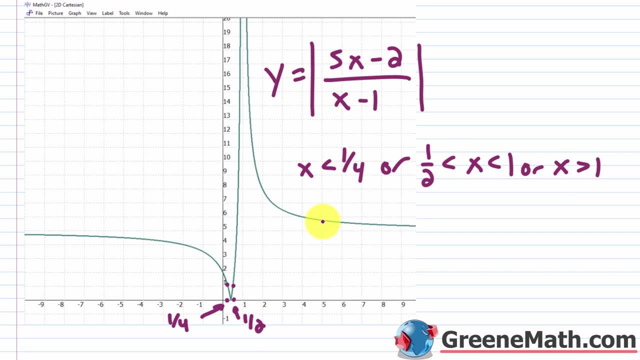 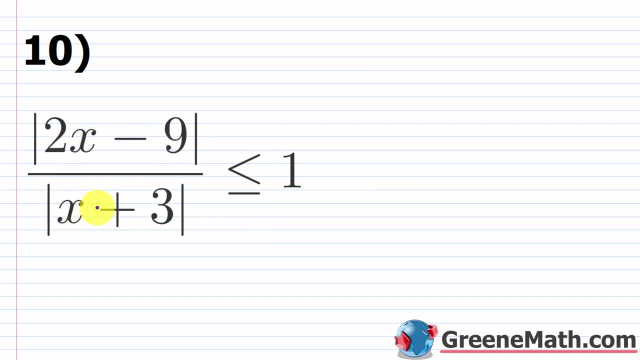 Again, you can always just use something like Desmos to see this for yourself. All right, let's take a look at problem number 10 now. So here we have the absolute value of 2x minus 9.. Over the absolute value of x plus 3,, this is less than or equal to 1.. 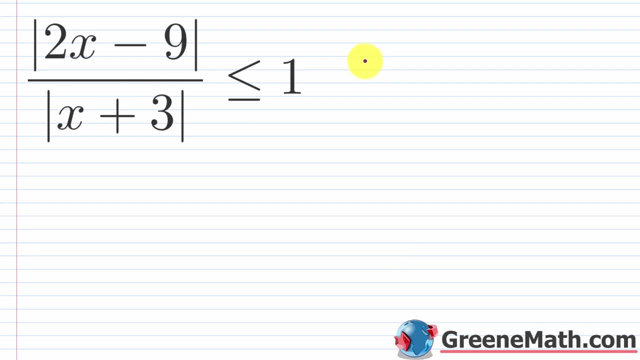 Now, the first thing I'm going to do is use a rule that we talked about earlier in the course. So if we have something like the absolute value of a over the absolute value of b, this can be written as the absolute value of a over b. 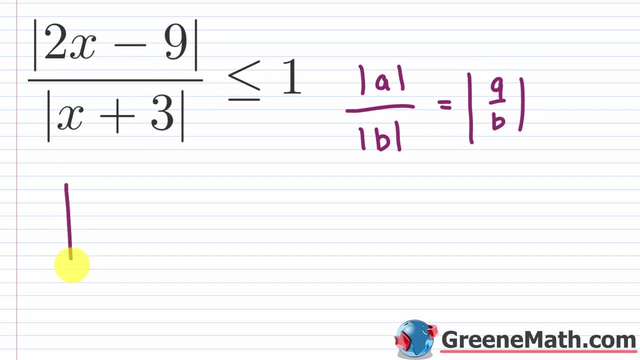 Okay, so we're going to make this little change here. So we'll say this is the absolute value of this 2x minus 9 over the x plus 3 here, And we'll say this is less than or equal to 1.. 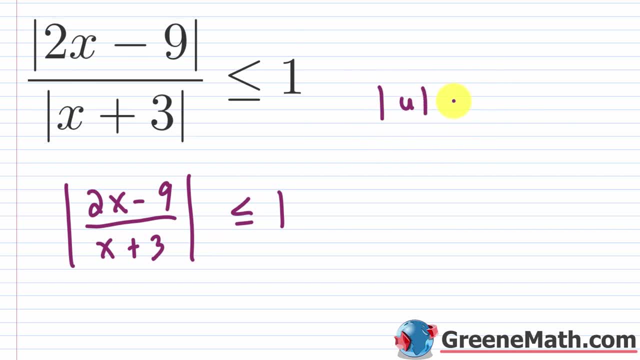 So now we're going to use a different rule. So if we had the absolute value of u and we said this is less than or equal to 1,, well, that means that u is greater than or equal to negative 1 and less than or equal to 1.. 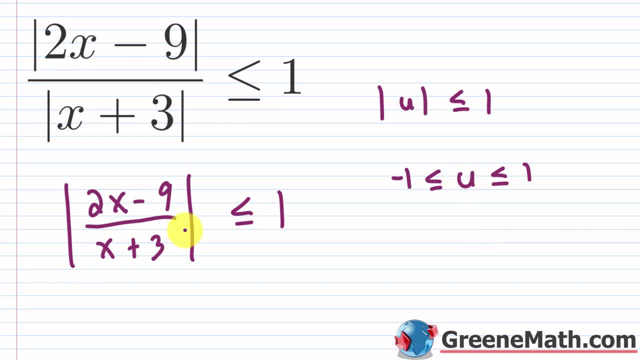 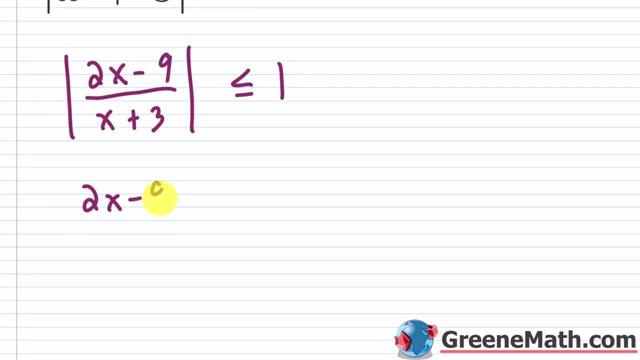 Okay, so I'm not going to write this as a three part inequality. I'm going to break it up and use the keyword, and I think that's going to be a little bit better here- And so I'll take this guy, this 2x minus 9, over x plus 3.. 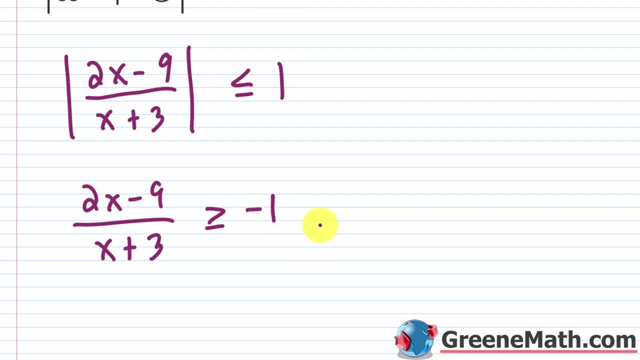 And I'll say that it's going to be greater than or equal to negative 1.. And then I'll say: and this: 2x minus 9.. Over this, x plus 3 is going to be less than or equal to positive 1.. 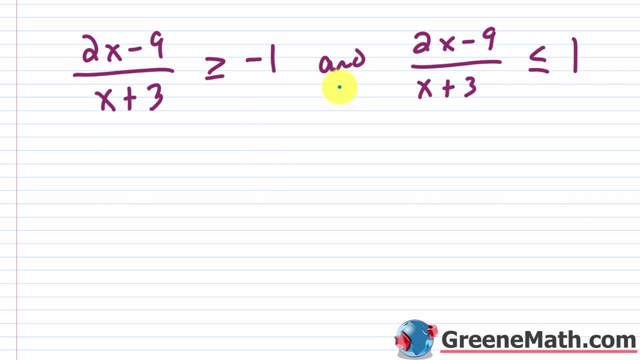 Alright, so we're just going to solve each part separately And then we'll join our two solutions with and. So for this one I would add one to both sides of the inequality you're going to get 2x minus 9 over x plus 3.. 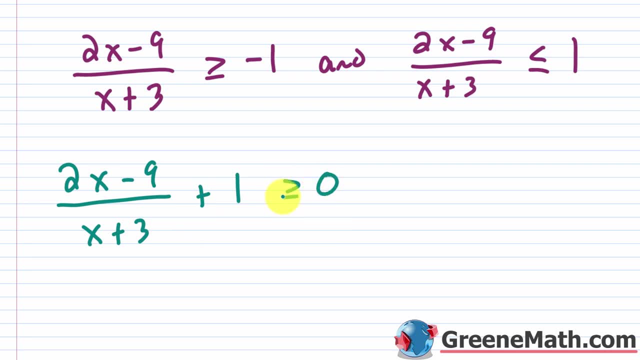 And then I'll go plus one here, and that's greater than or equal to zero. Now let me slide this down. This is pretty easy. If you just have a one, well then I can multiply this by x plus 3 over x plus 3.. 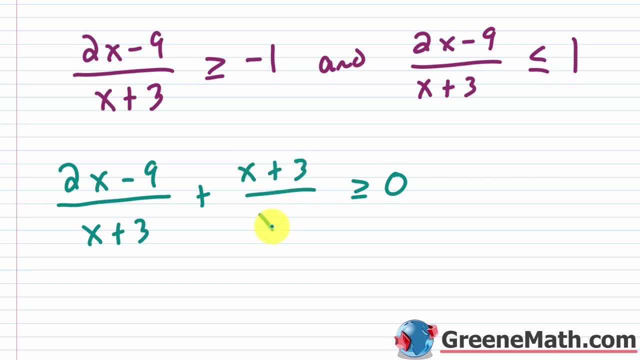 So that I have a common denominator. That's pretty straightforward. And then basically, 2x plus x would be 3x. So this is 3x, And then negative 9 plus 3 is going to be negative 6.. And this is over your common denominator of x plus 3.. 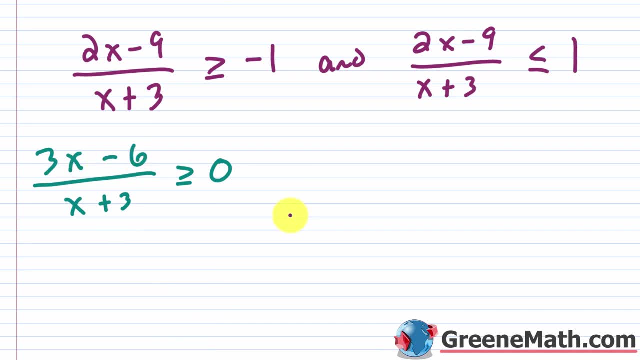 And let's think about our critical values now. So you'd set the numerator equal to zero. So you'd say 3x minus 6 is equal to zero. Add 6 to both sides of the equation. This cancels. We get 3x is equal to 6.. 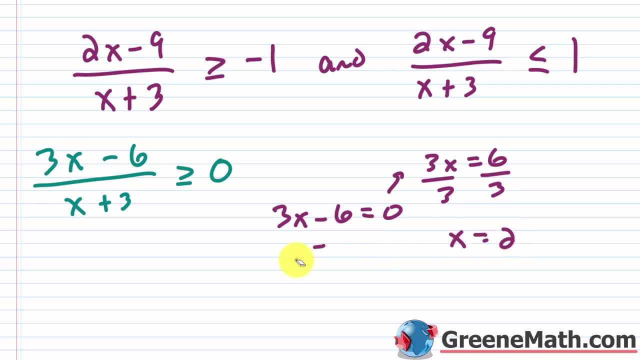 Divide both sides by 3. You get x is equal to 2.. All right, So that's one critical value. We'll say x is equal to 2. And I would note here, because this is non-strict, that 2 is going to work. 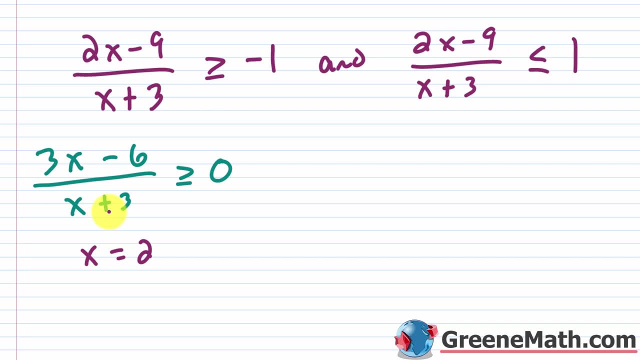 The other guy. you'd set x plus 3 equal to zero. You'd solve that. You get x is equal to negative 3.. We know that this is not going to work because this would result in division by zero, So let's go to the number line now. 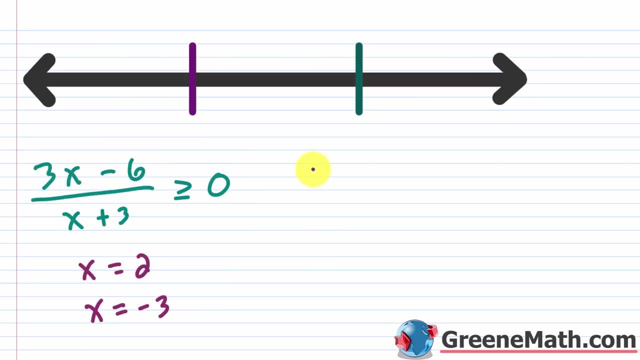 And we're just going to test Now. you could factor this to make it a little bit easier. So if you pull out a 3, you'd have x minus 2 inside Again. it's not necessary, But just something I like to do. 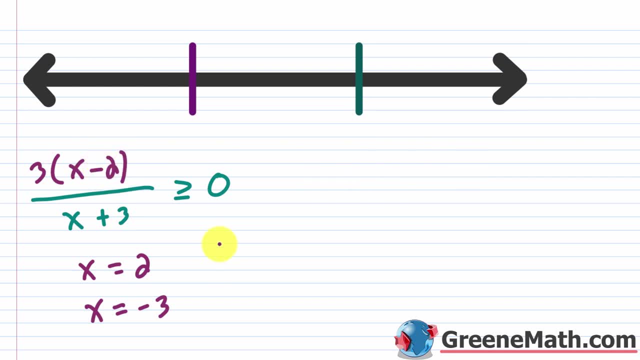 So 3 times the quantity x minus 2.. And then essentially you have the critical value here of negative 3 and then 1 of 2.. And then let's go ahead and set up this and say this is a, so anything less than negative. 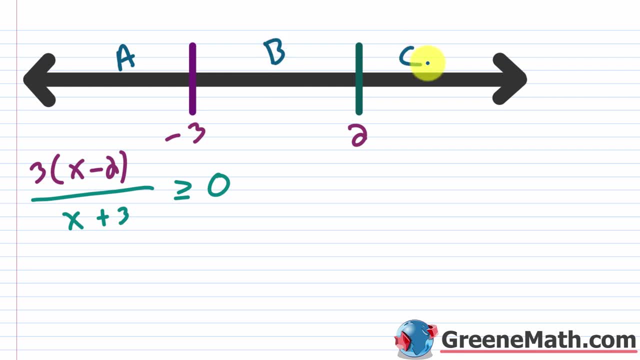 3.. This is b- between negative 3 and 2.. And this is c- anything greater than 2.. So, thinking about this, I'm going to start in a and I'll just pick something like maybe negative 4.. I think that'll be easy to work with. 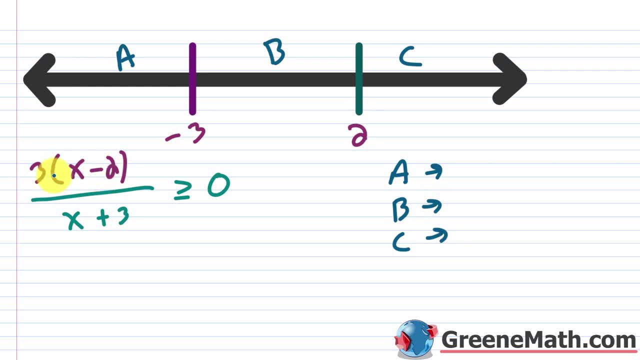 So negative 4 minus 2 is going to be negative 6. And then negative 6 times 3 is negative 18.. This is over. If you have negative 4 plus 3, that's going to be negative 1.. 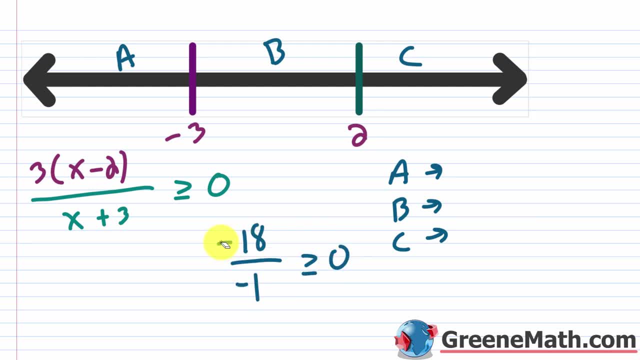 Now we know that a negative over a negative is a positive, So this is basically a positive 18 here, And of course, a positive is always greater than 0, or you can say 18 is greater than 0. So this is going to be true. 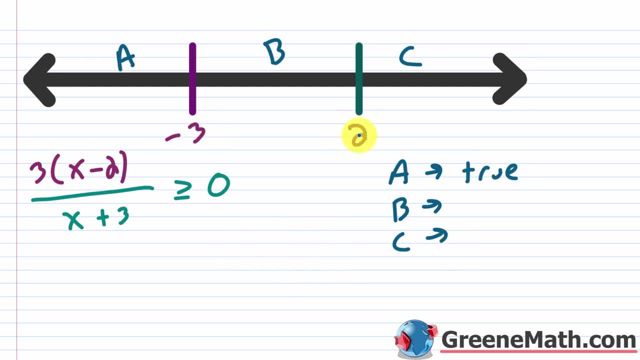 Okay, For the next one, you're going to be between negative 3 and 2, so you could pick 0.. So 0 minus 2 is negative 2.. And negative 2 times 3 is negative 6.. And this is over. 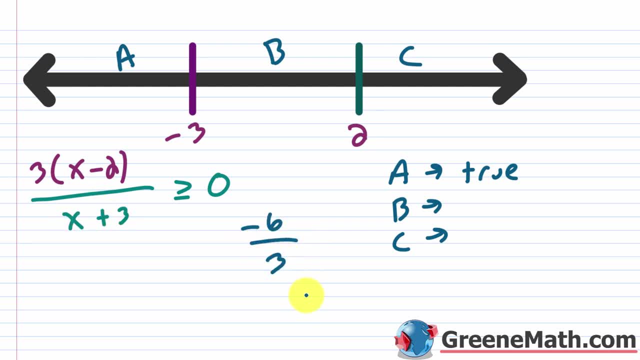 Here, this would go away. You just have 3.. 6 over 3 is negative 2.. So this is negative. 2 is greater than or equal to 0, which is going to be false, right. So you could say that any negative is never going to be greater than 0 or equal to 0.. 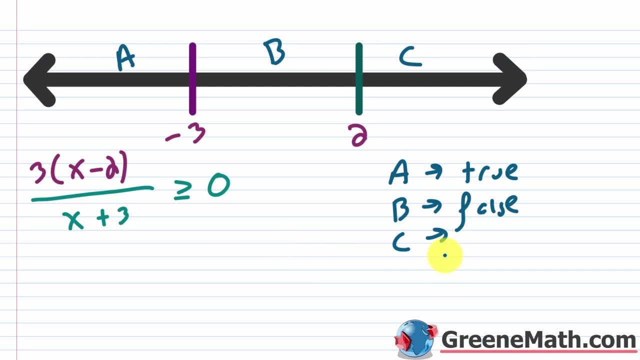 So that's why that's not going to be true. Okay, For c you could pick 3.. It's anything greater than 2.. So 3 minus 2 would be 1.. 1 times 3 is 3.. 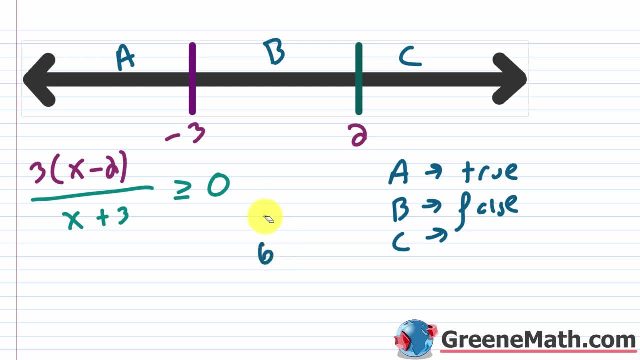 And this is over. If you have 3 plus 3, that's 6.. So 3 over 6 is going to be a half, But more importantly, it is a positive value, so it's greater than 0. So this is going to be true. 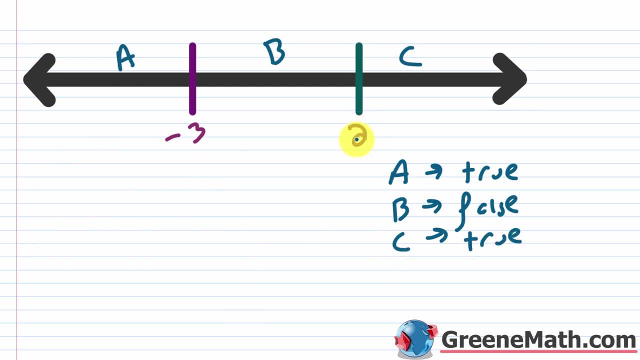 Okay, We're going to get rid of this, And I want you to recall that 2 is part of the solution, but negative 3 is not. So we're going to say that in region a, things are going to work, but negative 3 is not included. 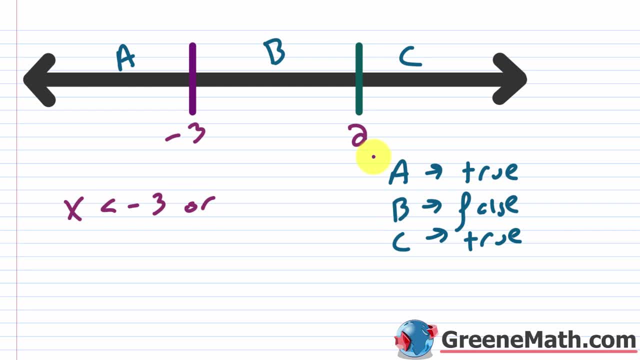 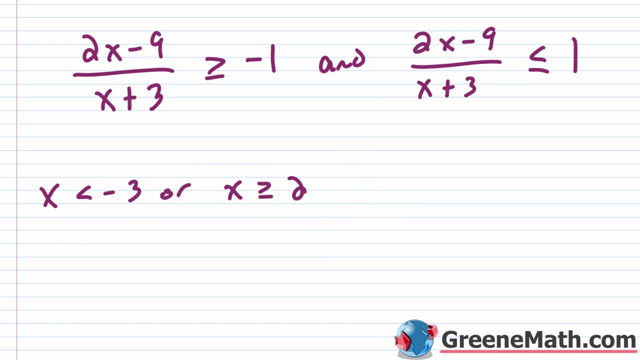 So x is strictly less than negative, 3 than or In region c things are going to work and 2 is included, So x is greater than or equal to 2.. Okay, So let's put this in right here, And then I'm going to write my keyword and: 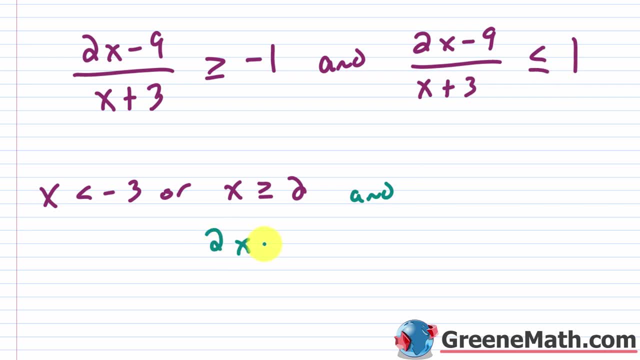 And we're going to think about the solution for this guy right here. So let me write this: So we have 2x minus 9 over x plus 3.. Okay, I'm going to subtract 1 away from each side, So minus. 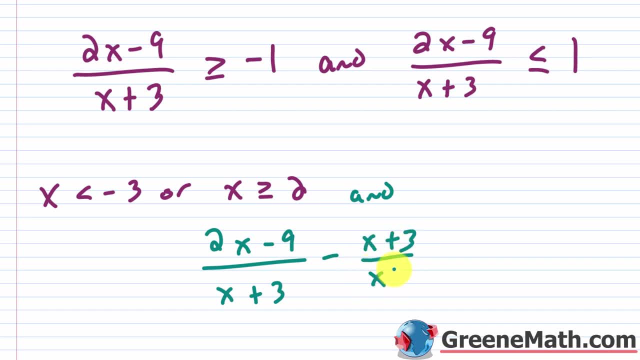 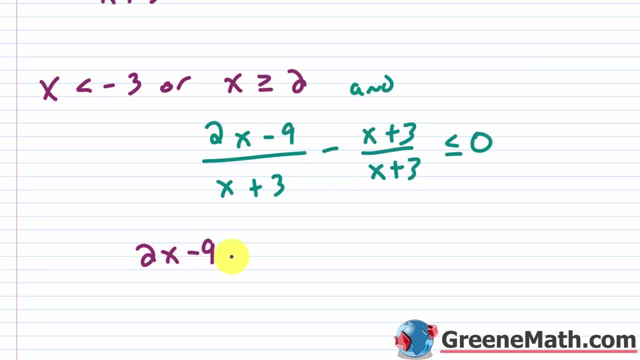 And I'm going to write 1 as x plus 3 over x plus 3.. So I have a common denominator And this is less than or equal to 0. What you want to do here is write 2x minus 9, then minus this quantity here. 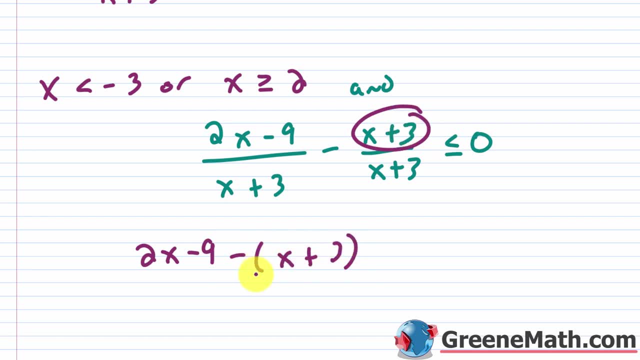 Okay, You subtract the whole thing away, So the quantity x plus 3.. And this is over your x plus 3.. Let me make this 3 better, And then we'll say this is less than or equal to 0.. Okay. 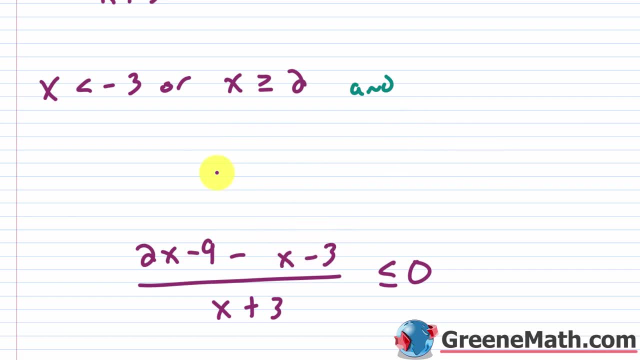 I'm going to get rid of this, And so this would be negative x And then minus 3.. So 2x minus x is x, And then negative 9 minus 3 is going to be negative 12. And this is over your x plus 3.. 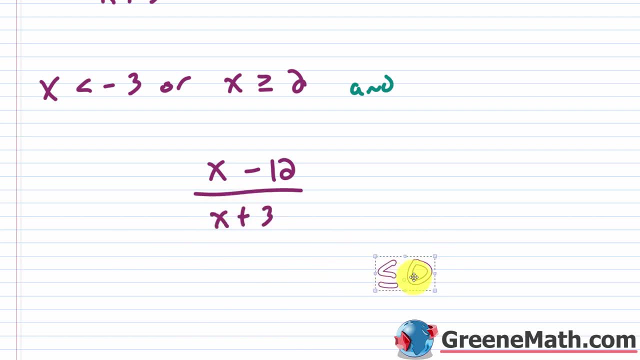 So your x plus 3.. And of course, this is less than or equal to 0.. Now for the critical values. if you put x minus 12 equal to 0 and you solve that, you get x equals 12.. And we already know this one. 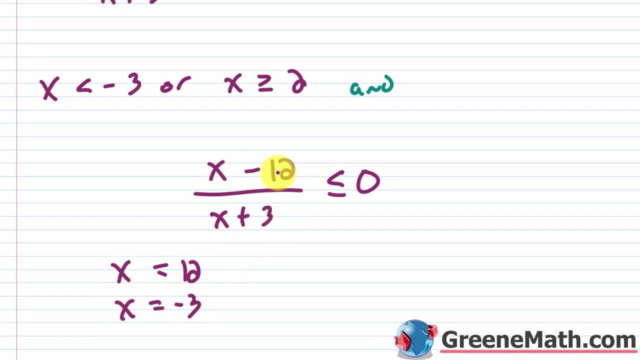 This is x is equal to negative 3.. Now 12 is going to work, because this is a non-strict inequality, But negative 3 is still not going to work, because that's division by 0.. So, coming back down here, let's put this as negative 3.. 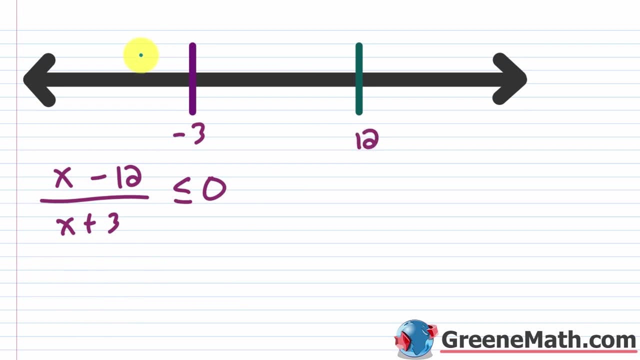 Let's put this as 12.. Let's get rid of this And let's say: this is a, b and c. So a, b and c. So let's see what we have here. All right For a, let's maybe pick negative 4.. 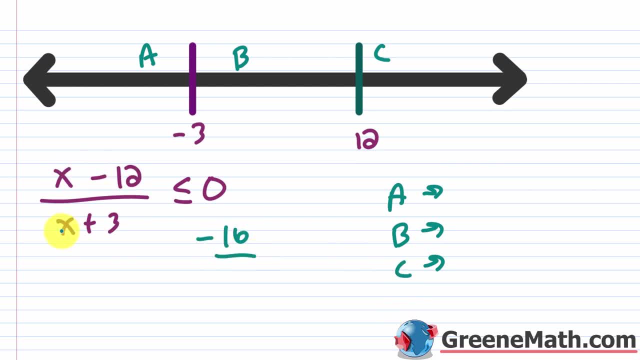 So negative 4 minus 12 is negative 16.. This is over negative 4 plus 3. That's going to be negative 1.. So is this less than or equal to 0?? Well, this is going to be a positive 16.. 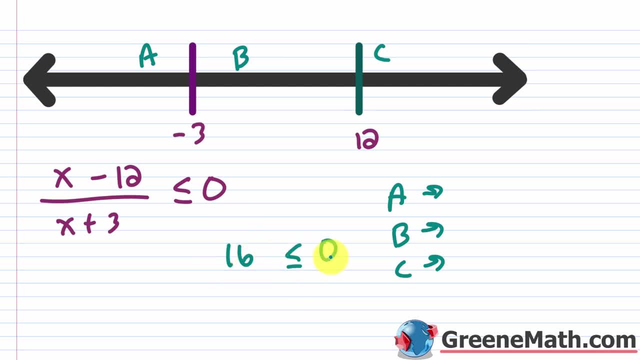 So basically a positive number is never less than 0 or equal to 0. So this is going to be false. Then for b you could pick 0. So this is negative. 12 over 0 plus 3 is 3.. 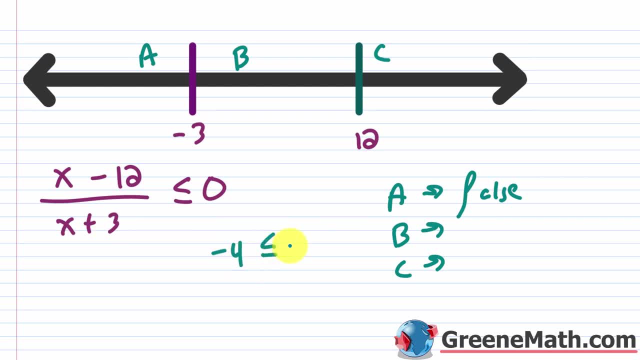 So if you do the division here, you're going to get negative 4.. So negative 4, is that less than or equal to 0?? Yes, Any negative is less than 0. So this is true. OK, For c, let's pick 13.. 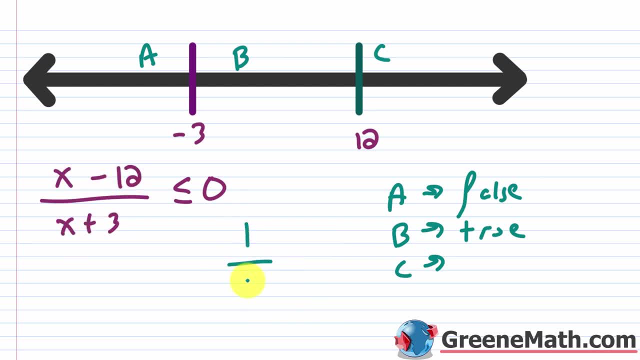 So 13 minus 12 is going to be 1. And this is over. 13 plus 3 is 16.. So this is going to be a positive value And that's not going to be less than 0 or equal to 0.. 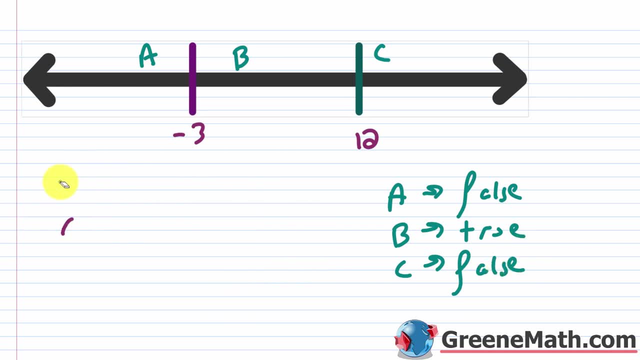 So this is false. OK, Let me get rid of this. I want you to recall that 12 is going to work and negative 3 is not, So we want things in b. So basically, x is strictly greater than negative 3 and less than or equal to 12.. 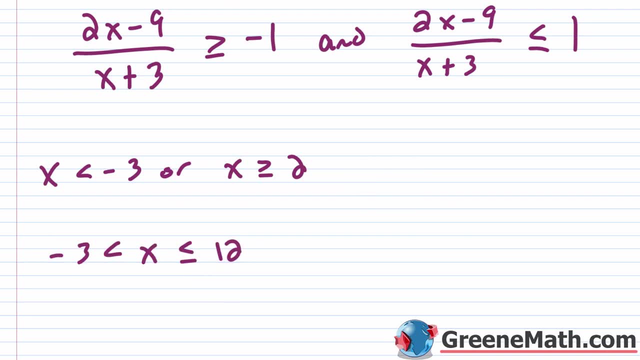 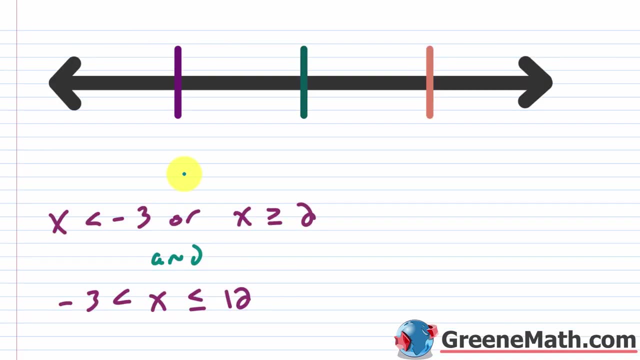 So let's grab this, Let's bring this back here, Let me move this word and down here. So basically, we're going to think about this with a number line, So we're going to have three values that I'm going to put up here. 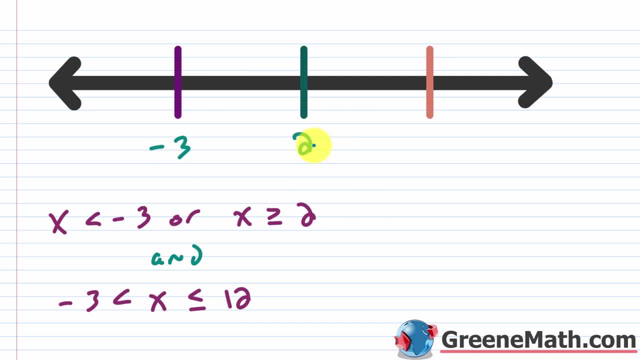 So one is negative 3. The other is 2. And the last one is 12.. OK, So let me think about this one first. So you have x's Less than negative 3. So let me just draw that out. 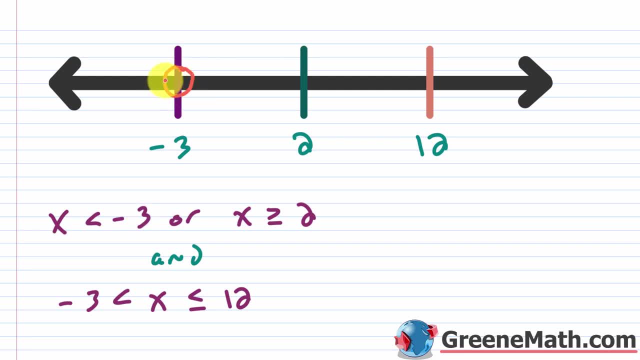 I'm going to use an open circle here. I don't typically do that, But for this purpose I think it's probably better. Then you have: x is greater than or equal to 2. So let me put a filled in circle there, because that's included. 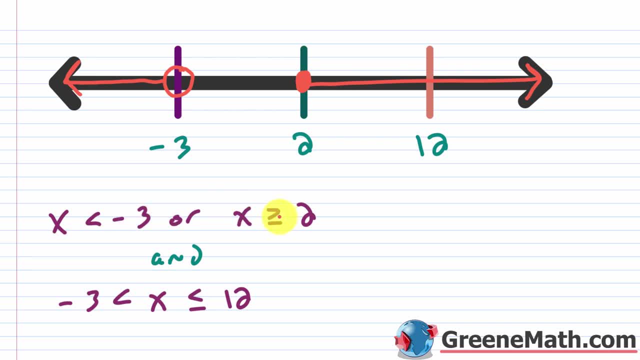 And then let me shade everything to the right. OK, So that's this one right here. Now let's think about this one right here. So here we're saying that x is greater than negative 3.. So greater than negative 3.. 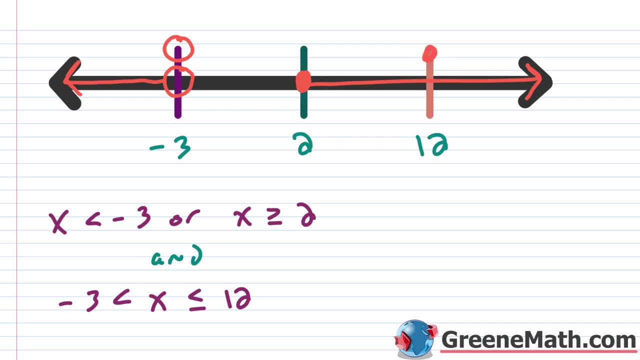 And less than or equal to 12.. So let me put this in right there, And I need a different color. Let me get rid of that And make this a little bit better there, And then I'm just going to shade everything in between there. 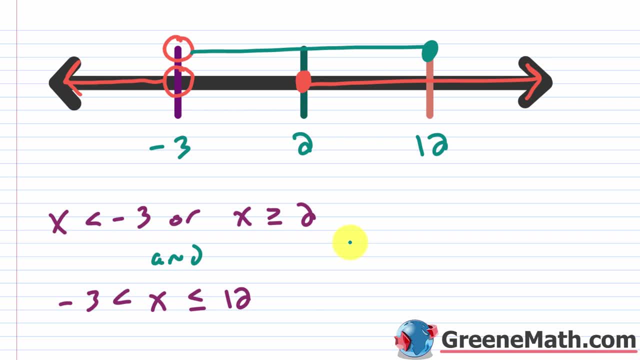 OK, So you want to think about the overlap here And essentially, looking to the left of 2, there is no overlap. You have this guy up here which is between negative 3 and 2, which is not a solution in the other one. 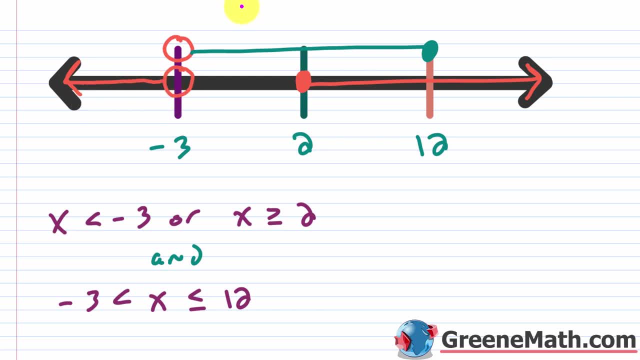 And the other one is anything to the left of negative 3.. So this part of the graph you can forget about. There's no overlap between the two. And then past 12, there's no overlap. So basically, you're looking between 2 and 12, with 2 and 12 being included. 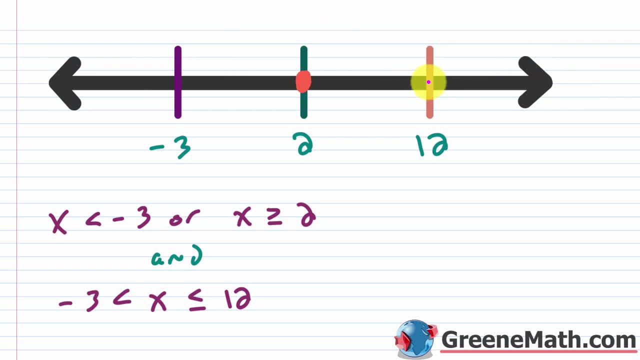 So that is what I want. if I'm thinking about my solution, Let me maybe use a different color, because that's not showing up so well. So you want between 2 and 12, right? That's going to be your overlap between the two solutions. 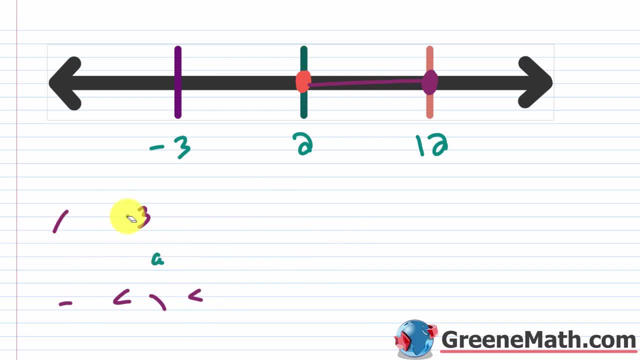 That's what you have to do when you have the keyword AND. So what we're going to say: just erase this, you don't need it. that x is greater than or equal to 2 and less than or equal to 12.. 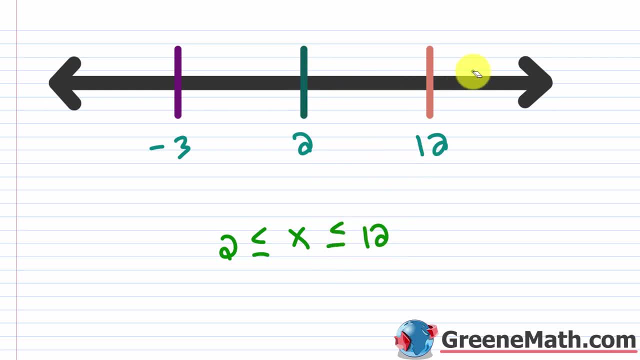 So both of these are going to be included, And let me use a bracket here. I'm just going to change the color up completely, So let me use this color. I'm going to use a bracket at 2, or you can keep the filled in circle and a bracket at. 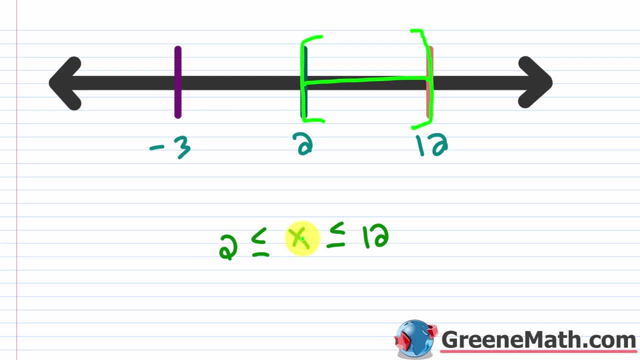 12.. And I'm going to shade everything in between. So x can be any number, including 2 and going up to and including 12.. In interval notation it looks like this. So you have a 2 here with a bracket and then a 12 here with a bracket.